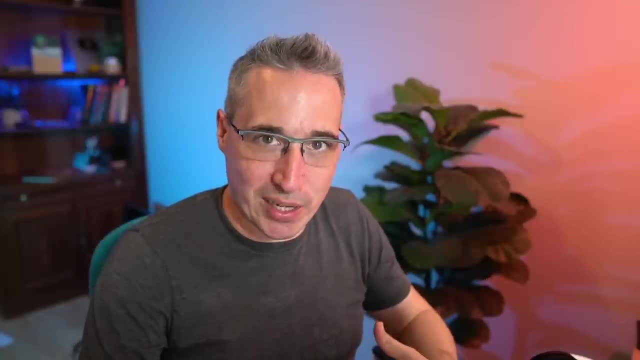 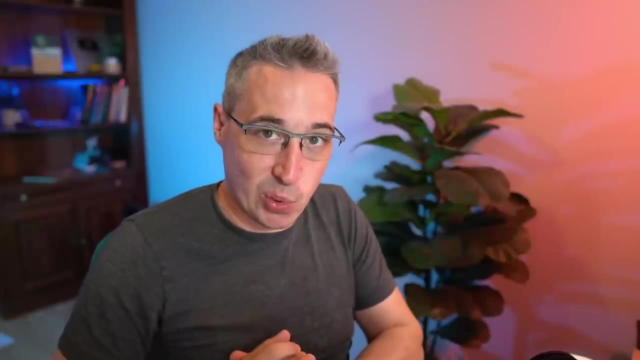 mostly going to be about, but maybe a little bit more than that as well. So, as I said, it is the beginning of a series. There will be multiple videos in this, each one coming out a few days after the previous one, and we're really going to go into this one in how I would approach starting. 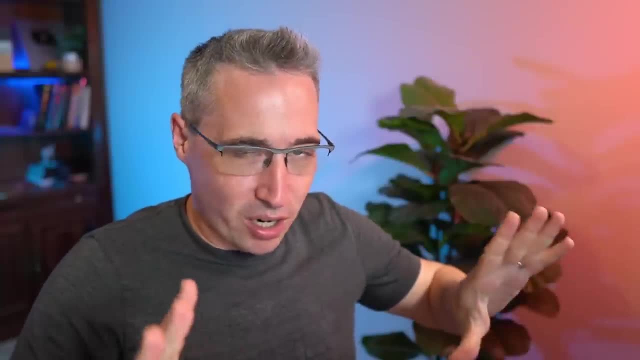 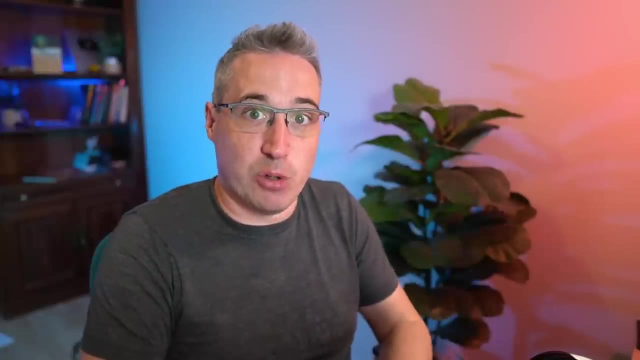 a new project. The designers have just given me this file. I haven't done any work on it yet. We're going to be diving in, analyzing the layout, looking at the different things that might be a challenge and building it how I would build this as an actual 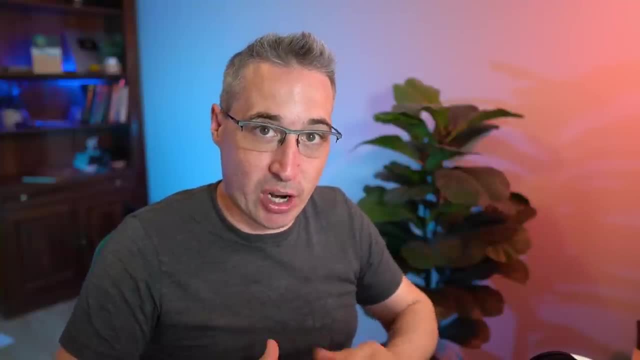 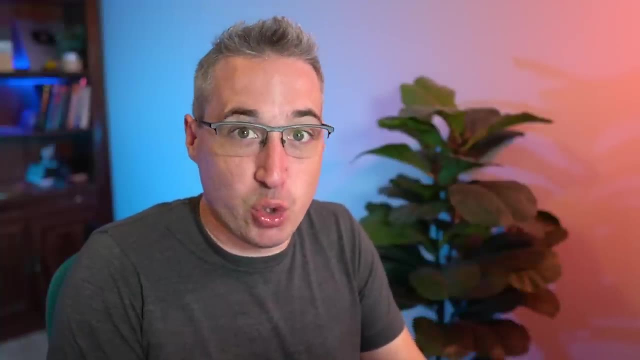 project Now. that said, I do want to keep this fairly beginner friendly, so I'm not going to be going into the world of SAS or doing other things like that. We will be using VEET just to sort of get things up and running and all of that, but nothing too complicated there You're going to 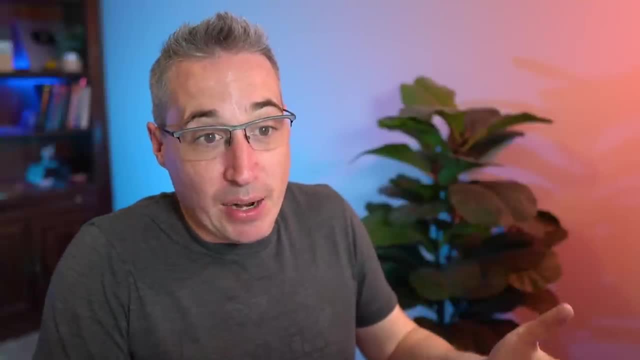 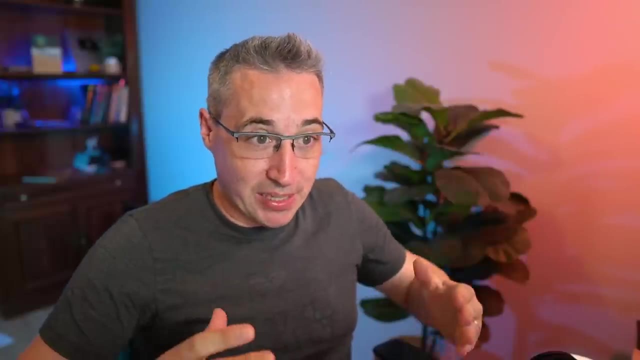 see, it's very, very easy to do and, yeah, I want to make it so we can sort of explain my thought process as much as possible. This will be the first time that I'm actually building this project out, because I want to show you really how I would do it from scratch, including the problems I might run. 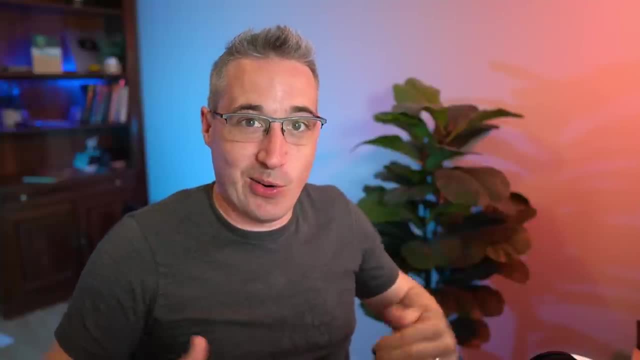 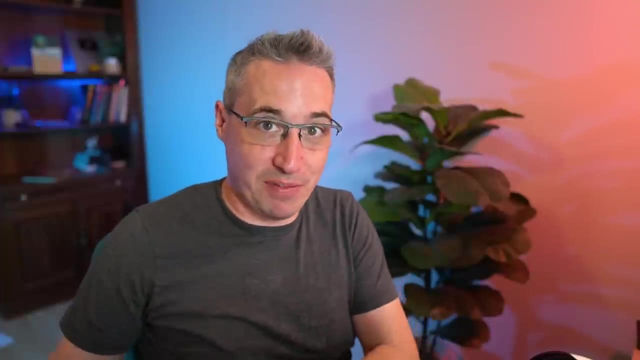 into and how I solve those problems. Now these videos will be edited. so if I do run into a problem that takes a long time to fix, I won't show you 45 minutes of me banging my head against the wall, but I will show you how I eventually found the solution to it. but I don't. I don't know what. 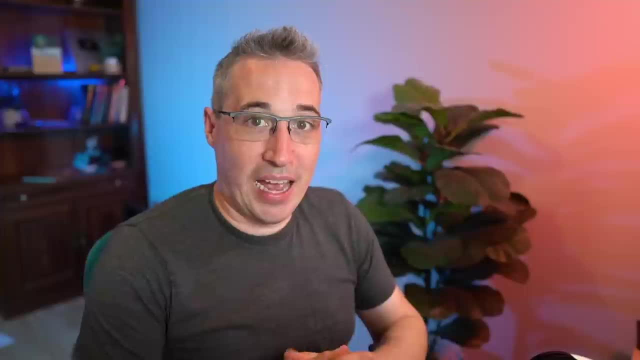 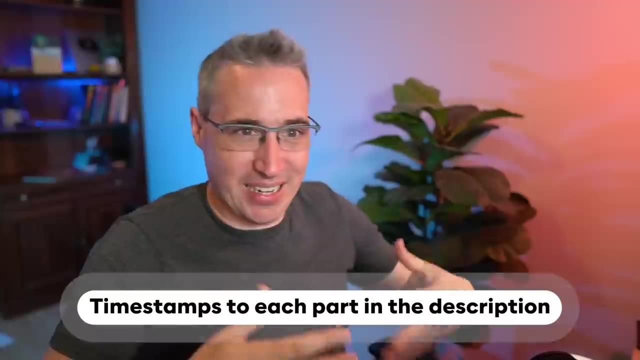 we're going to run into or anything, because, as I said, I haven't done any of this yet and, as part one of this series, what we're going to do is analyze the files that we're actually going to be starting with and what we're we're looking at, break it down a little bit, see if there's. 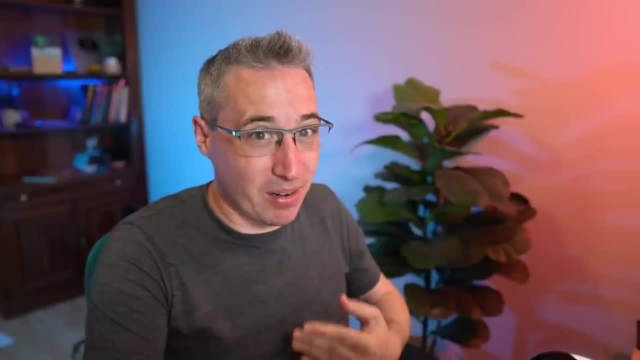 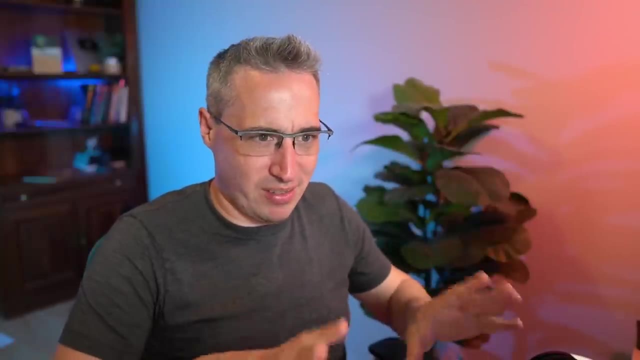 anything that might be a problem Or things that we might have to think about a little bit deeper and just get an idea of what we're actually trying to do, a big picture idea, and then we'll set up like the basic project structure and starting thing that we're going to use and build off of from there and that will 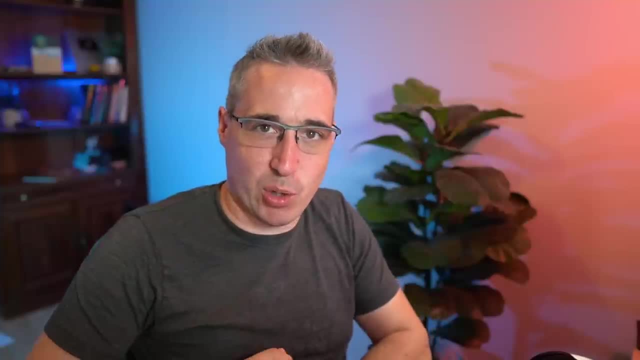 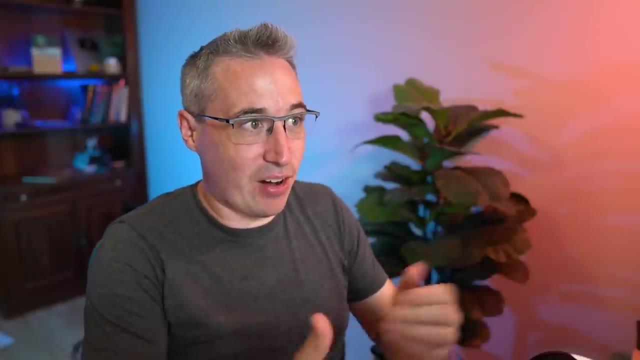 lead us into the following parts. We'll go into more detail on each section that we're going to be looking at as we build it out, and so, yeah, the first thing, let's dive in right now. for the beginning of this- and you can see, here I have Figma open, so if you do have a free friend and 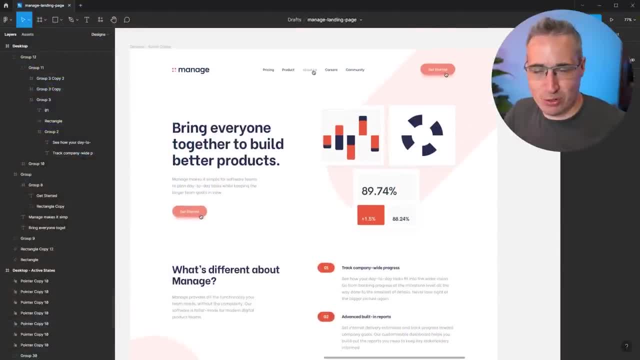 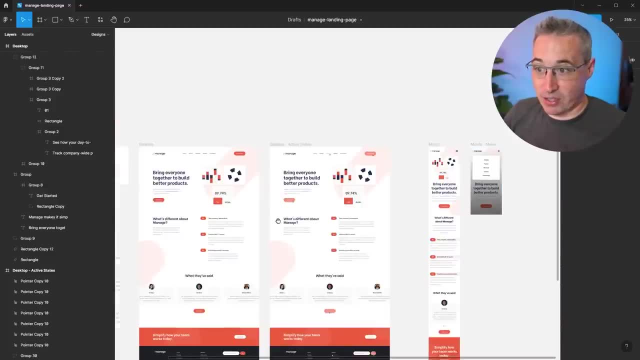 mentor account. you can't get the Figma file, but don't worry about that Too much. there's not too much extra. you get in a project like this one anyway, and let's look at what what they've given us as our files. to start with, where I have my colors, I have my desktop, the 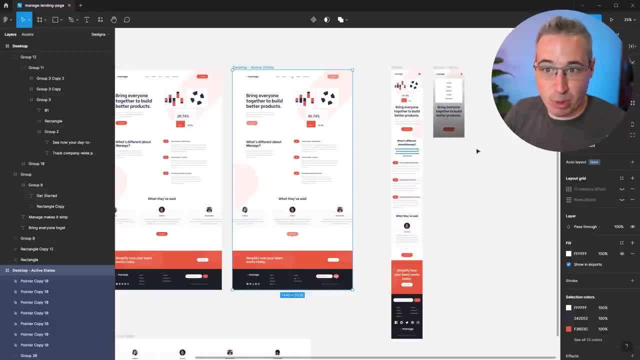 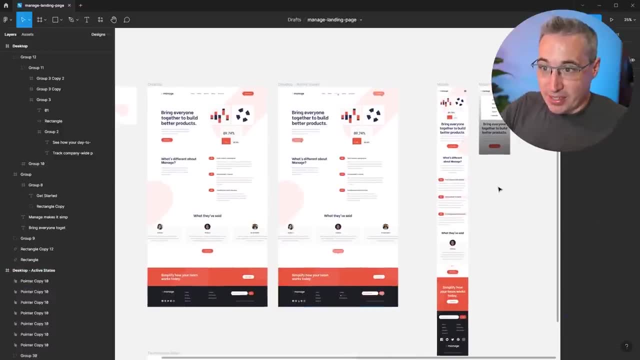 active states for the buttons. so when we're hovering on top what they look like, and then the mobile view here, as well as the mobile menu that we're going to have to build out, and, yeah, when I have a project like this, the first thing I really generally like to do is 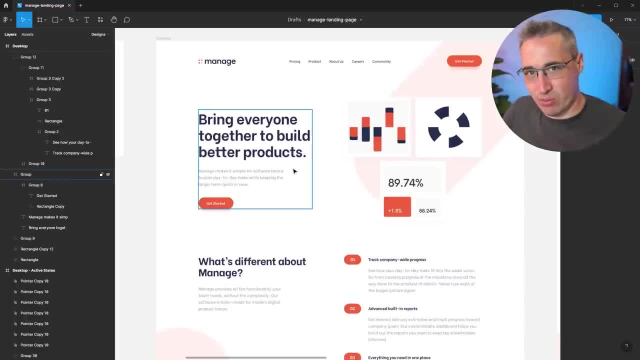 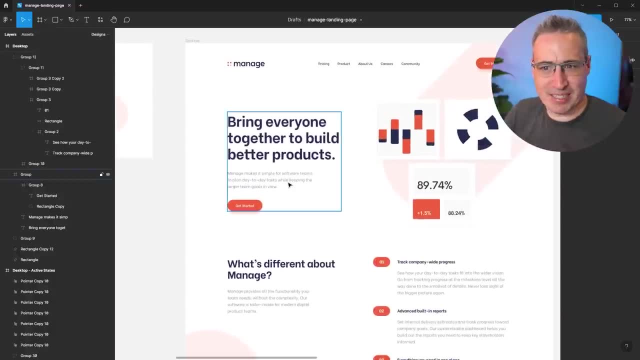 just look at it really quickly and sort of analyze a few different things. so, right off the bat, one of what is nice is the consistent colors throughout. there's not very many colors, we just have a handful of them, which always makes life a little bit easier on that set of things. the typography: 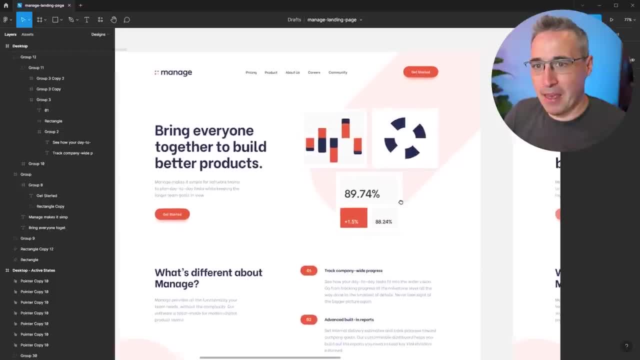 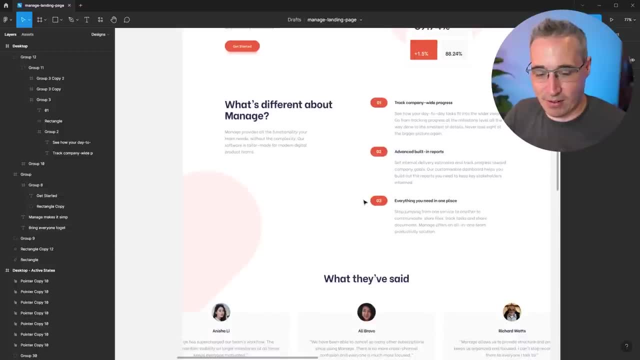 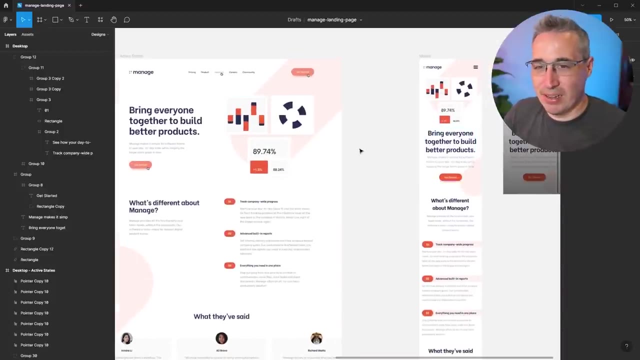 looks very straightforward. I don't see any problems arising from that. the navigation looks fairly straightforward. now this SVG. I'm guessing there and here. I like looking at how that's going to work across. so you know what. what happens to those when we get to mobile. so a few little differences. 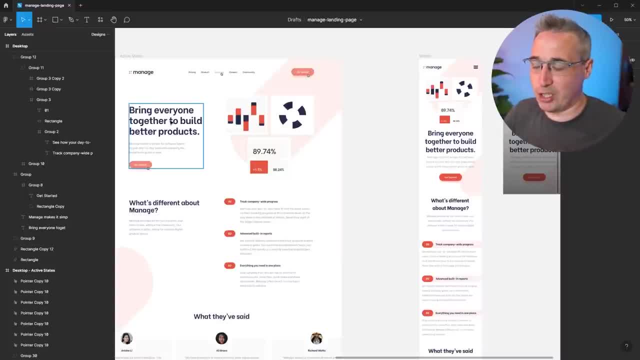 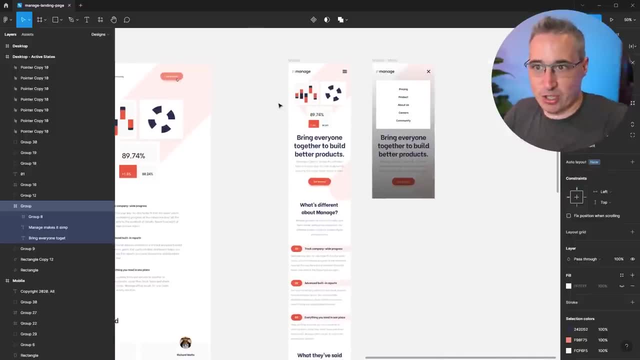 happening also just here, something I think it's a little bit more unusual. actually, usually I find whatever's on the left ends up on the top once we move over to mobile, but here, in the mobile view, the image is actually shifting up. it's like all of this goes up into that space and then this comes after it. so it's a little bit more. 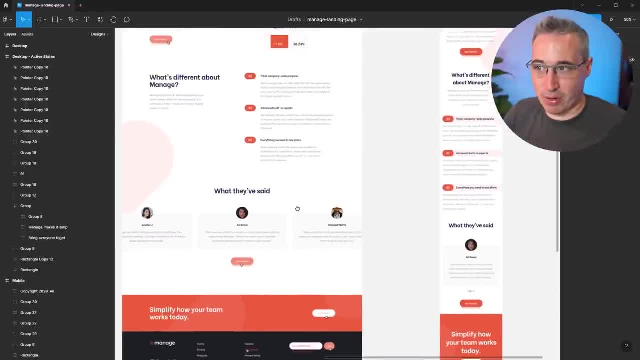 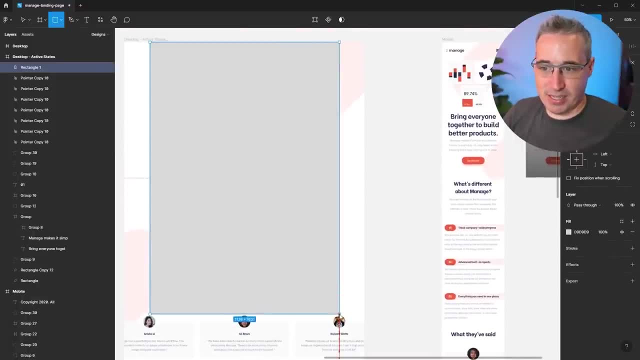 unusual. um, we don't have too much when it comes to like shifting background colors or anything- though we do have a few things here- but it looks like we do have a consistent container type thing, like all of this is all the same width until we get to this carousel down here and then that same. 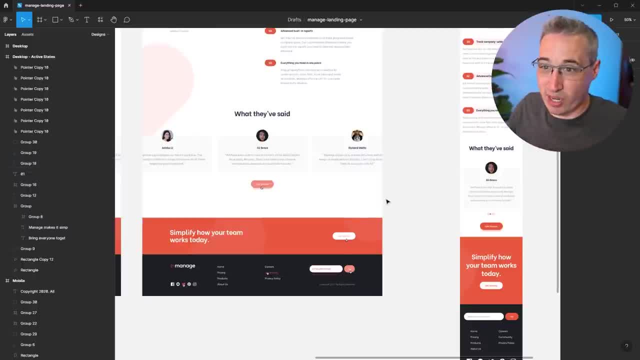 container carries through to all the stuff down here, so we don't have, like, different widths showing up on stuff which is always nice and handy- uh, because that makes things just a little bit harder to do. um, the biggest challenge, honestly, is probably going to be this carousel right here. 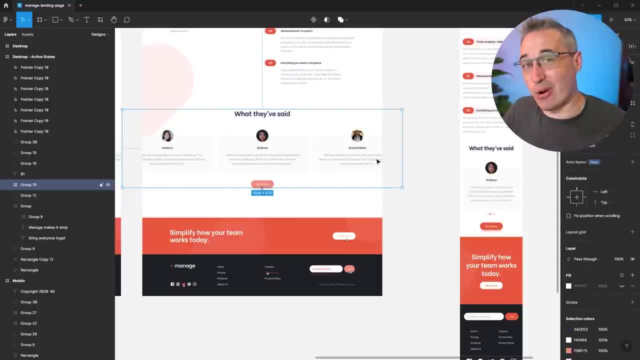 because we have it here where there's no real indication. I don't see any arrows or anything like that. I think we might deviate a little bit from the design just so we actually have arrows to click on, because as it is now, unless I guess it's auto going, but I'm not a fan of those. so 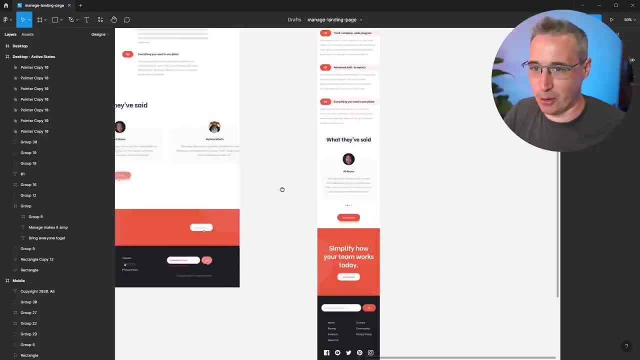 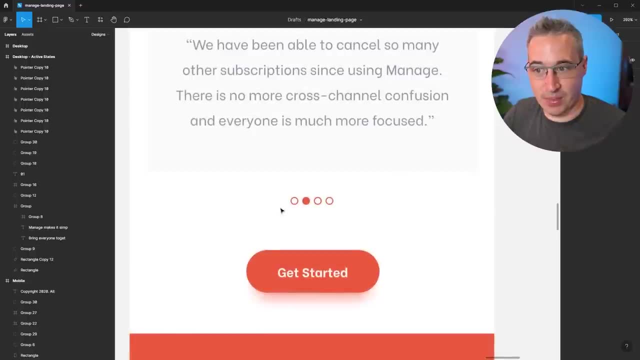 uh, anyway, we'll see what happens when we get there. I'm going to plan some things out, but we can see that things look quite a lot different when we're in the mobile view, where we get the the little icons down here at the bottom to show us which. 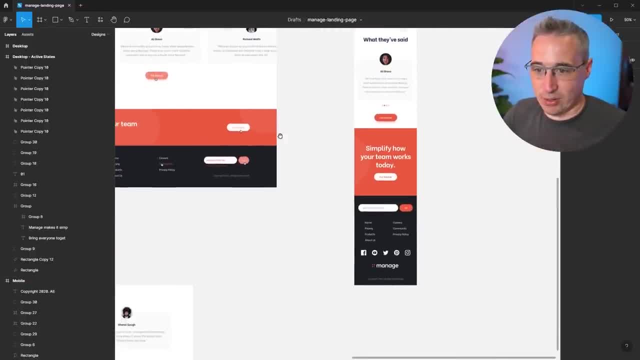 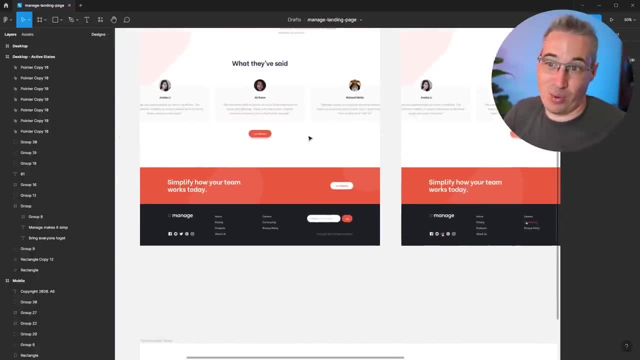 slide we're on. so a few things that we need to take into account, but nothing too complex. oh, here's the full slider. I didn't even see that before. so here's all. like we have four and we fit three on the screen, or like two, and these two are hiding a little bit, I guess, just to show us. 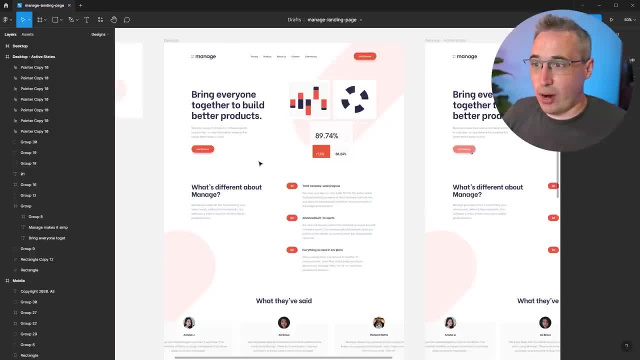 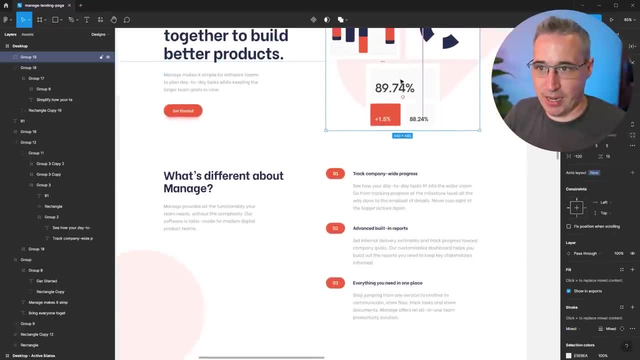 that there is more uh, that's there. so, uh, overall it doesn't look too complicated. but before I like diving into the projects, I do want to like look at a few more things on here. like here we have a two column layout and actually this looks pretty consistent when we come down to 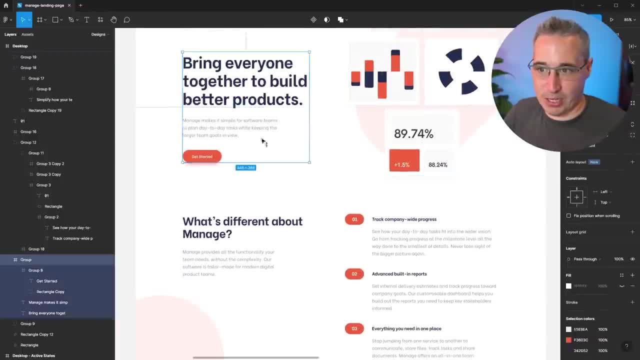 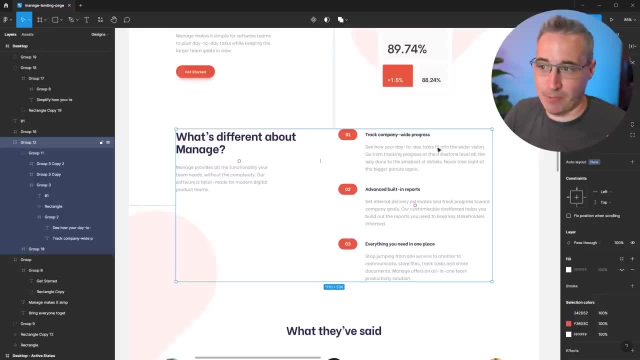 this section. so this two column and this two column, including, like, the gaps that are around these things. they actually look really consistent, which is nice, because that's not always the case, but that makes life a bit easier. um, this area is what's different about like. this box here is not. 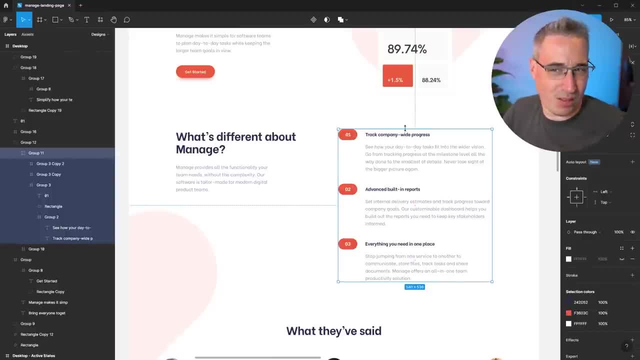 too complicated, actually, but then here we sort of have two columns, but it depends how we want to approach it, uh, and when I am looking at a layout like this, the first thing I am thinking of is, like what, what elements am I going to be using? so, like for most things, it's- you don't stress too much- like oh, 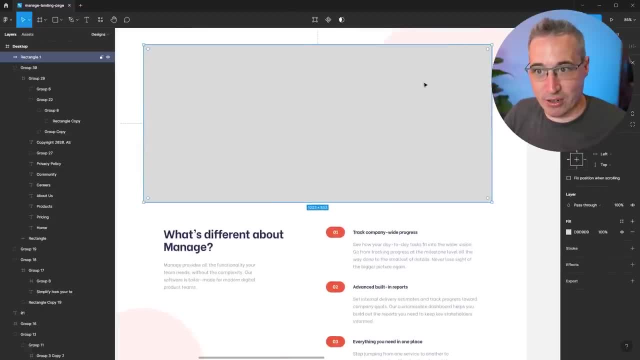 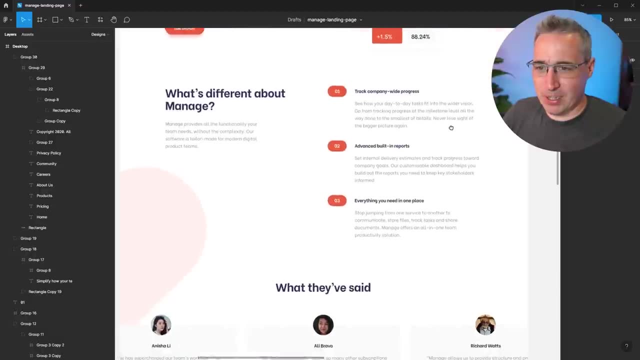 here. I see like a div coming across. this, which is my container. I'll have something in that that's going to create the two columns, things like that. um, I don't really stress too much about uh, but it's when you see things like this where we have these numbering systems and it's like well, what's? 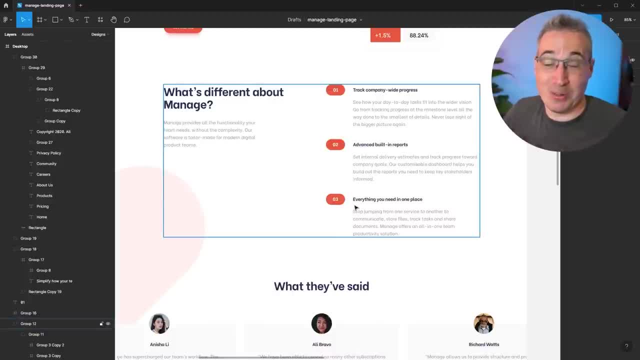 different. is it really like? are these zero one, zero two, zero three purely decorative, or are? is it more of a numbered list and so like? from a semantics point of view, which one would be better to use here? to me, the numbering here is more visual than it is like. oh, this is the number. 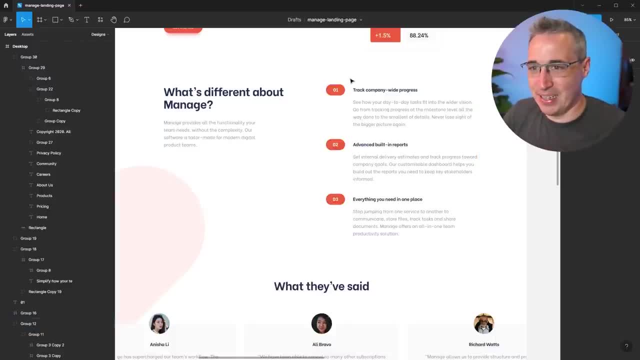 one thing, the number two thing, the number three thing- because we do have the numbers- I might do this as a numbered list- I'm still trying to decide on that and maybe we'll sort of make a decision- but definitely ul's here or ols and then depending how we'll do the numbers, and that would actually 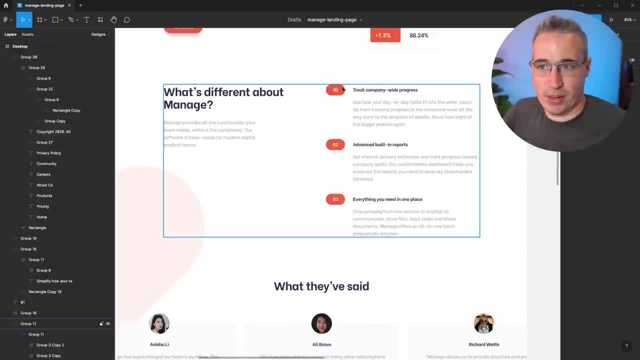 change a little bit how you'd want to do this, but I'm just going to go ahead and go ahead and do this, because if you're doing it with a list- and this is part of your list, um- or even if you're doing like a before and an after you need, this would become like padding or something like that, whereas if I 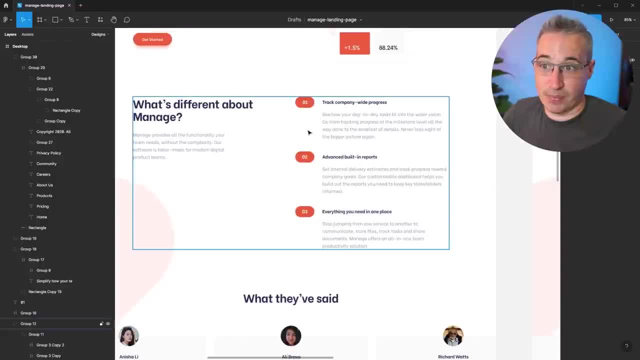 was doing this as something that is, um, you know, just a visual, where I could just throw a div in there or something like that. uh, then I could actually make this like a two column section where I have a div that's doing a left column and a right column for each of them, so some. 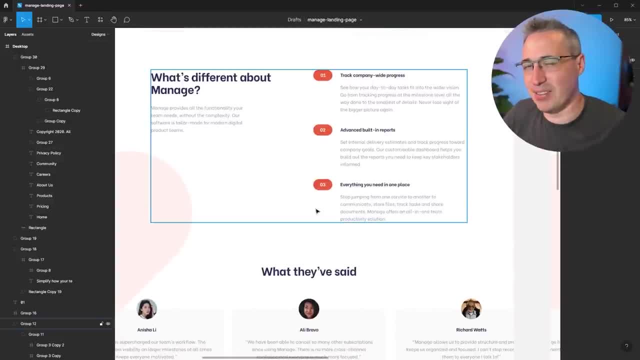 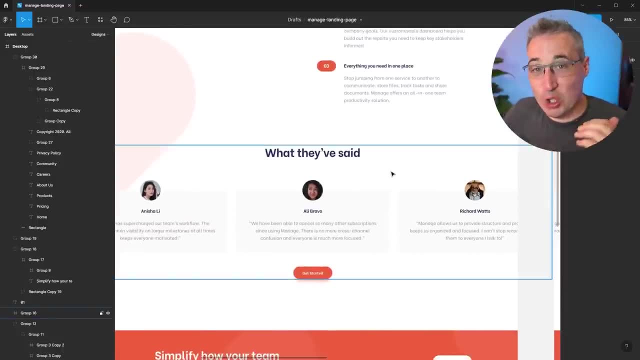 thought will be going into that, or we'll see, because if it is pseudo elements, there's a bit more. I have a few ideas there. um, we'll see. this is a carousel that I don't want to spend too much time on making a good carousel, so we're going to see if we can find um like a nice, accessible, easy slider. 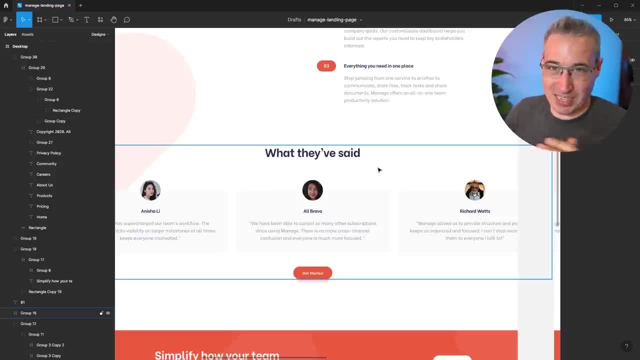 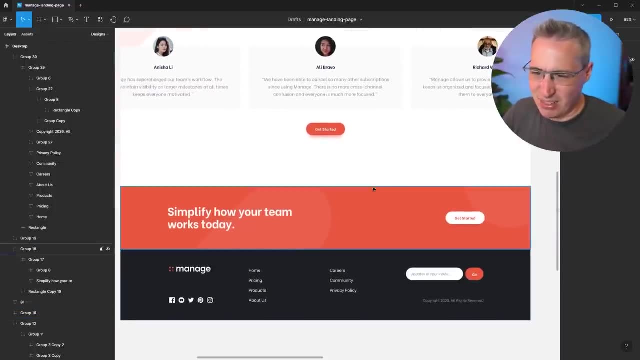 or carousel type thing, because making ones that are accessible is actually really, really hard to do. there's a lot that goes into it, so maybe we can speed that up by bringing a third party in for that and down here there doesn't look like there's anything too complicated. um, yeah, so I think. 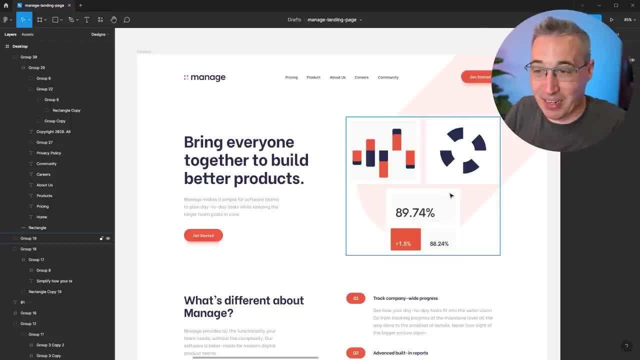 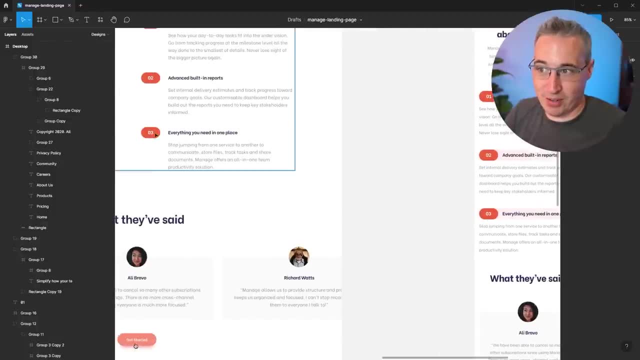 overall, it's looking pretty good. yeah, that's sort of the first step that I like to take and now that I've sort of had the time to look over things- and of course you know, looking over these, oh, there's another difference. actually, here these lists look a little different, but that's not a big deal, I'm not too stressed about. 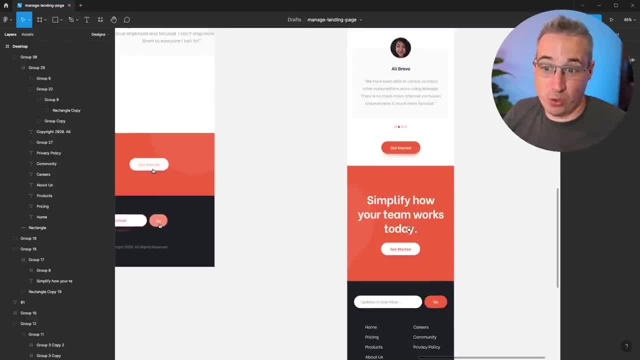 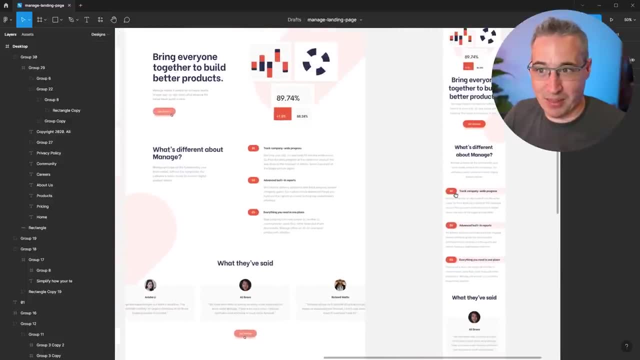 that there are some thoughts we're also going to have to make here when it comes to where's the media query going to be. do we need more than one media query? I'm guessing the font sizes shift around a little bit, and things like that as well, so we will have to, at least some of them will. 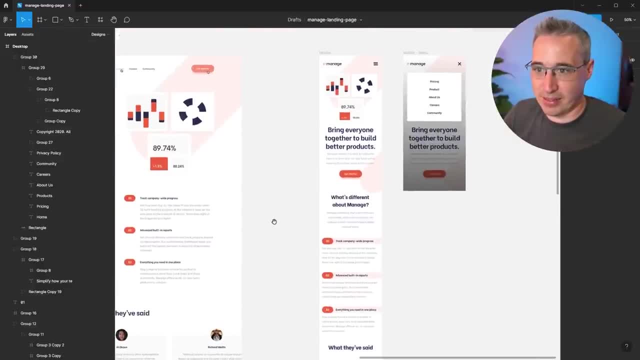 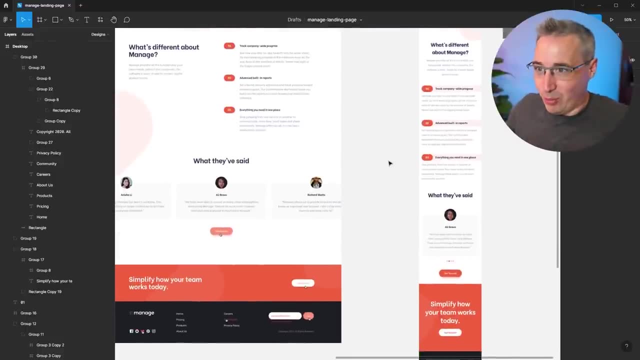 um. anyway, we'll dive in and look at that as we're styling things up a little bit more. um or not styling things up, we'll do that in the next step, when we set up everything we need, which I think we're ready to do now. I think we're ready to sort. 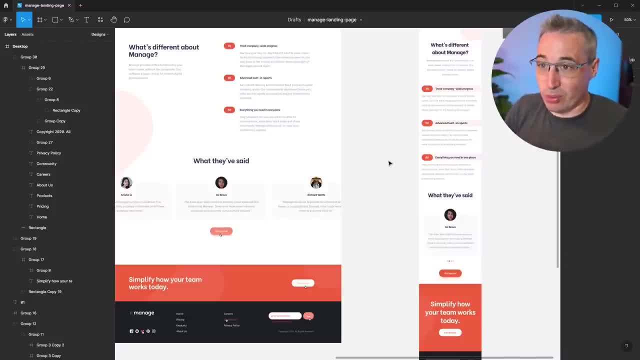 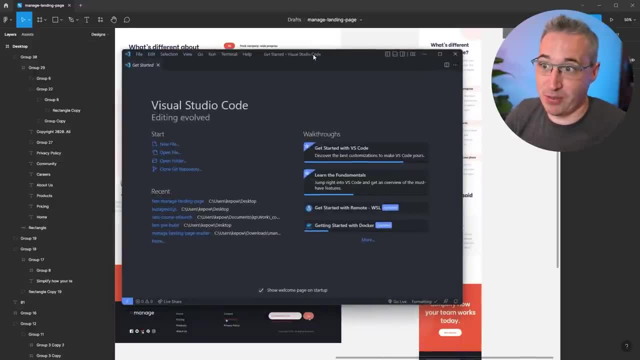 of set the base that we're going to build everything up on top of. so yeah, we'll jump into VS code and we'll start doing that, and so here's VS code. they don't even need VS code for this step. you could open this up in terminal or something else if you want, but I'm we're going to be using VS code, or I? 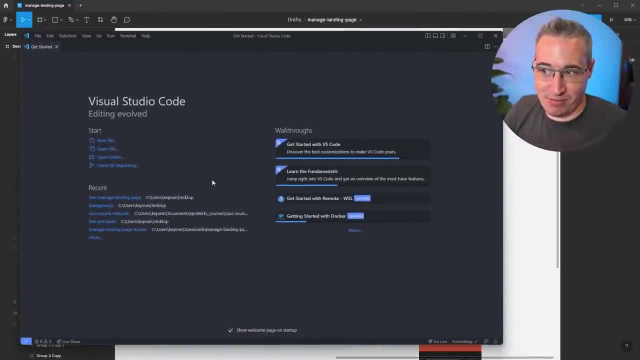 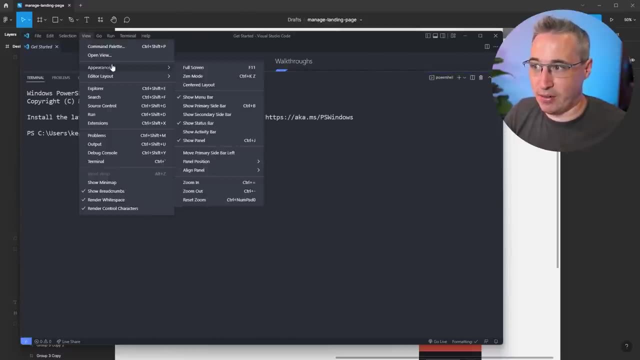 am anyway. so I'm going to open up VS code here and instead of going to a folder or doing something- and you can get that by going to view and then uh, terminal here or on my keyboard, it's control back tick, it's command back tick. but I know in Europe apparently that doesn't. it's a different shortcut. 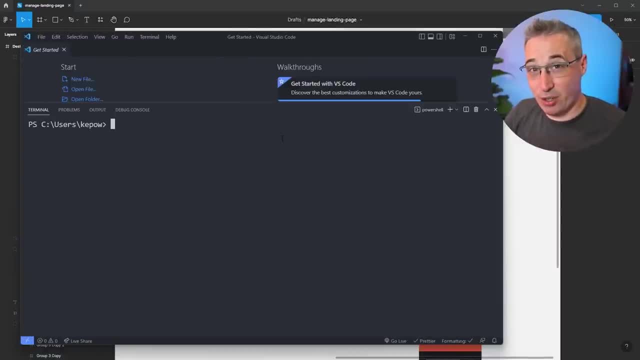 so uh, but yeah, we want to open up our terminal here, and so the first thing I'm going to do is navigate to my desktop and I'm just like in my my thing here, so my users. so I'm just going to do a CD which is a change directory- let's make this a little bit bigger- um CD. and then I'm just gonna. 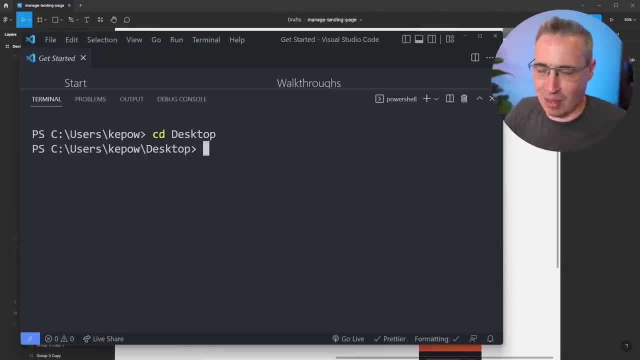 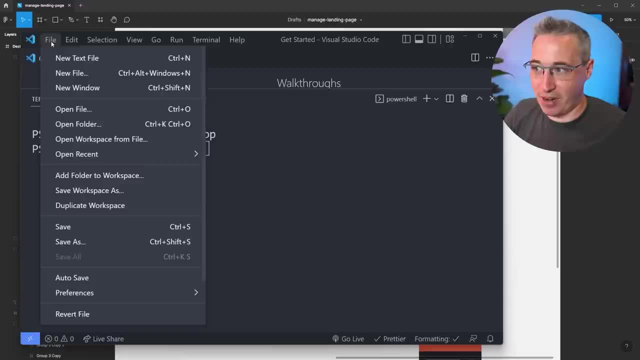 write desktop desktop and from here, and I'm doing it on my desktop, just that's where I want to work, um, you can get to there, uh. or you know, you can even just do an open file and open folder and wherever you open that folder, that's where you're going to be like, where this path will be, uh, if 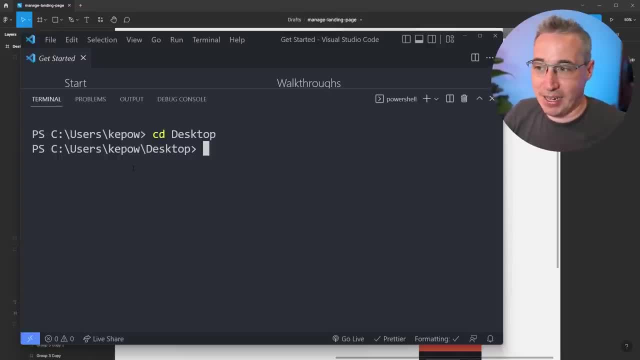 you're newer to using the terminal and all of that. and now that I'm on my desktop, I'm going to do an MPM, I'm going to write, create and it's beat at latest just like that, and it's going to ask us a couple of questions and we're really not going to use this to its full potential of what it can. 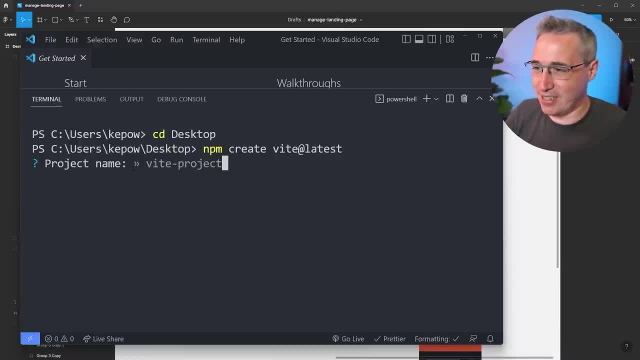 do, but it just makes our life a little bit easier and we'll probably add some post CSS in here to help us do a few extra things, which comes pre-packaged and it's easy to run in here and so here on my project name: this is the folder that it's going to create on my 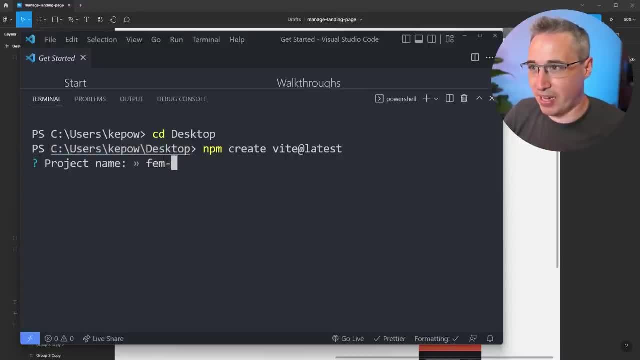 desktop, and so what we're going to do is I'm going to write FEM for front-end mentor and I think it's called manage- manage landing page. you can see it right up there in my figma file. so we're going to do that, and it's going to ask me if I want to use a framework. so if you do want to, 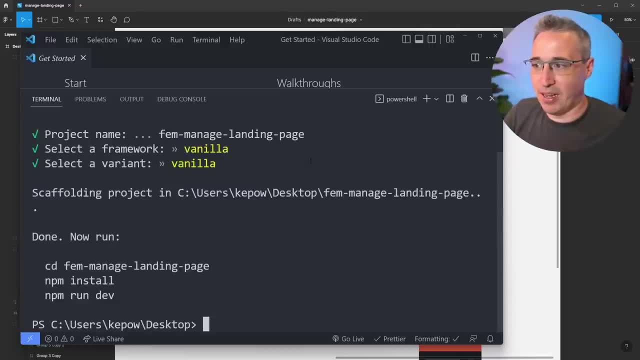 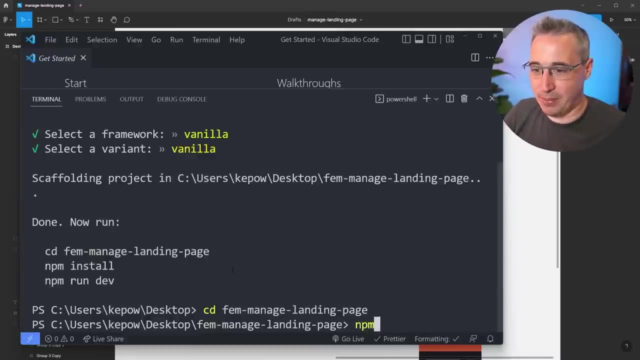 use one and you're following along by all means. but we're just going to go with vanilla and vanilla and that's fine. and then it tells me the next steps that I want to do. so CD, we'll do that. FEM, manage landing page, so we're actually in that folder and then we can do an MPM, MPM install, and I'm not going to do the. 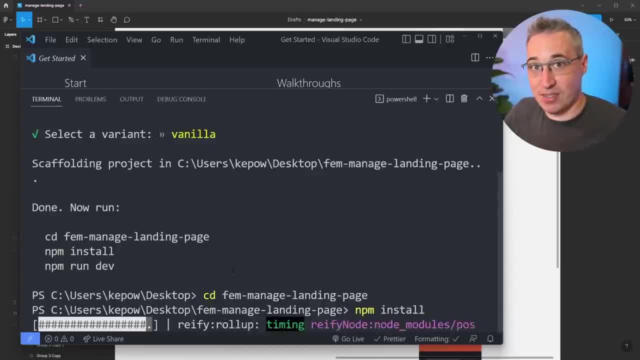 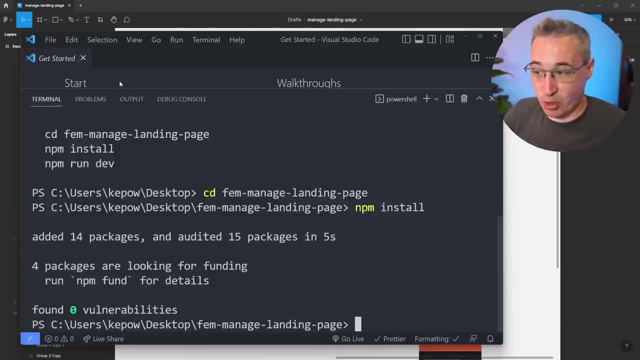 MPM run dev yet, but what the MPM install is going to do is install all the dependencies that we need to be able to run. what we're going to do here, and before I actually get started and start doing anything, while I'm here in my terminal in VS code: 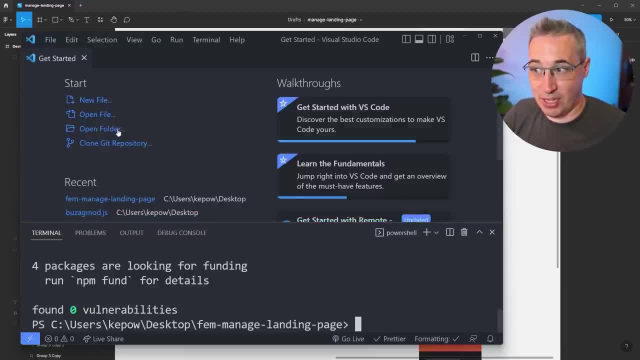 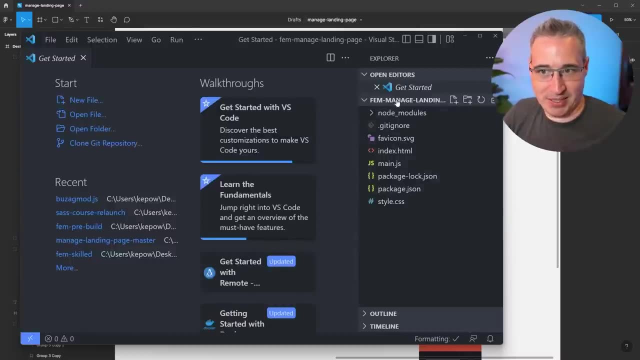 so I'm going to go to the here where it says open folder and I'm going to open that folder in VS code and there we go, it's been opened up and we can see that. I'm there because we have it. says it here: you can just see the files that are all in there and just really fast if you've never used beat before. 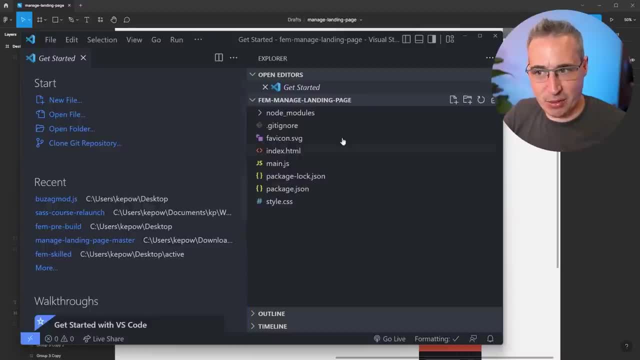 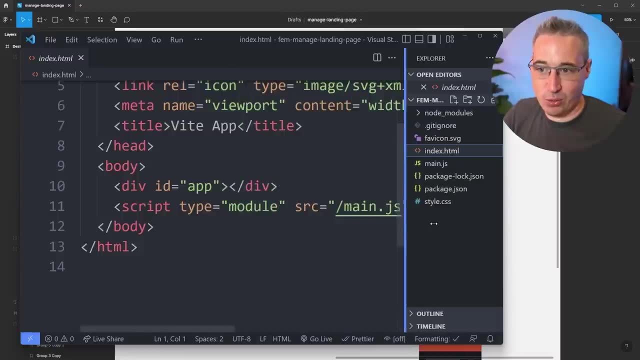 it's giving us a stylecss, some other things in here, if you're not used to them- our main JavaScript file and an index here, and it is looking to actually do like inject everything via JavaScript. so we're going to delete this. we're going to keep it a little bit simpler than that, so we're going to 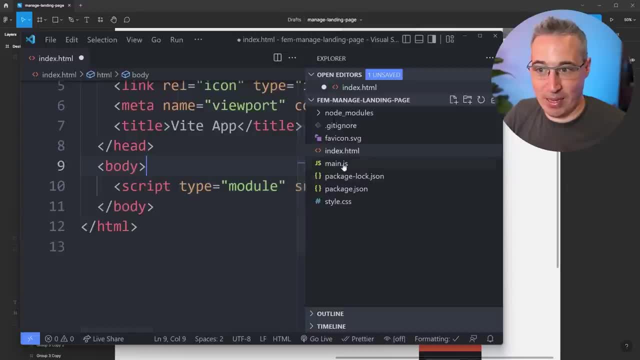 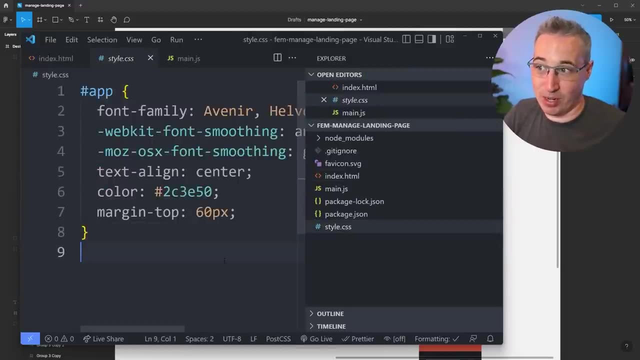 delete that. and then I'm going to navigate over into my mainjs and I'm going to delete everything that's here because I don't need that. we'll save that. we'll save that, and my style sheet has a little bit going on here, so let's copy that and we're going to save and delete that as well. now. 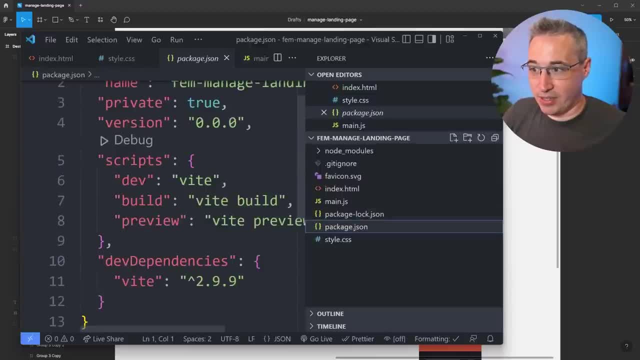 if we go over to the packagejson file, we can look in here and you'll see that there's a few scripts and these are sort of the dev dependencies, and the scripts are, for now, the most important things in it- and our build script. those are basically the two that are the most important, because we will 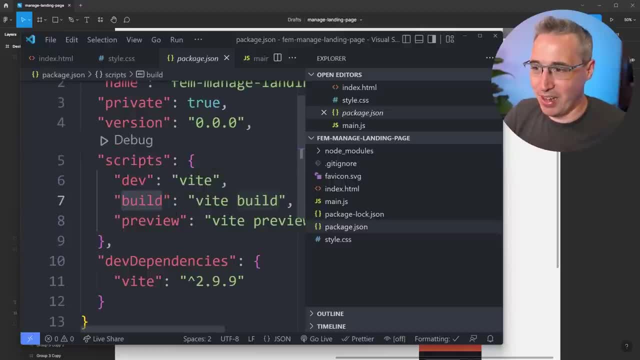 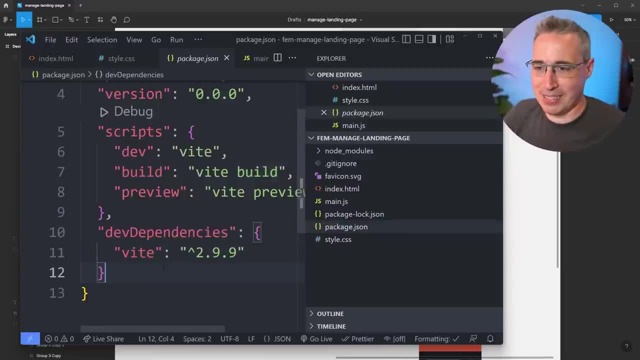 eventually get this online and working, and we'll use the build script as part of that process, and here we have the dev dependencies, which right now, is only which is going to run stuff for us, basically, and so why don't we start that off and make sure it's working? so I'm going to open up my 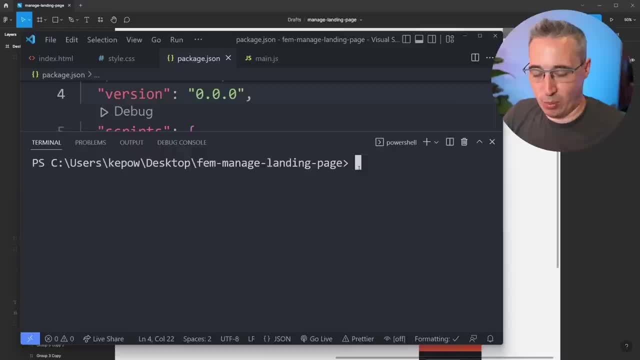 terminal again and let's just close that sidebar down because we don't need that. and but what we're going to do here on my landing page, we're going to write an npm, run dev, like it said, and this will have a dev server running right there so I can control. click on this. I'm guessing, if you're on. 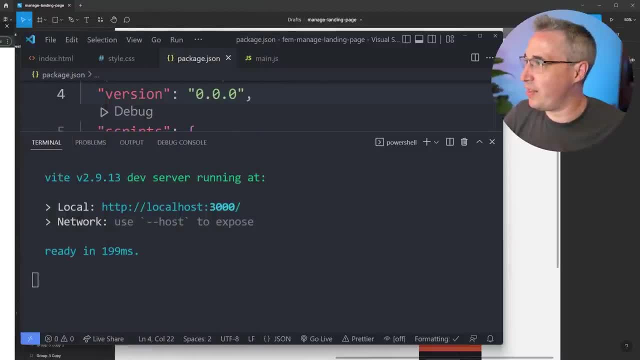 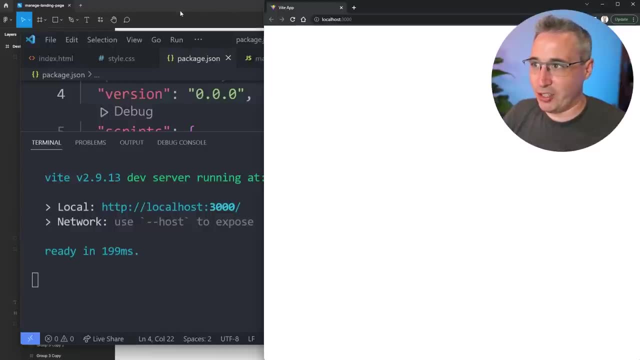 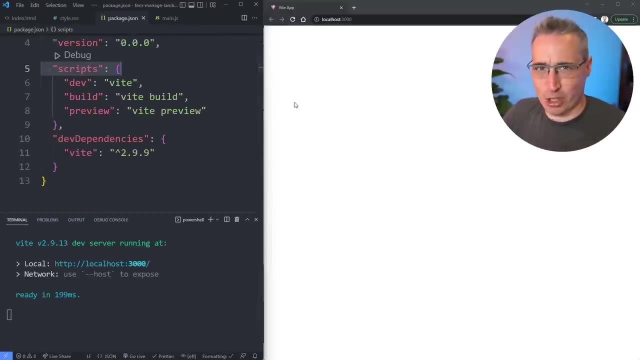 Mac. it's a command click- though I'm not completely sure- and it will actually open this up in Chrome for me automatically. so if I bring that over, we get a blank Chrome page. so let me just move things around here really fast and zoom back out. so now, with that open, just to make sure that it's actually. 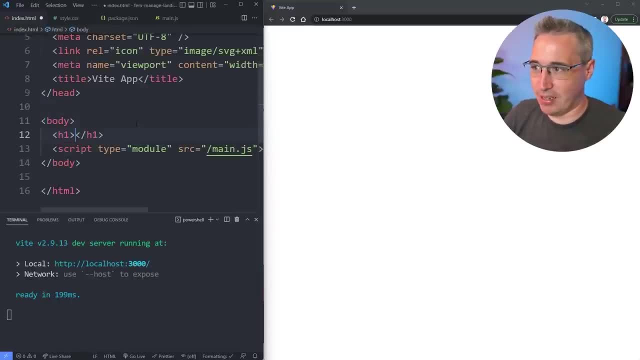 working. let's come over to my index and I should be able to come in and let's just write in hello there, hit save and immediately we can see it actually did show up over here. if I go to my stylecss, let's do a body background. 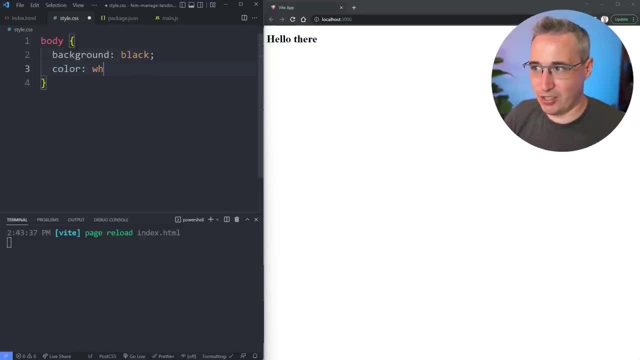 of black, color of white, just to see and ah, notice how that didn't actually work. so this is why I like testing things, making sure they're working right off the bat. so we're going to come back over to my indexhtml and that's because originally the CSS- I'm pretty sure with beat- is actually going. 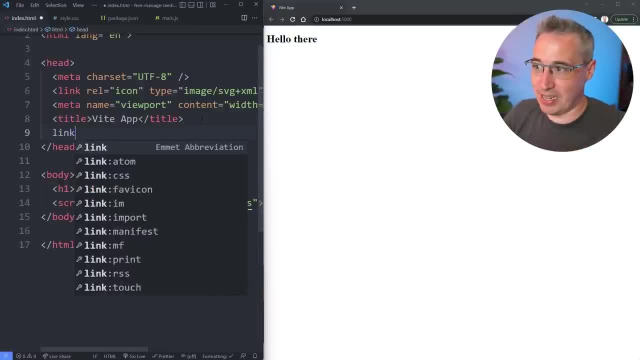 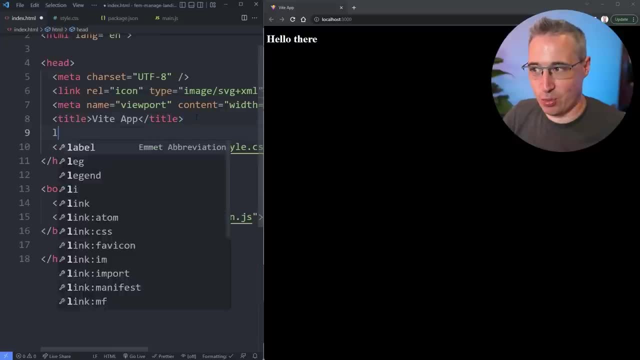 via the JavaScript. so just going to come here and let's add a link CSS, hit save on that and there we go. you will notice I did that really fast because I just wrote link colon CSS and this is just emit. that's coming in and I hit tab and it's going to make the whole thing for me. and when you do that it's the href is. 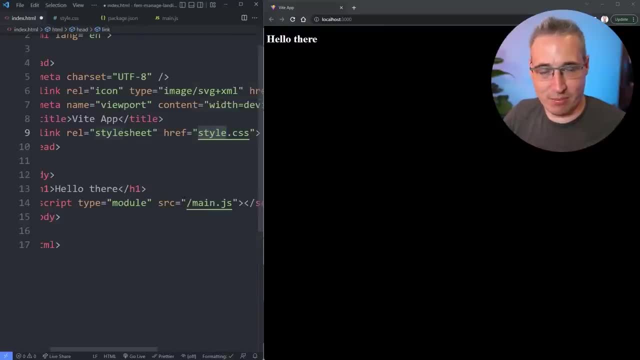 just going to be the stylecss, which is exactly what we have right there, so perfect, it's working. um, and because it's all just running, we have hot module reloading and all of that. if i change something, hit save. now you can see it's linked there as well, so we can delete all. 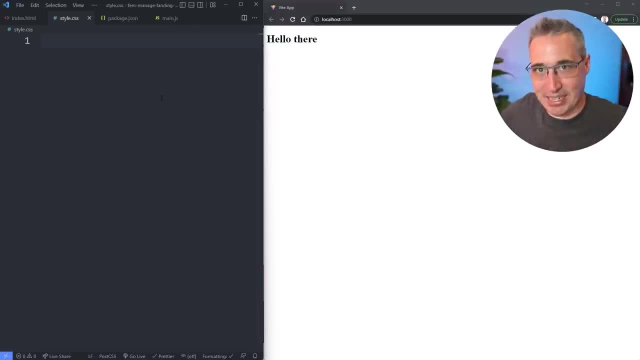 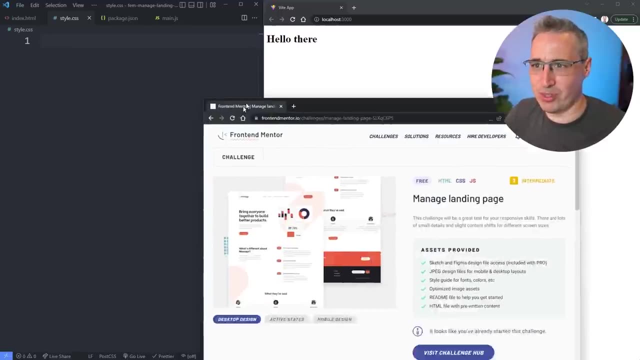 of this because we know it's working and we can get started with setting up the stage to get this project off the ground, and so the first thing i want to do is just bring in all my assets and stuff like that. we're not going to use them right away, but we want to get everything ready for the 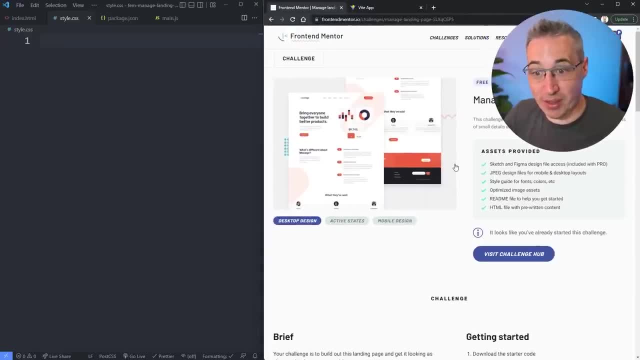 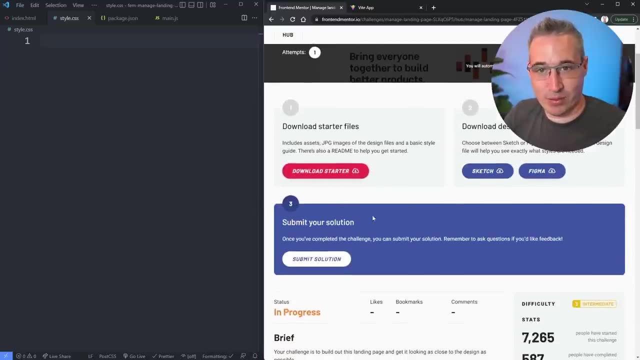 project. so if i go to the front end mentor page for this- and again this is linked in the description below- we can download the starter um and when we down and you can download the starter files and you can download the design files if you have a premium um subscription to front-end mentor. 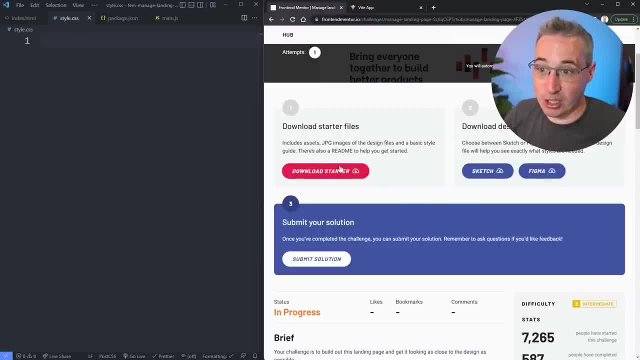 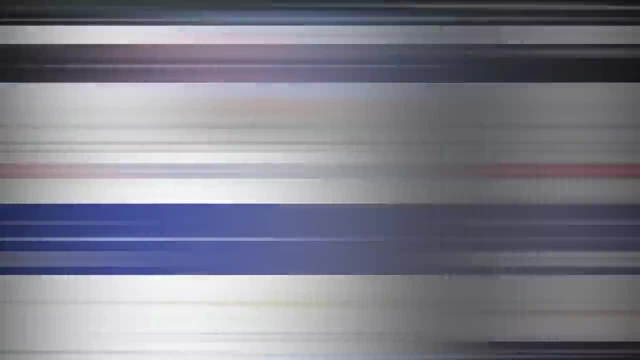 but again, you don't need this at all, uh, to get through this challenge. but let's click on download starter and get those starter files. so that gives us a zip file. i'm just going to unzip it and open up what it gives us. and here i've just unzipped the files that we got and it gives you an index. 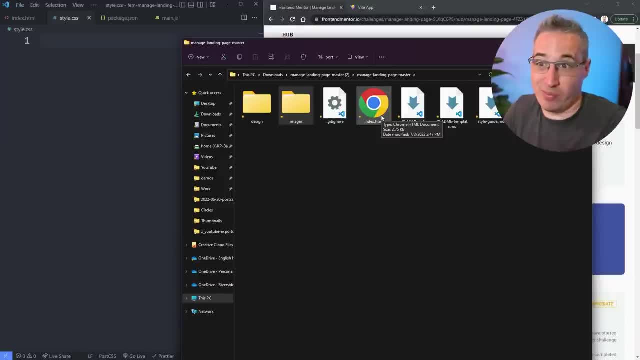 starting file that you can use to copy and paste the text from, or i mean you could work. you know we could bring this in as our index file. um, i'm just not going to do that. if we need to copy and paste text, though, that is where you would get it from. there's no structure or anything in there, there is just basically a. 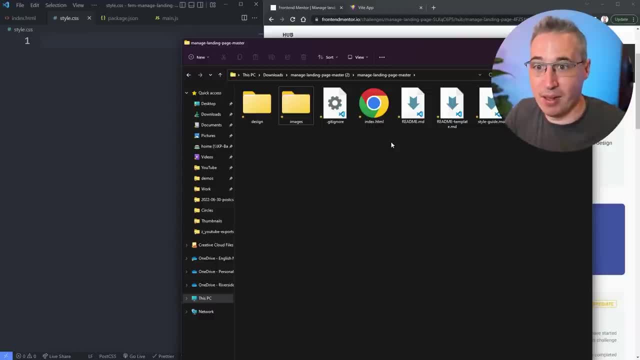 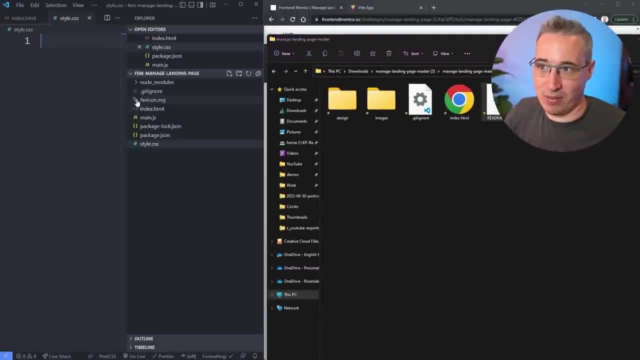 blank. um, you know, there's just all the text there for you to easily work with. um. there's the readme. if you want a bit more information, this style guide could come in handy. so what i'm actually going to do- and this is a nice thing with vs code- is in here. i'm just going to drag the style guide. 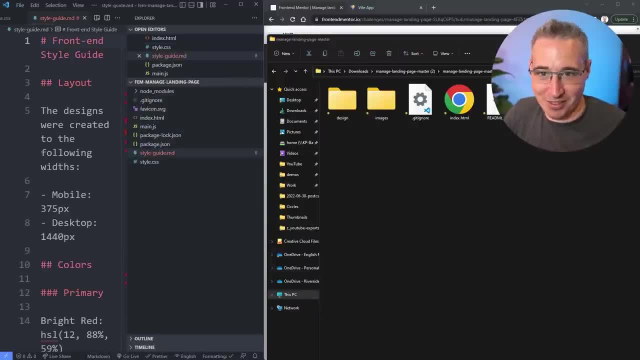 into here and it copies it over from wherever you were. no problem at all. so we're going to bring those images in because we are going to need them in this case. it's asking me: do i add it to the workplace or am i copying it? i want to copy this, so i will click on copy and i think that's all i. 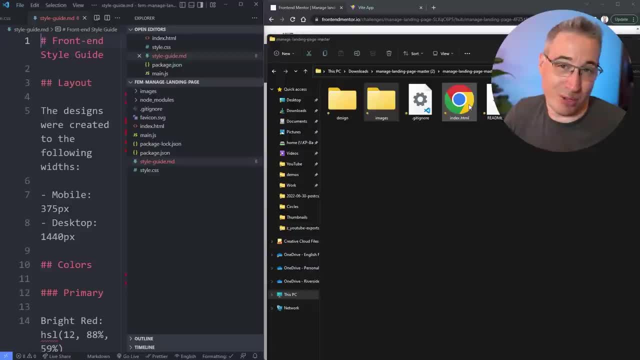 need from what they gave us. but again, if you do want to start from their index, you could bring their index in as your starting point as well. so you have all the text there. i'll just copy and paste it off from the side though instead. so let's close that down and we can look here in. 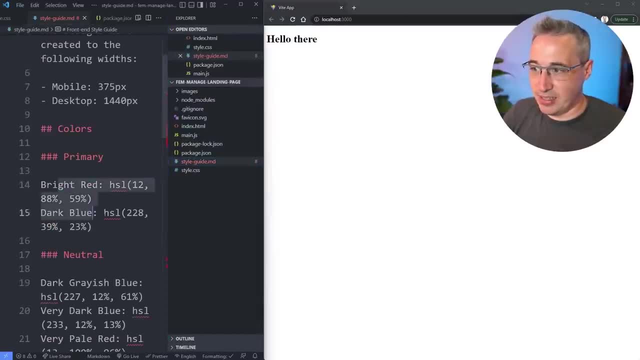 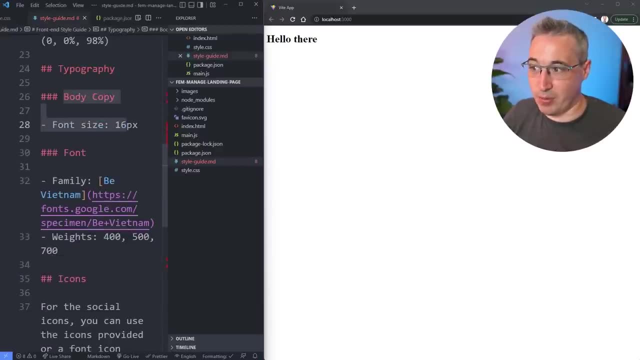 our style guide and we're going to be using this a little bit just because it does give us our colors. and there it gives us a little bit on the body, though not very much, and it gives us the font that we'll be using and the font weights- 400, 500 and 700- that we'll be using, and it also talks. 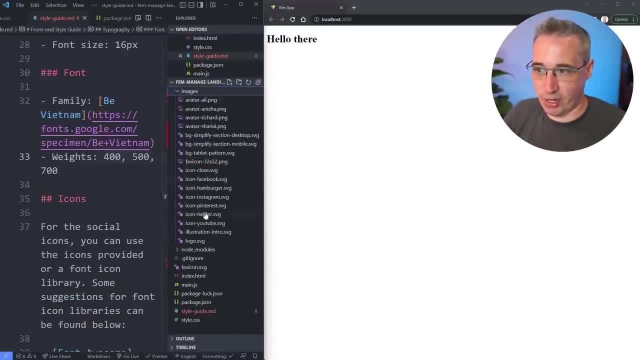 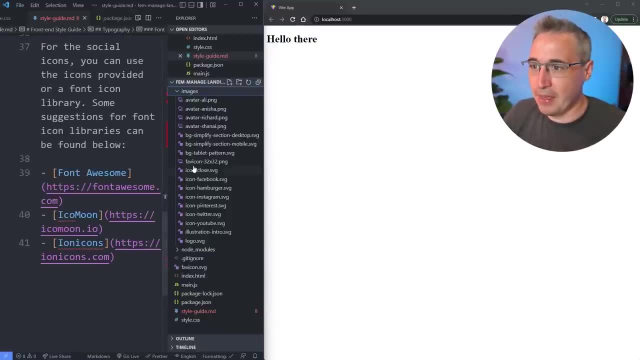 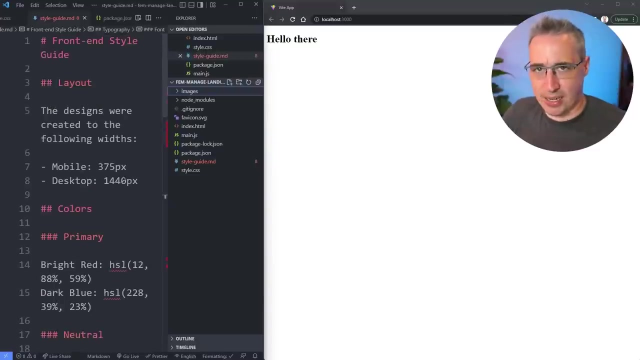 about the icons. i think the icons are also provided. there we go, we have them as svgs, or it talks about how you could get them from other sources as well. we'll be using the svgs, though, for this one, um, and yeah, i think we're we're good to get started on this, so let's go and set up the. 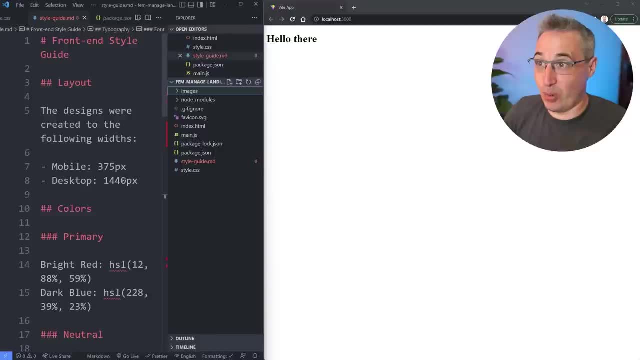 the base of our style guide, and then we're going to go ahead and create a new one. so let's go ahead and create a new one. so let's go ahead and create a new one. so let's go ahead and create a new one. so basic structure and starting things that i would like to have in place before we really dive into. 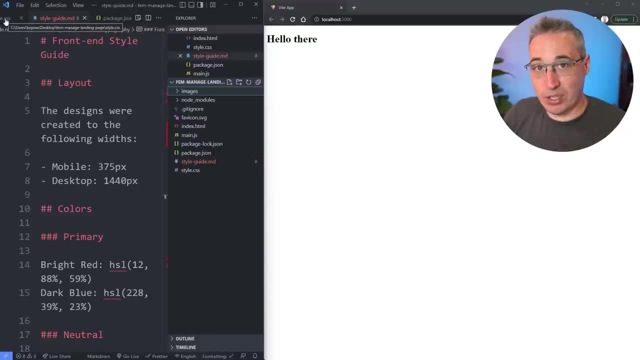 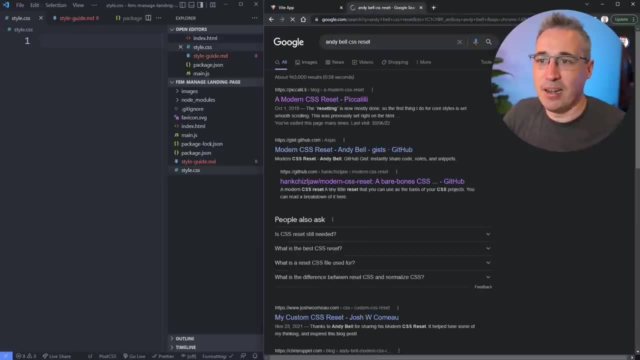 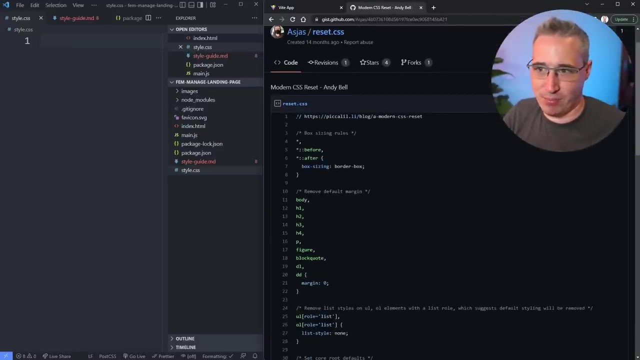 the entire project. um. so the very first thing we're going to do is get a reset in my style sheet. so what i tend to do is use andy bell's um css reset. there's another really good one by josh como. they'll all be linked down in the description, and so right here it's as a just, and you know i'm 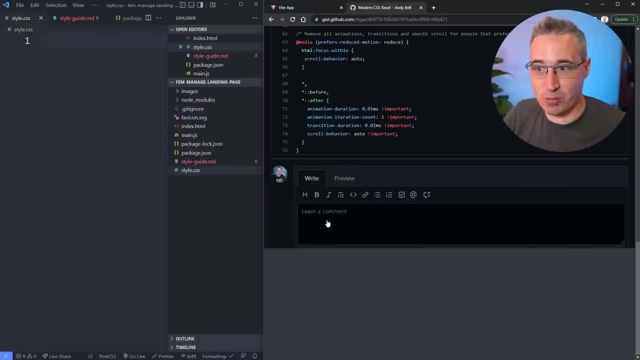 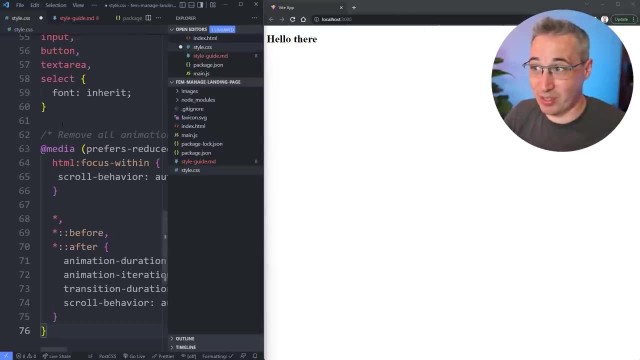 just going to come in here and copy the entire thing, though i will make a few small changes. but it's nice because it's a very basic reset. there's not too much happening because we don't need to need that. if you'd prefer to use normalize or something else, you're more than welcome to use. 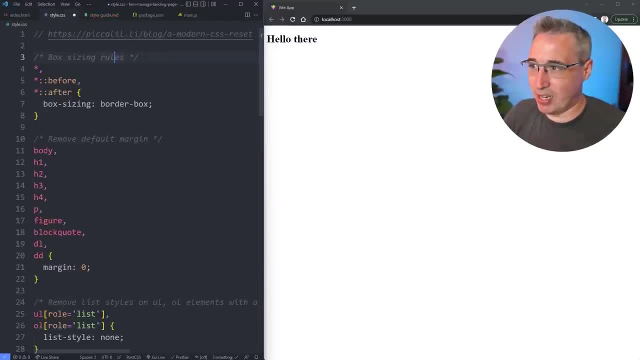 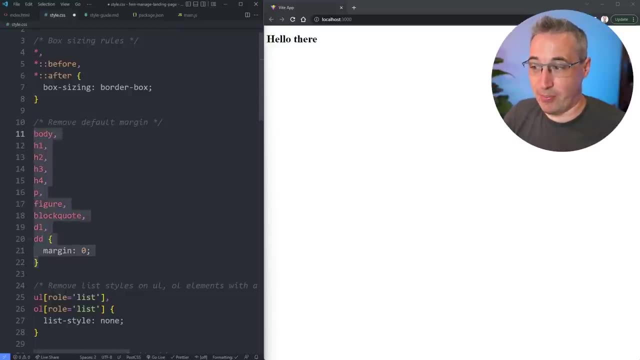 those as well, um, and let's just zoom out a touch more, and so this is always a good one to have just to do that. uh, one thing i'm going to change is actually on this, though. um, this is removing all the margins, which i like doing, but lately, what i've actually been doing is just doing a star. 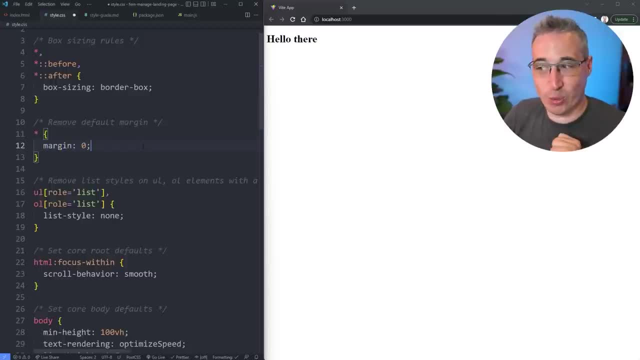 and doing a margin of zero, and it's because not only do i do the margin zero, we're going to throw a padding zero, a little bit more aggressive on this front, uh, and then we're going to be doing a font inherit, and this is a pretty strong one, and if you disagree with it, that's completely. 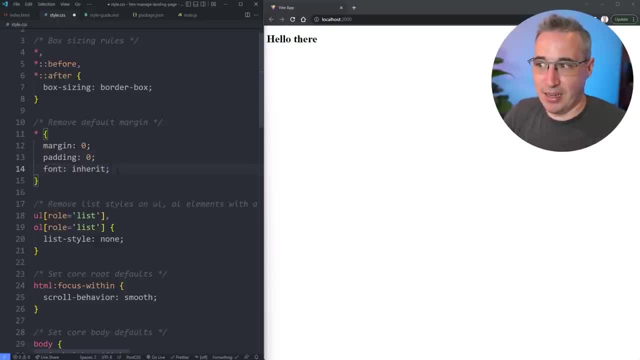 fine, uh. but what i like about the font inherit is it resets the font sizes of all of our h1, h2, h3. it takes the bold away and all of that. so if i hit save you can see it's shrunk away. uh, it also. 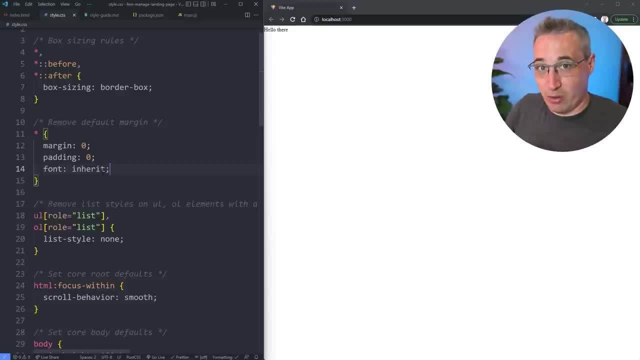 makes sure that everything is working on my form elements and all of that where normally they're not inherited. uh, but the reason i like doing that now it was mike aprichio- sorry if i said your name, i got this from and as he explains it and i think it makes a lot of sense- is this: forces people. 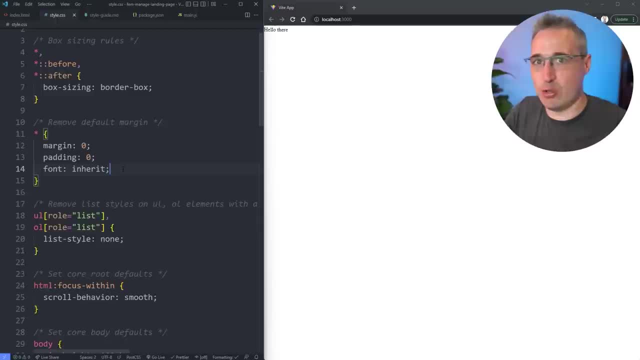 to use the proper classes rather than using an h3 to style something. so like: oh, i want it to look like an h3, so i'm going to use an h3. that's not the proper way to do it. like: oh, this looks like an h2, this looks like an h3. um, we'll talk more about semantics when we start writing the html. 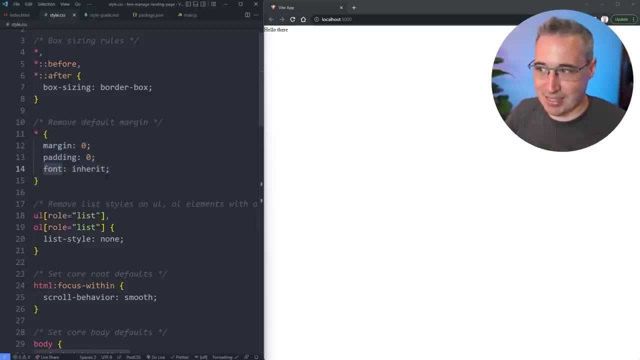 but yeah, i like doing the font inherit here resets everything, and then i build these things back in: uh, this we can keep. um, it's the role equals the font inherit, and then i build these things back in: uh, this we can keep. um, it's the role equals the font inherit, and then i build these things back in. 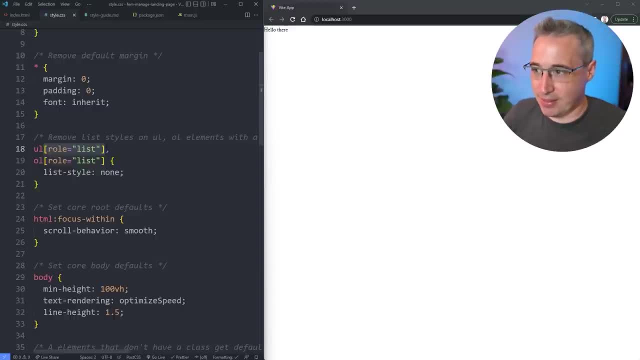 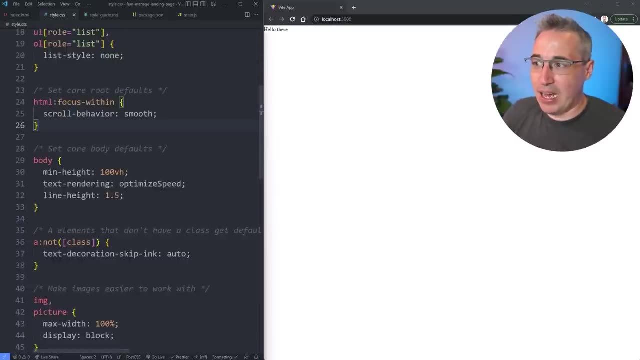 list, because you're going to be restyling that, but you want to keep it as a list, so that's completely fine. scroll behavior, scroll behavior- smooth, is always a good thing to have. uh, another thing that i've used this for, um, but actually run into a few little issues every now and then. 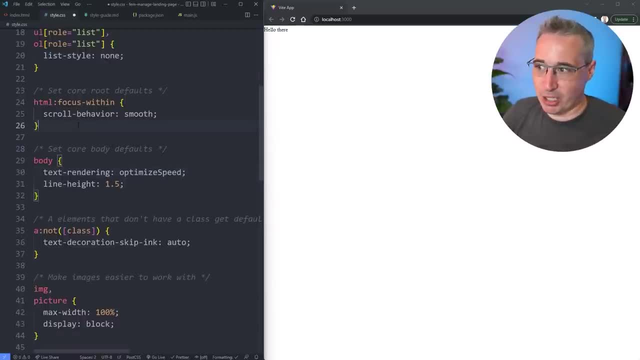 it's not very often, but instead of having the min height here, what i'm actually going to do is, on the html and on my body, do the height of 100 percent. um, and it's again not very often, but when you do need to use the body's height sometimes, this can just. 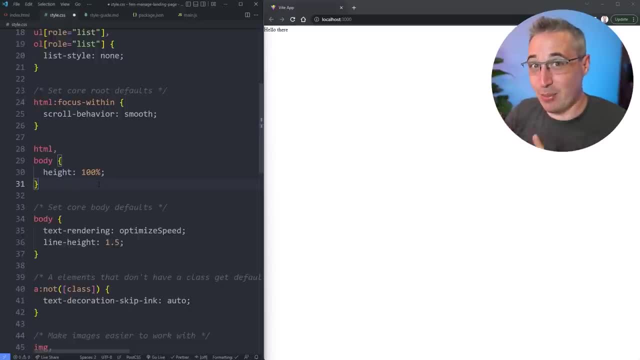 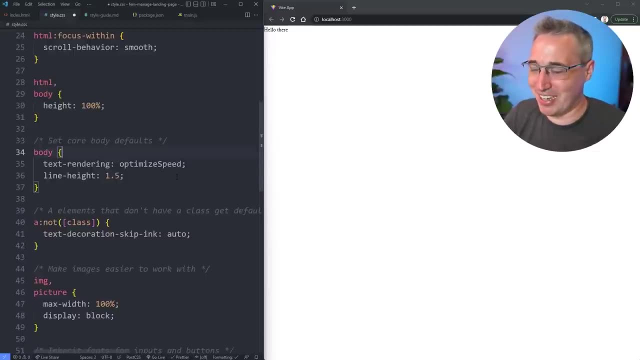 help out a smidgen, and I've actually had a rare instance of a double scroll bar once that it's because I hadn't set this up, so hopefully that that avoids those problems for me. this we can keep no problem with that, though I don't know we. 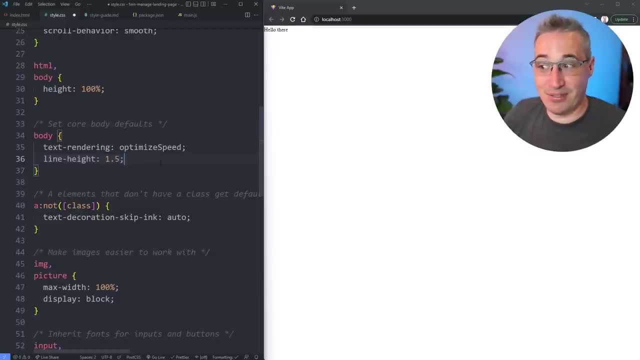 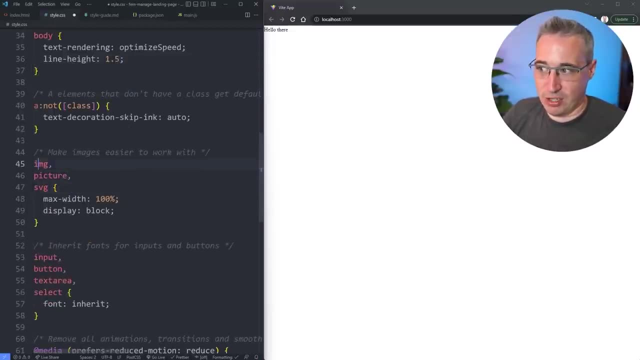 might change away from that line height, but it's a nice sort of default starting point so we'll stick with it for now. here we're also going to add SVG, so we're setting our images, our pictures and our SVG as a max width 100%. so this: 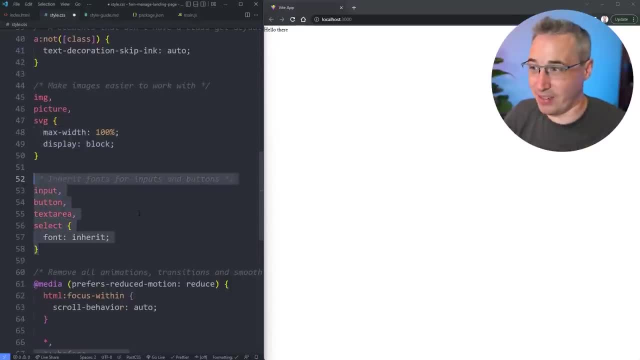 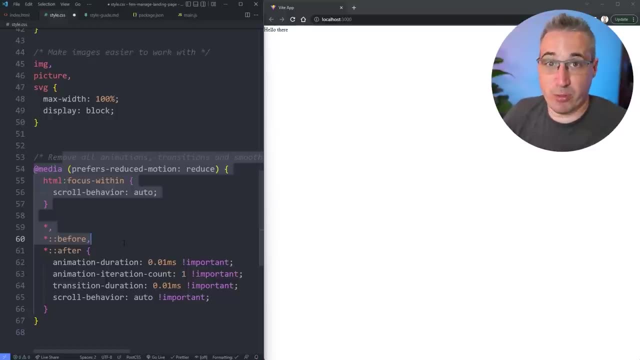 we don't actually need anymore because we have the font inherit for everything set up higher, and this is to remove transitions and animations and stuff for people who prefer prefers reduce motion enabled on their system. it's not a hundred percent perfect, but it's a nice way just to have that as at least set up. 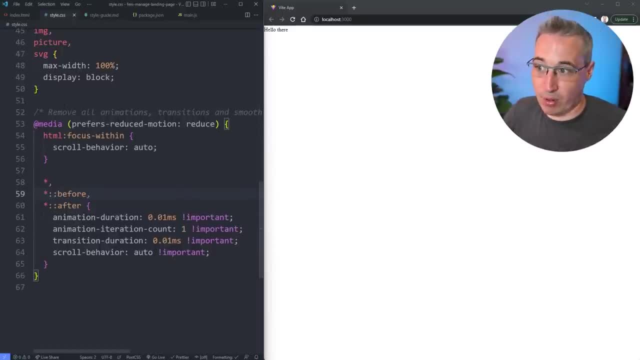 for that, to prevent that. because it is important that if somebody's disabled animations, it often is because they just don't want to. they're, they're made uncomfortable, sometimes by a lot of movement and a lot of animation on a page. it doesn't mean there should. 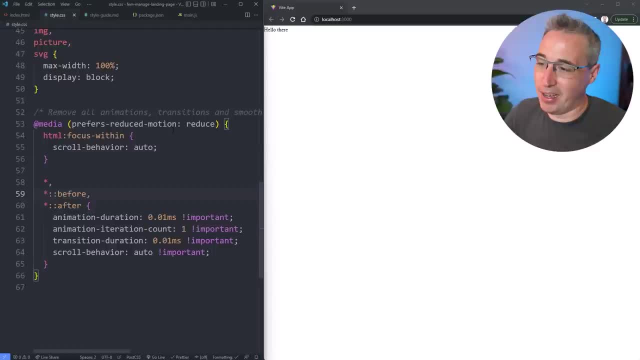 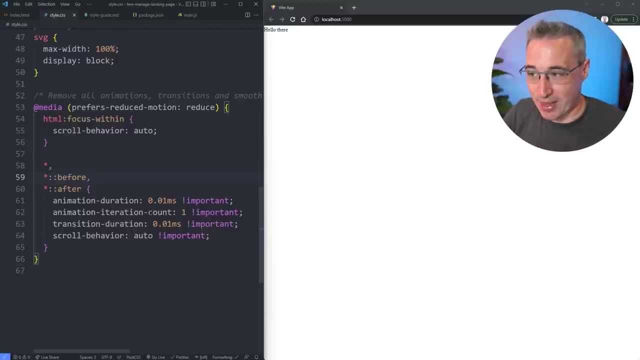 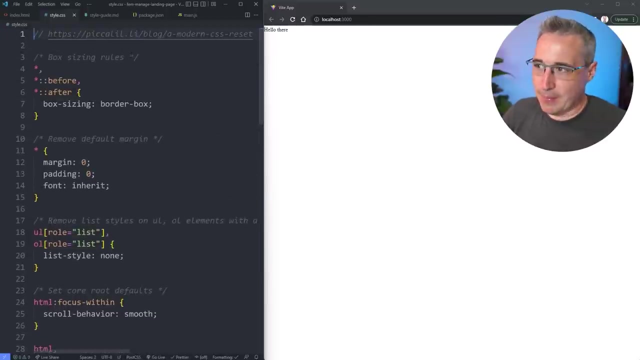 be zero. it's prefers reduced motion, not zero motion. but yeah, I'll put a link where you can read more about this if it's something that's new to you. but yeah, that's what we're going to include right there, and then the next thing we're going to do is: let's come all the way up to the top. I'll actually keep 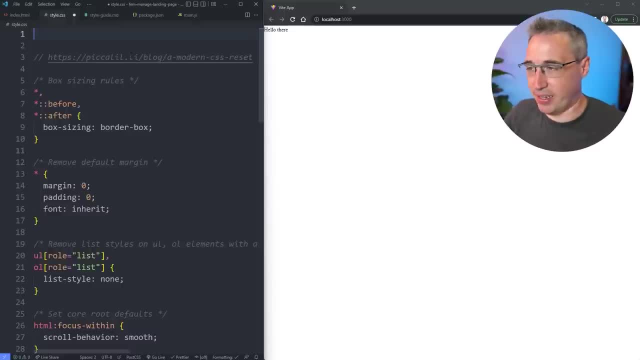 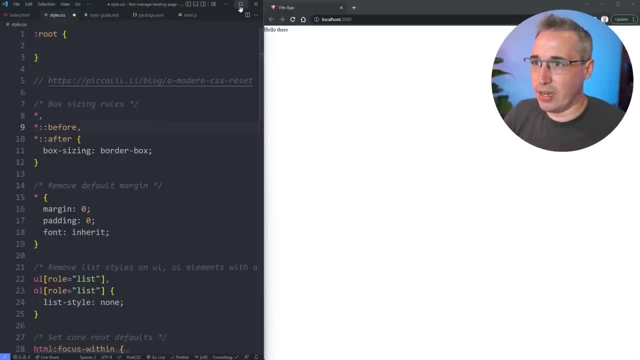 that comment in there, just so people can access it. if they're accessing the github repo from this project and then we're going to go ahead and add our github repo and we're going to come here and go to my route and the route let's switch over to our. actually let's go full screen here on this. we're close. 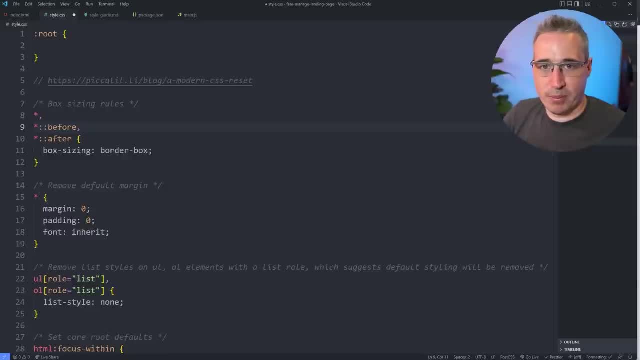 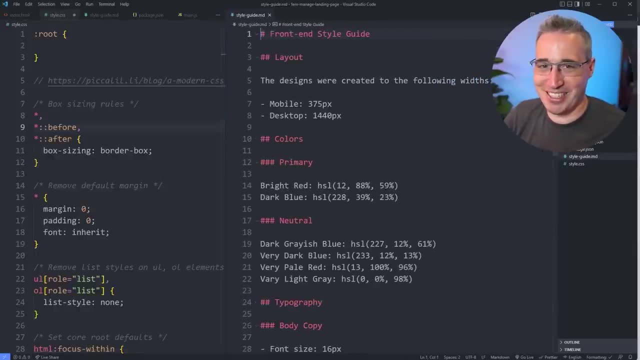 to full screen. we can go full screen and let's open up my style guide and we're gonna open it on the side. so we have my style guide. you know, we split it apart a little bit, which makes it easier to access the two of them. one thing in VS. 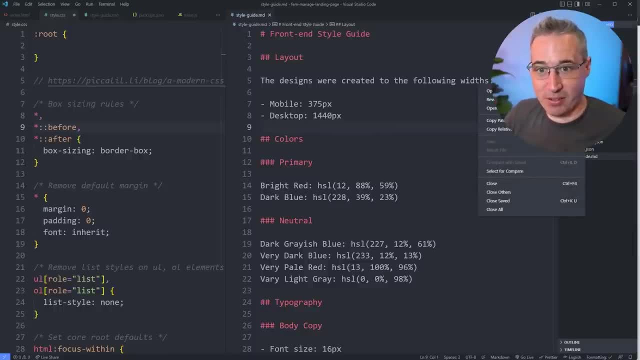 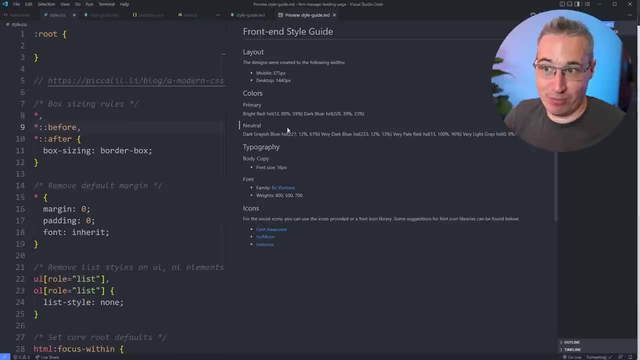 code. actually, if you right-click on a markdown file and we can do an open open preview right there, or we can do an open preview right there, or we can do an open preview right there, or we can do an open preview right there, or we can control shift V and it opens it up in a prettier, a little bit easier way to. 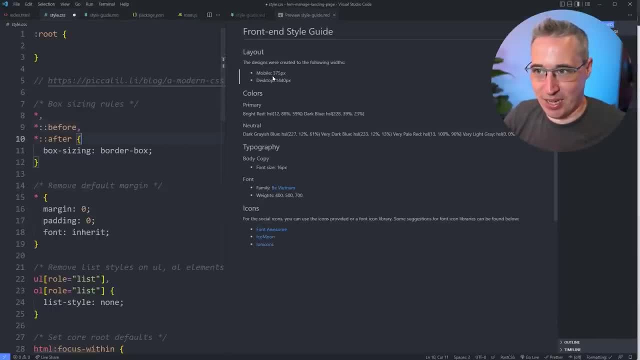 read. so whichever one you prefer, we can do that now. I know it's a little bit small, but at least we have our colors a bit easier to access here and let's come in and set up a few things that we're gonna do. so we are going to set up a few. 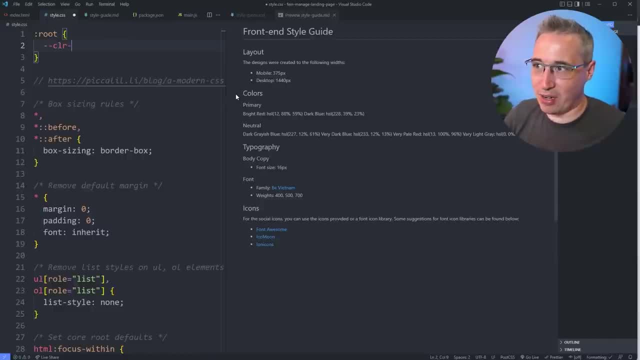 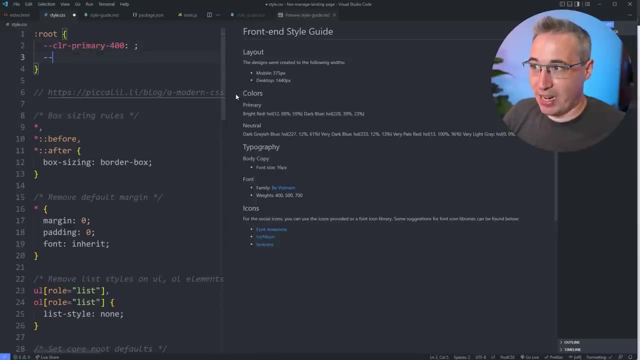 colors. it's not a lot of colors in this project, but we're gonna have our color primary is going to be that orange and we have sort of that main orange. so that's gonna be my color primary- 400- and then we're gonna have a color primary. 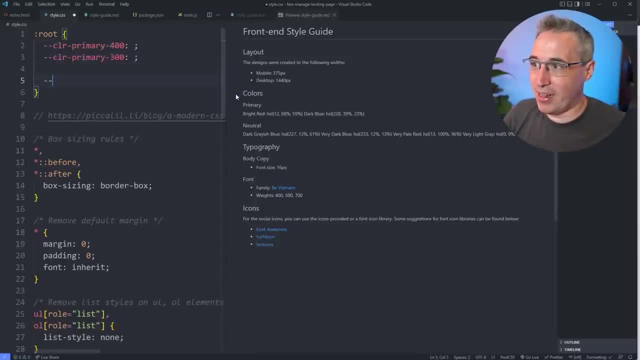 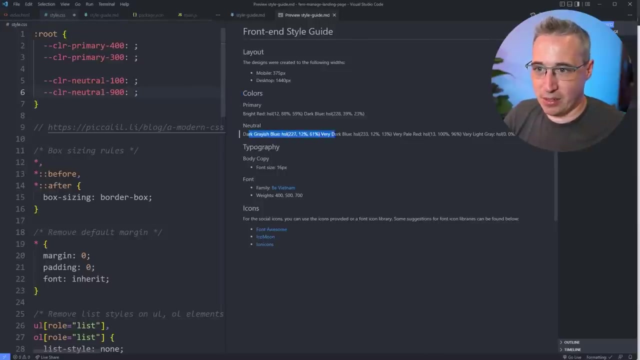 300, which is the lighter version. then we're going to have my color neutral light 100, which is going to be white, and my color neutral 900, which is gonna be the darkest color that we do have in here, and it does look like we have a few. 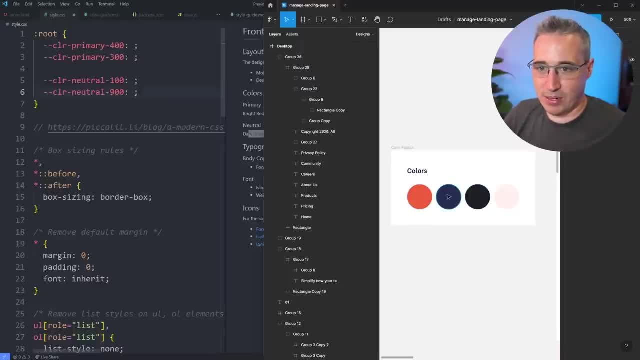 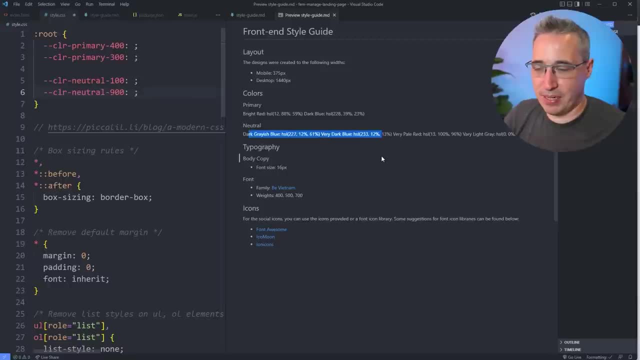 others. let's just open the Figma file really fast. here we're only we have the blue. I'm just I'm curious, because here there's only the blue that's listed, but here, Actually, this primary is going to be a 100 because it's super light, that light, light, color. 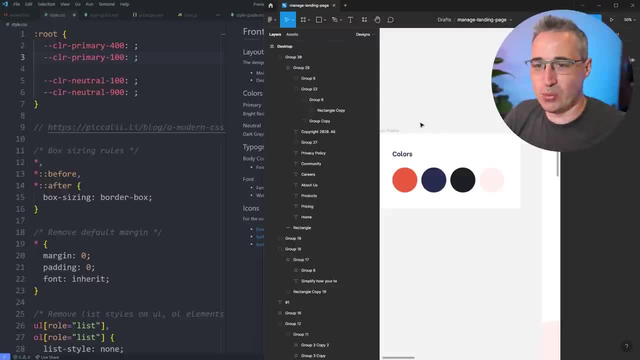 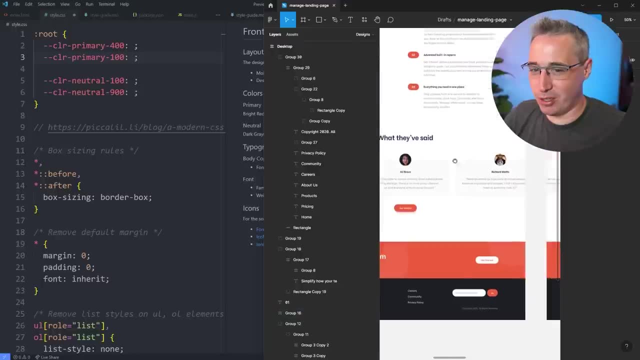 Here we have a bright red and a dark blue. So this is one of those times where I'm looking at something and I'm like, hmm, what colors are they referencing? So we have a really light gray that's coming here too. that I'm not too sure about. 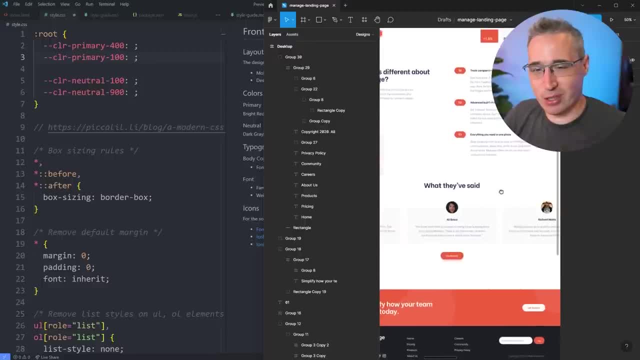 And so actually I'll show you how we can get colors. I'm on Windows so I know that we have the build. So Windows shift C is a color picker and you can actually color pick. So if you don't have access to the Figma file, it takes a second to open the first time. 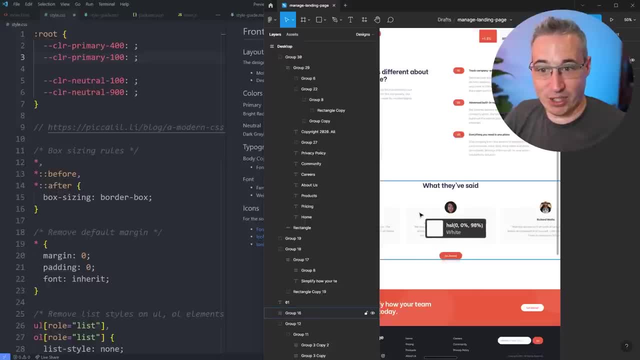 There we go And you can see I have my color picker now. So if I go on something, I can actually see what it is and I can get the value. But if I click on it it also pops up in an overlay. 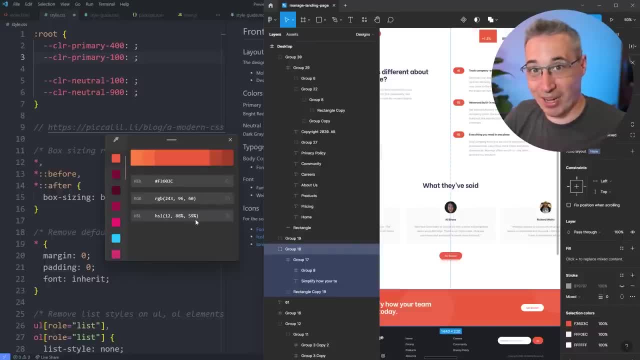 There we go, And I can get the colors really easily in whatever way I want to access those colors. So if you're just working off a JPEG, this could be a nice way to get them. What I'm going to do, Hmm. 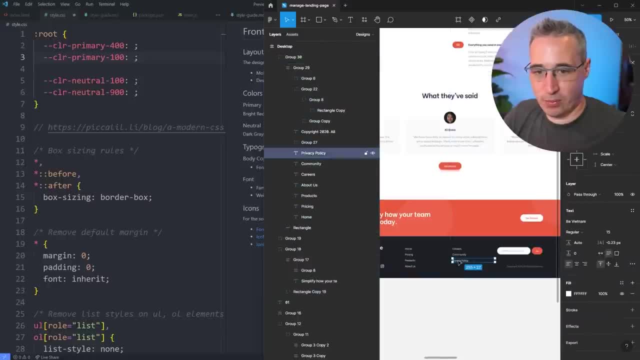 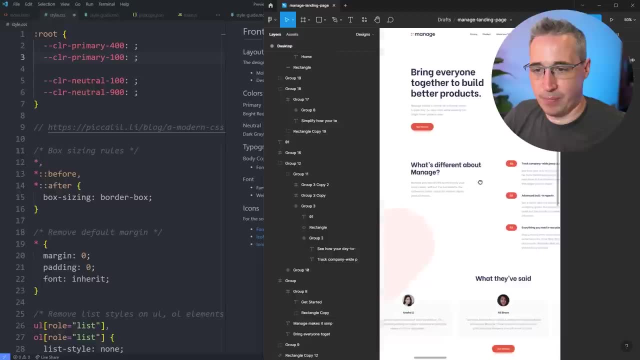 We have that color here as well. What color is this? This is just white. I'm just trying to figure out where those colors they're talking about in the markdown file are. Hmm, I'm not too sure, So I'm actually going to grab the colors from the Figma file. 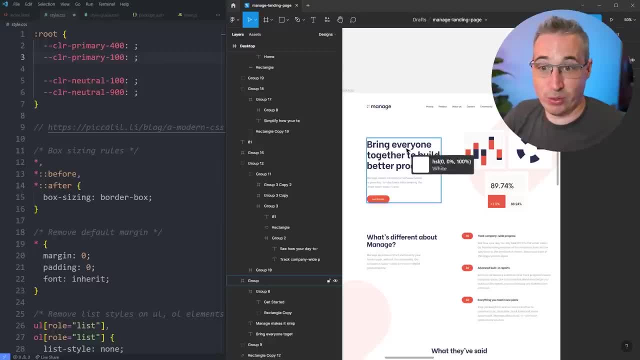 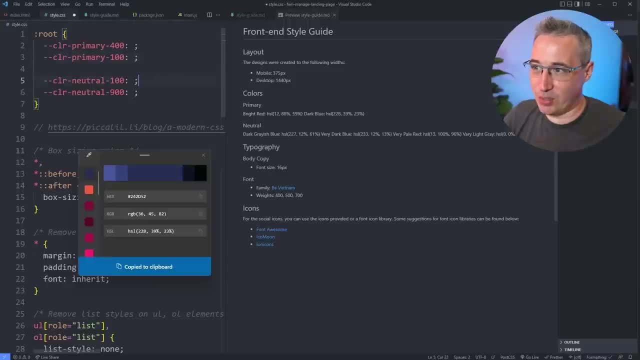 But we'll do it the way the control shift or Windows shift C, just so we can grab them this way. And I like working in HSL, So I'm going to grab that. That's going to be the blue color. Okay, we have the blue. We'll call that. 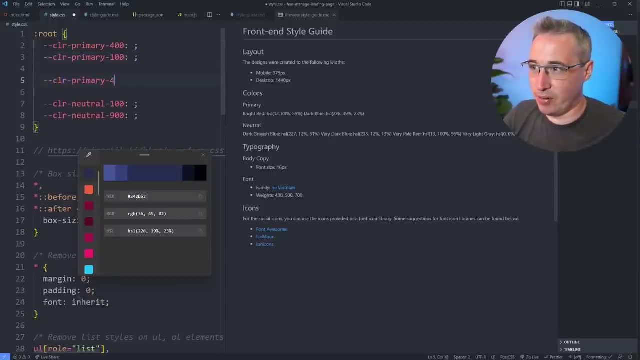 We're going to change things. We're going to do color primary. 400 will be my blue, And this one and this one are going to be my accent color, which is the red, the red color we're going to use, and then we have the neutral, and if any other colors do pop up, we'll add them to our system. 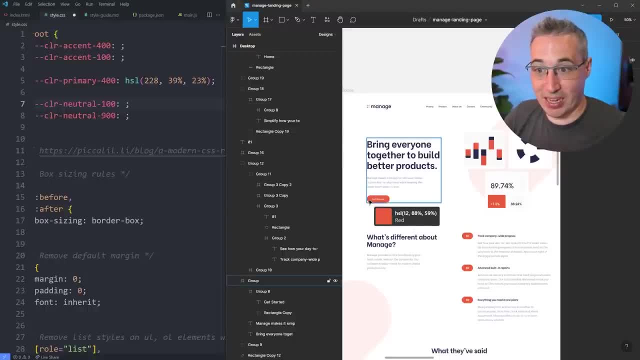 I think that's what we're going to do, And so I'm just going to go through quickly and fill those out, So you don't have to watch me copy and paste stuff and I'll see you in just a second. Alright, so I've brought the different colors in here. 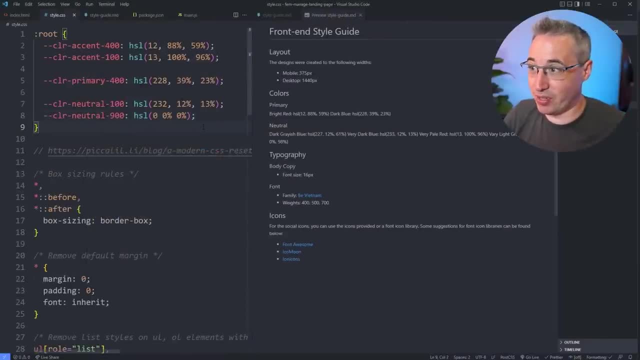 And, as I said, if we run into any problems dealing with the colors, we'll deal with those when, when we cross that board. So yeah, there's the colors that are going to be there. Then the next thing where we need is my font stuff. 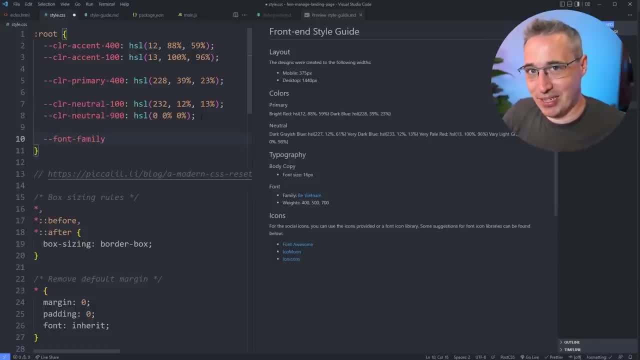 So let's say font family. I tend to like splitting things off. We only have a one font family in this case, But it's what? sometimes it can be actually useful to like, thinking long term, have a separate font family setup. So what I'm actually gonna do is font family. 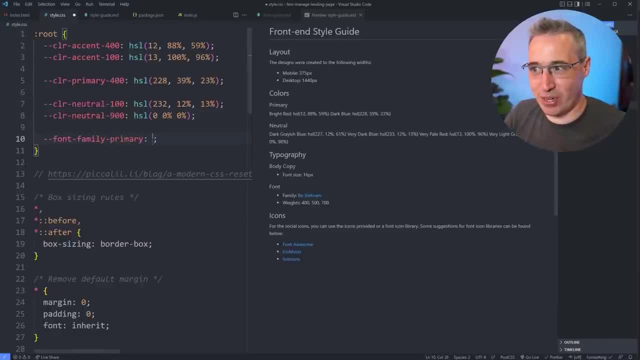 primary and this is. you might be saying, Kevin, this is overkill and it could be for something standalone like this, but I'm always forward thinking where, like this project, a year down the road they might keep the body font the same but change the heading font. 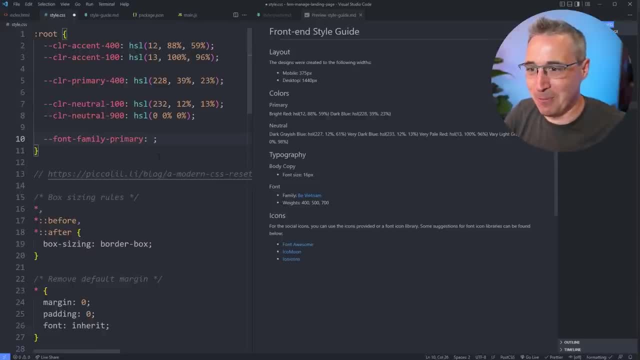 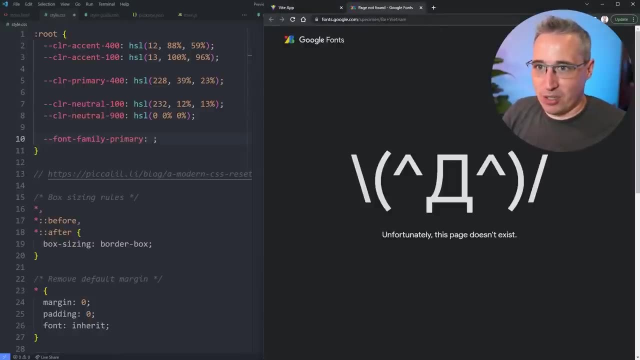 and I want to make it really easy to do that. so I'll show you one way we can do that, which is my BVietnam. so let's go and look at that and get it from Google Fonts while we're here. unfortunately, this doesn't exist. oh no, let's, let's. let's see if we can find BVietnam here. 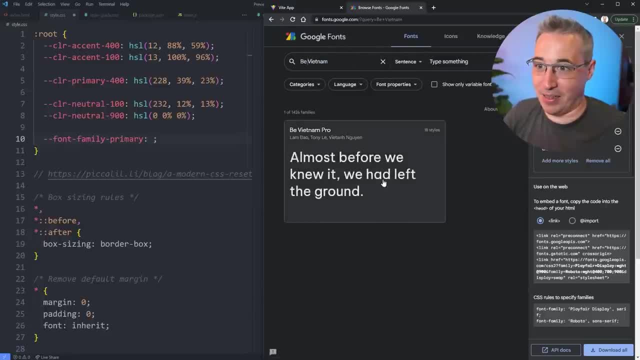 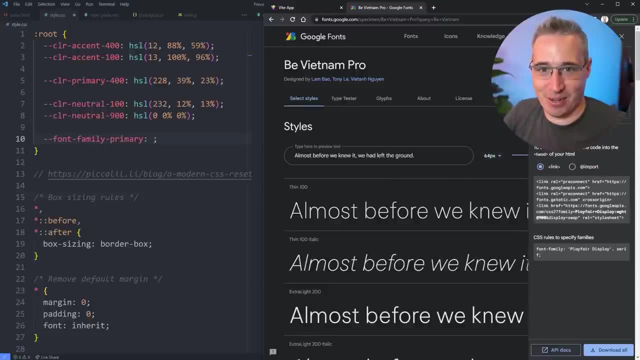 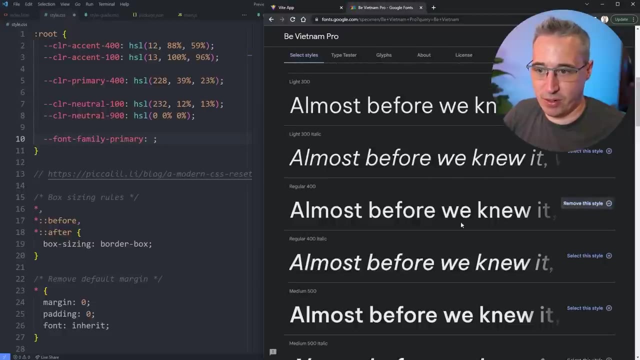 and if not, there it is, oh pro, they changed the name of it, I guess. so these are the last ones I was using, which we don't need. play fair. I also don't want remove all. there we go. we need the 400, the 500 and the 700. so that's three. there's 400, we need the 500 and we need the 700. I'm guessing. 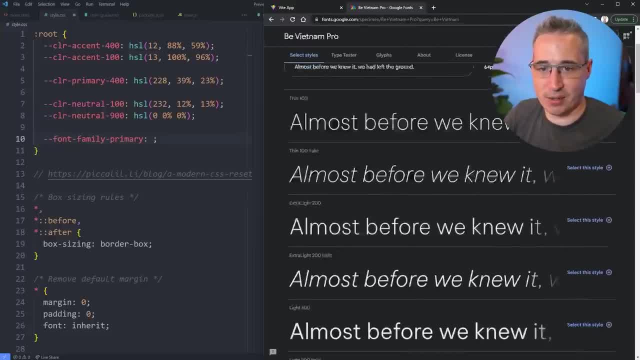 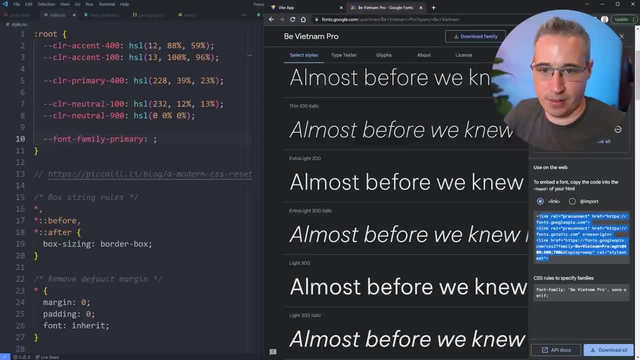 this isn't a. I'm just looking really fast, but it doesn't look like it's a variable font, so that's okay, we have everything we need there, so I guess we might as well grab this right away. copy that. it'd be really nice if Google included a really 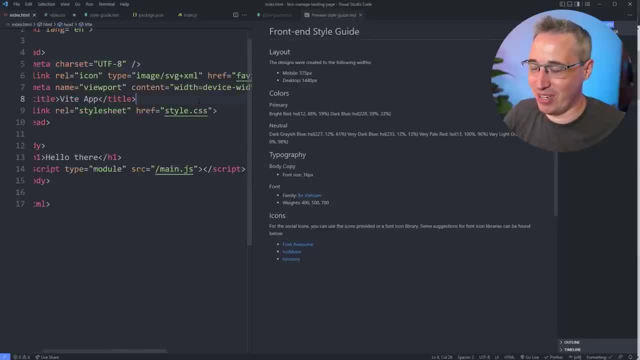 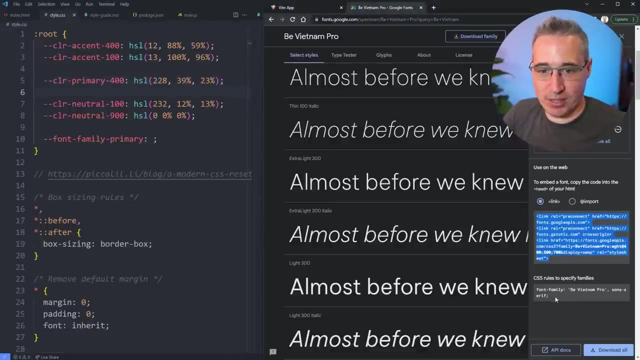 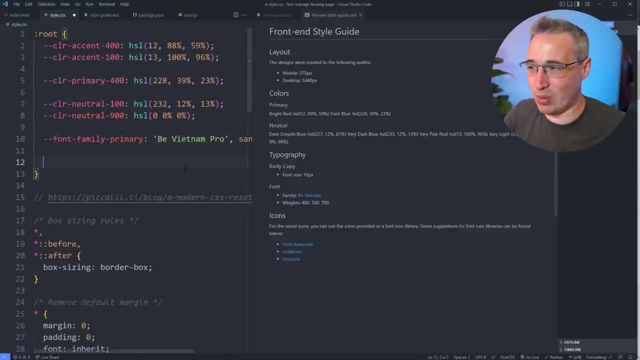 quick copy button, but anyway they don't. so we'll come right here right above my own styles and just paste that in so we get access to the Google Fonts. and then what we want is: my font family is right there, so my font family primary will be this, and then what we're gonna do is we're going: 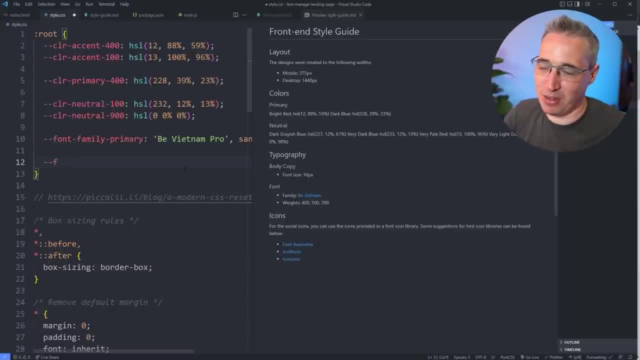 to save my font family, or I wrote font family. I usually do it like this, and then I'm going to do FF. we're actually going to change this. I was writing it out again there and I'm like: wait, why font family primary? so font family primary. and then I'm going to font family body, which is going 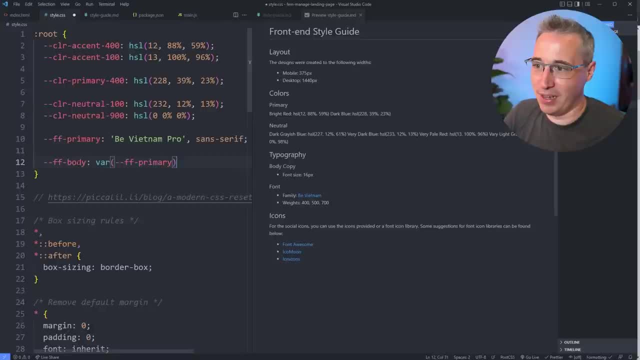 to go to my var font family primary and I'm going to do my font family heading, which will be var font family primary instead of heading sometimes. here I also will call this accent. you might again say this is a little bit of overkill, but the nice thing with this is if I set up my custom properties. 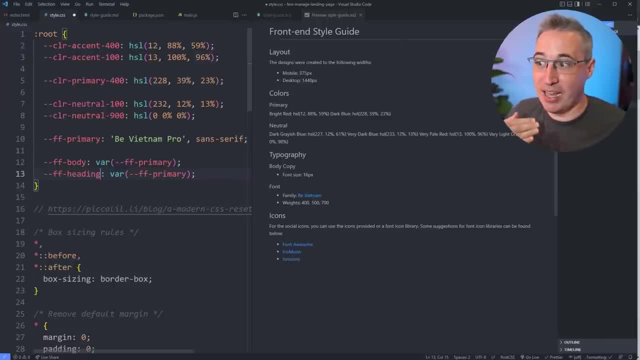 in this way, the project does get updated later down the road and I have all my headings pointing to this and my body pointing this, and I just need to change one of the two of them. I don't have to go through every place I've used it, I can just go. oh, all my headings are now just going to be. 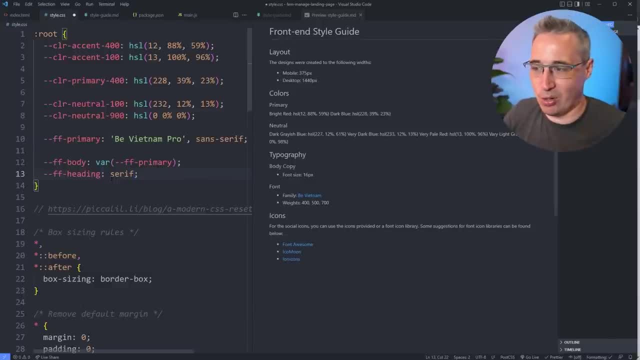 a serif font and I switch it over or whatever it is, so I don't have to have like right now. they're both pointing at this. so updating this can update the entire site. so we're just sort of gonna add a layer of abstraction by doing something like this, and we could definitely do this for our colors, as 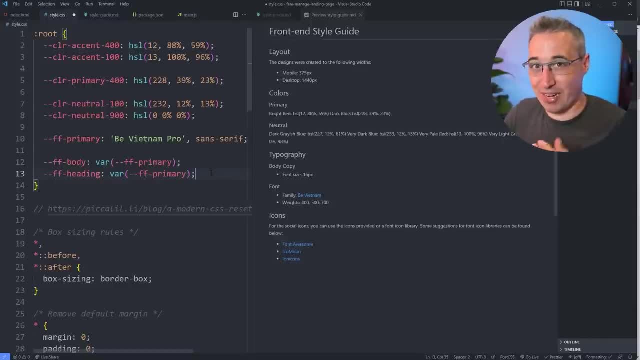 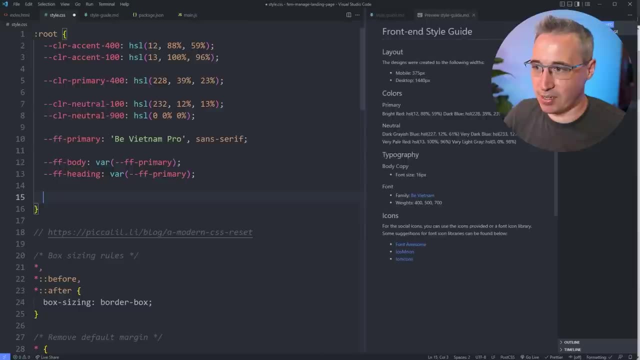 well, um so having I tend to do that more if I have sass. but for font families I'd like doing this, but if I had sass, I'd probably abstract out my colors more. but we're not going to be using sass in this project, so I think we can just keep our colors like that. we need our font weights as well, because 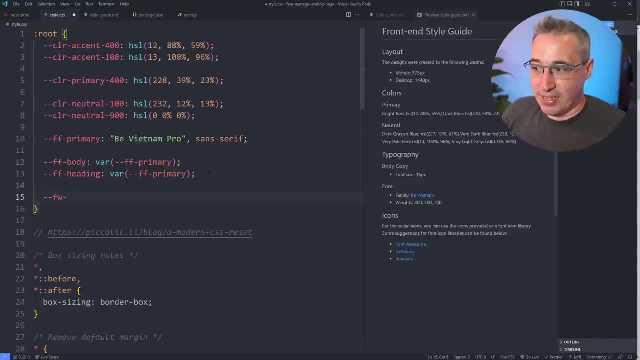 we do have three. so, um, font weights. I tend to do- I actually for this- because we have a 400, a 500 and a 700 and for some reason we switched away from our preview. I guess it's easier for you to see because the font size is different, and I'm going to go ahead and do that and I'm going to 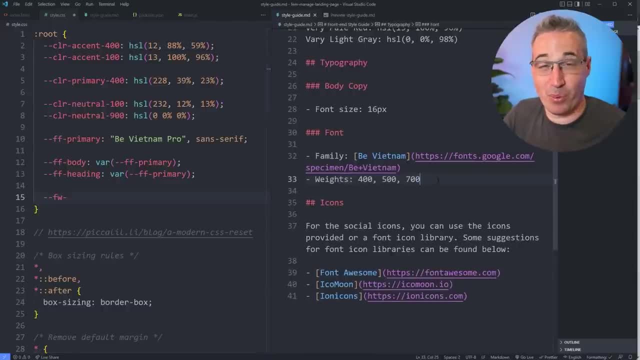 do this is pretty small on another one. so we'll look here and we have these four different or three different weights and I want to see how they're being used, because I want to know where the 500 is being used actually before I name my variables here. so let's jump back on over to figma. 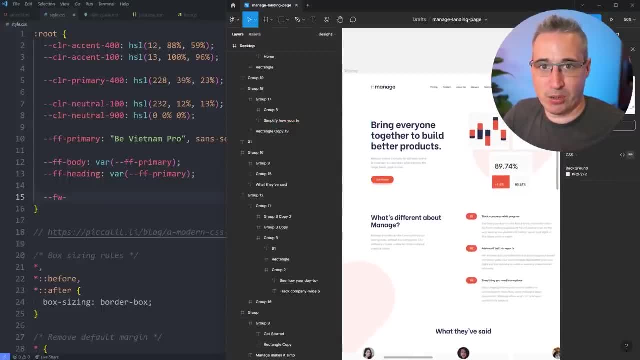 and just take a quick look in here I'm going to go to the inspect version, because then I can just get information a little bit easier. so that's 400. this is my 700. these are so my navigation is. that's interesting. and what about the buttons? they're probably bold, though that's 700.. uh and 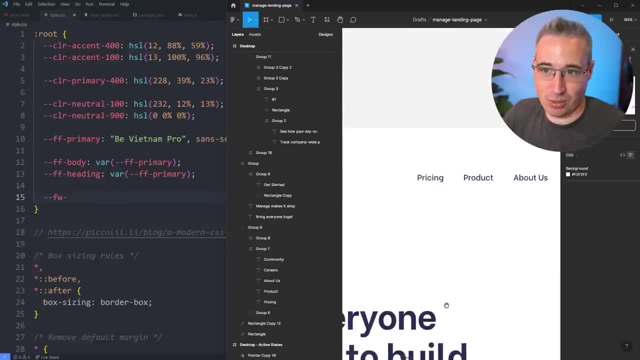 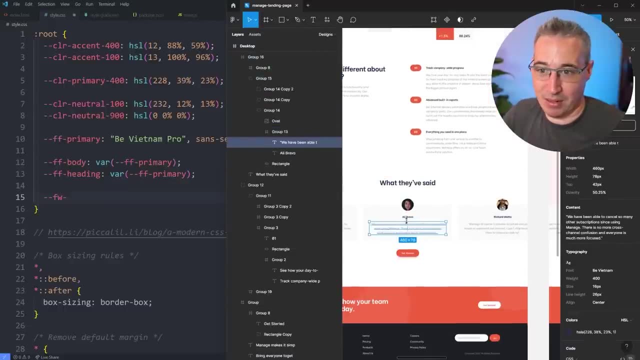 if, again, I have the advantage of having my figma file. but if you come and take a look you can sort of they look very similar to the four in the 500. to be honest, maybe it's not even worth having the 500, but I'll stick with. the design I'm just going to poke around is the only place the 500, that's 400. 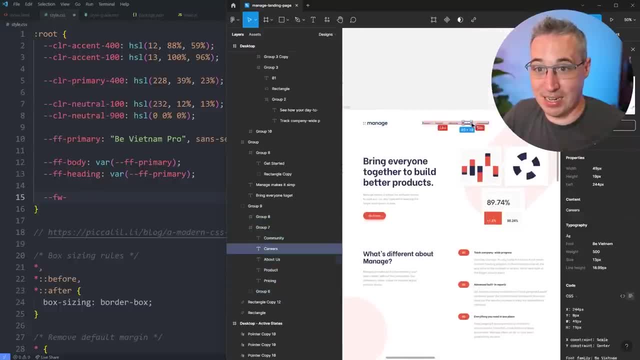 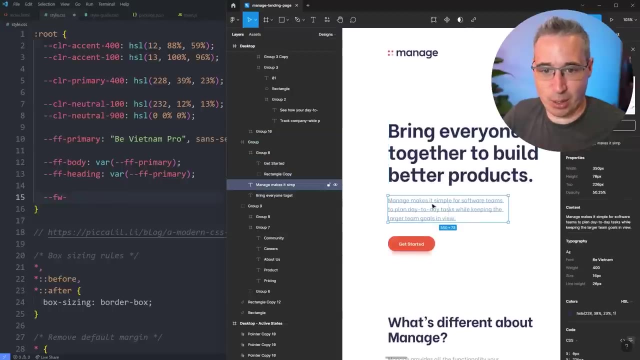 that's 400. the only place the 500 is being used is the navigation, with a really small font size too. um, I have noticed with front-end mentor projects- some of the older ones- the font sizes get a little low and the contrast ratios sometimes get a little low. uh, because here actually I was looking at the 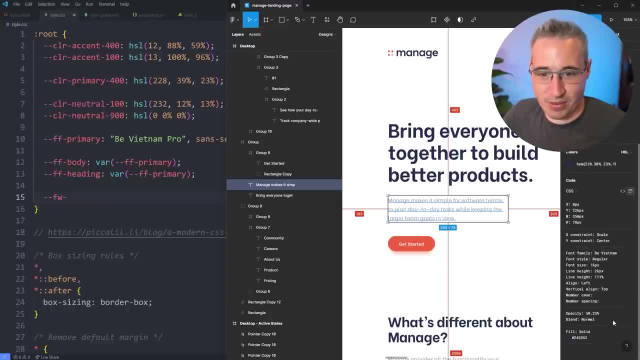 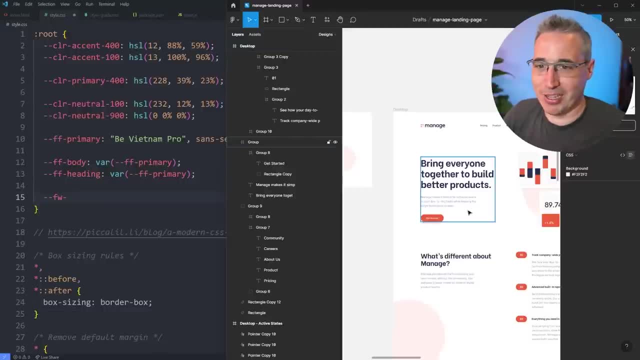 color of this and it's using the dark color, but I almost feel like there's an opacity. it's at 50 opacity. so I'm going to set it like this when we get there: but we'll talk. we'll talk more about that later. actually, we'll talk more about that when we, when we cross that bridge- um, oh and that. 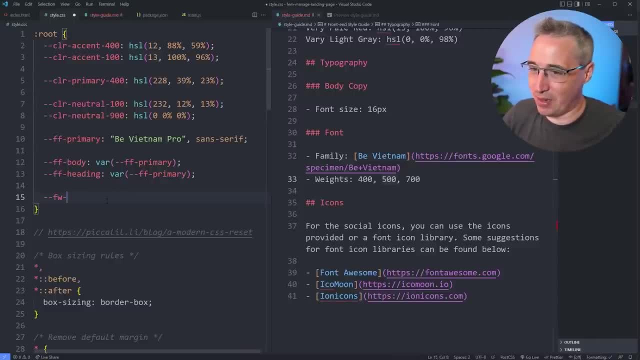 actually lowering the opacity. oh, there's a way of doing that. actually we'll be okay. um, but I think just regular is my 400 and my font weight bold is my 700.. um, and I guess font weight semi bold will be my 500.. I'll use it just because it is in the design. um, you'll notice I'm using regular. 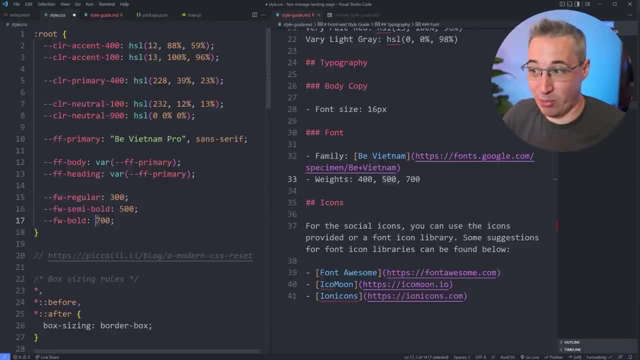 semi bold and bold. it's because on some designs your regular will be a 300 and your bold might be a 900.. so it's kind of funny because I use the font weight numbering system for my colors, but I don't actually use it for my font weights, um. but yeah, that's the reason why. 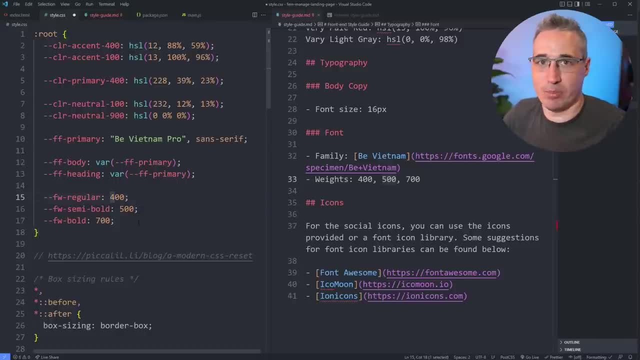 I? I do that because it makes it easy to have a regular that's 300, or a bold that's 800 or 900, uh, rather than linking it like when you have 700 here and then this is a 900. it just feels a little. 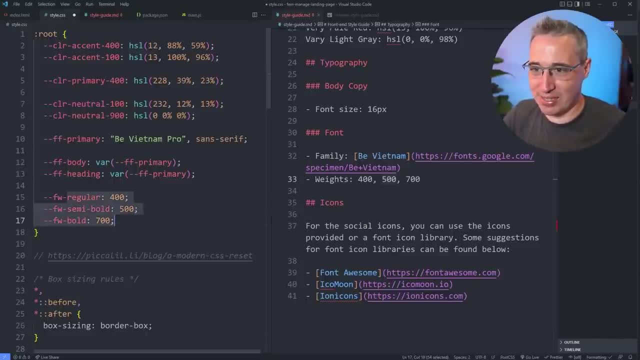 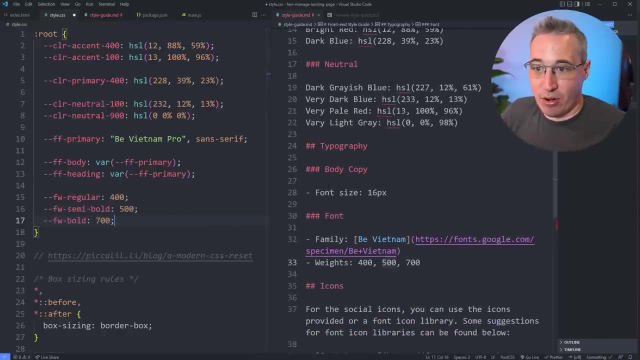 weird, but whatever you want to go with. um, but I do want to set up as many of these as custom properties, because it just keeps a lot of my styling in one place afterward. um, and is there, there are the font sizes, and in this case we don't have any in the design system, in the figma file. 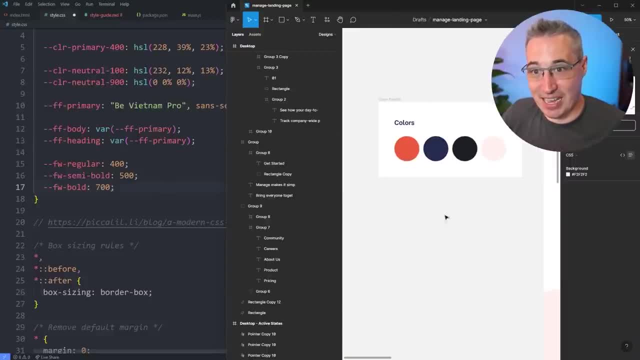 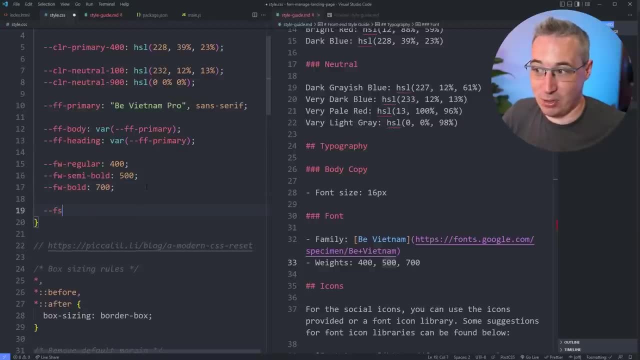 um, sometimes we have more information here. we don't have anything that's in the actual one. I'm going to grab the font sizes that are in the figma file and so I'll just run through that really fast. so I just do font size and I try to do 400 as my body, which. 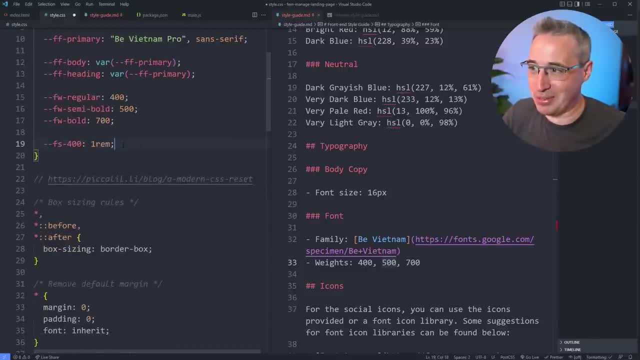 in this case, I know is one rem, because I poked around when I was getting my colors. uh, so we get my one rem there. then I'd have my font size 500.. I don't know how many. we're going to have font size 600.. um, and I did. we saw the Navigations actually at 13 pixels, so that will be my font. 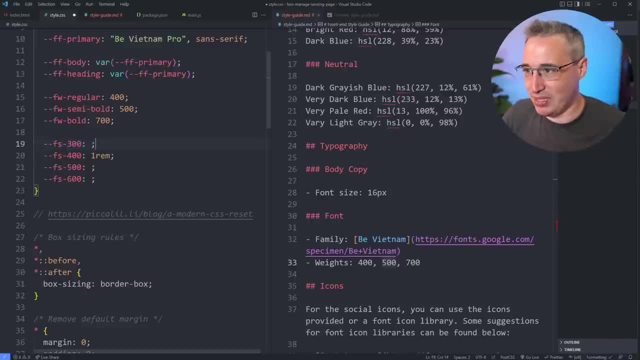 600.. um, and yeah, 13 pixels is really tiny, so I almost feel like just ditching it, but we'll stick with the design as closely as we can. um, but yeah, if I was working with someone and I just had to match the design, I would just match the design, which I'll do in this case. but if I was working, 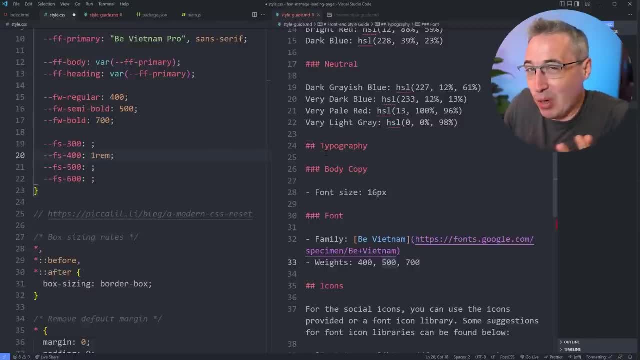 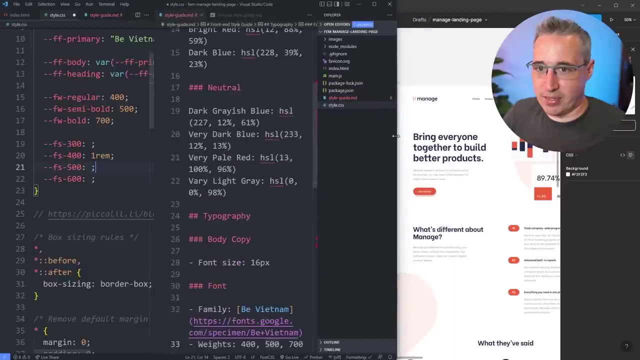 with the designer and I had an open communication with them. I would be like, well, can we actually find a way to make that 16 pixels, and could we make that work? because there is we we do want to. there's a very good reason to, um, so let's shrink this down a little bit and just see. that's it, 56.. 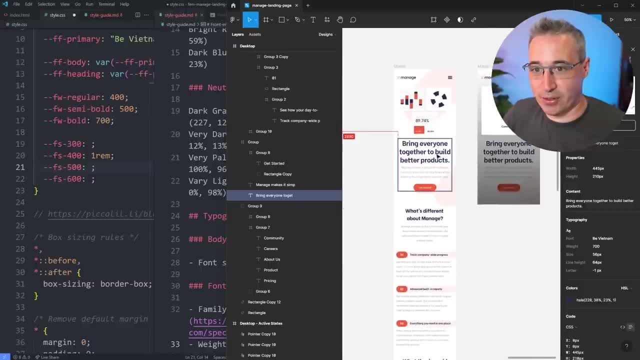 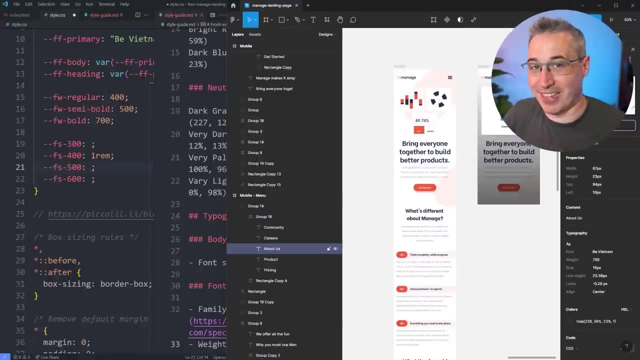 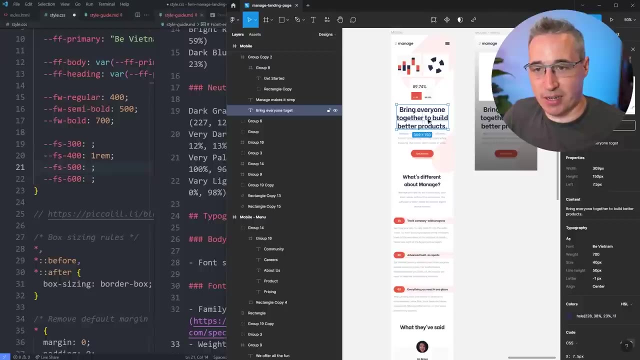 oh, uh, what we're actually going to do. let's go look at the mobile sizes first, because these, that's a 40.. that's at 16.. oh, look at this, the Navigation's bold. huh, that's interesting. that's interesting, which is fine. actually it's going to be completely fine, but interesting, uh. so. 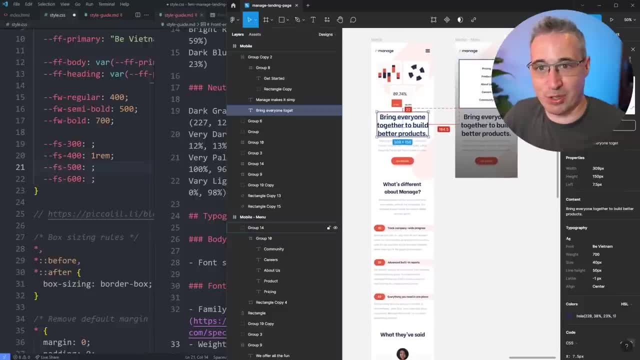 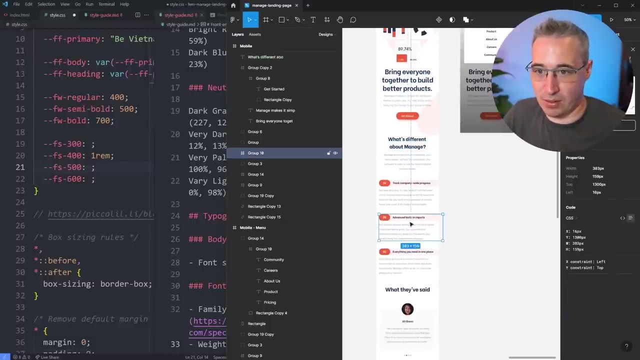 there's a few different ways we could tackle that. actually, we'll talk more about, like abstracting our custom properties when we cross that bridge, um, but here we have. so that's at 40.. so 40. that's probably the biggest font size. right, we have that one. this one's at 30.. these are also 16, or no those. 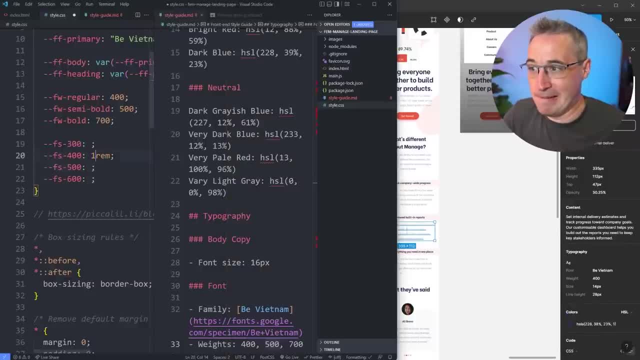 are also 16 and that's: oh, these are down to 14.. so there's something. if this was, I'm going to leave it at 16, actually just for my body text. uh or no, we're, I'm not going to. um, I keep saying it. we're going to follow the design and try and match it, though I will make. 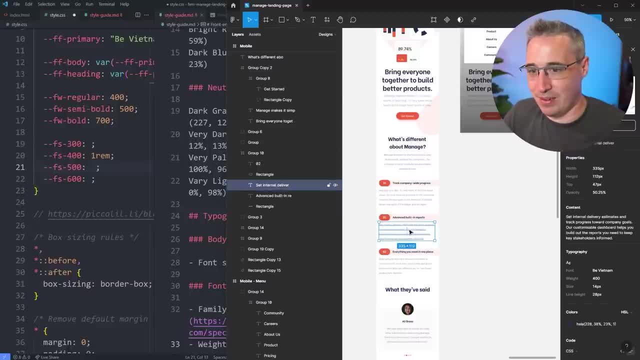 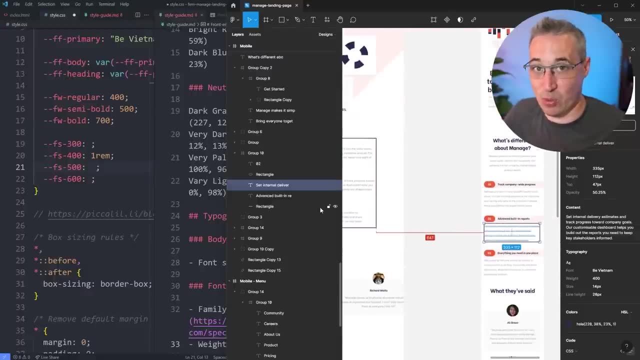 a few small changes. if the yeah, 14 small, this to me should be like a 16, and then at the larger size, maybe up to an 18.. um, if you do want to have that font size difference, but that does mean here, uh, 14.. 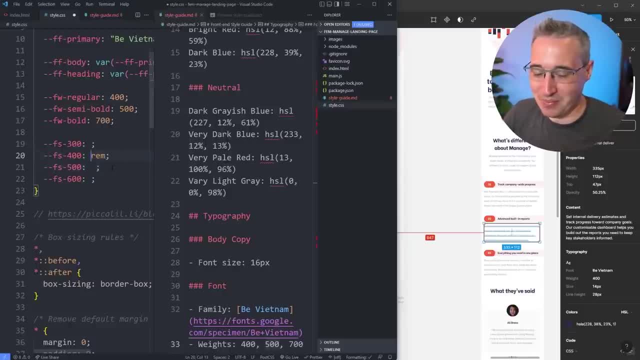 I don't usually go smaller than one rem um, so I don't know what 14 is. it's probably in the point seven. I think it's bigger than seven five. let me open my calculator and, yeah, so it's a point eight seven five um. as we can see. 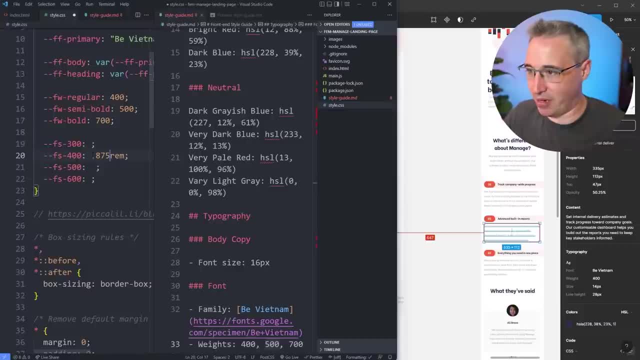 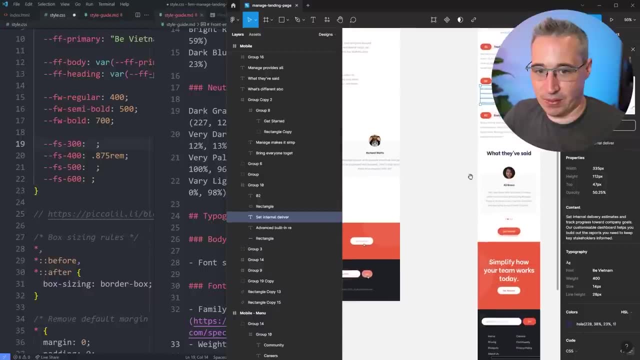 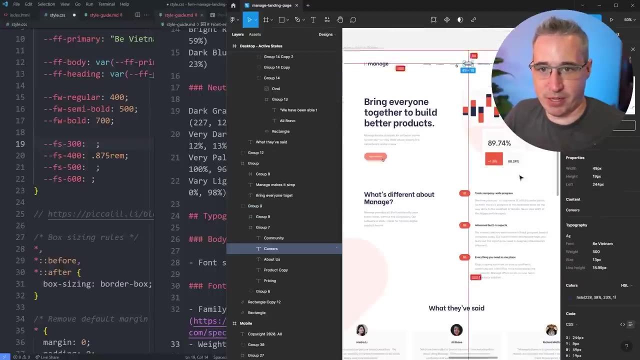 right there, so we'll do that. uh, point point eight, seven, five rem, my 300 would probably stay at 13 pixels. um, I don't remember what we had that was at my navigation was the one that was at 13, right? yeah, sorry, I couldn't find it. I couldn't remember what it was and here is it small. it's at 16 here. 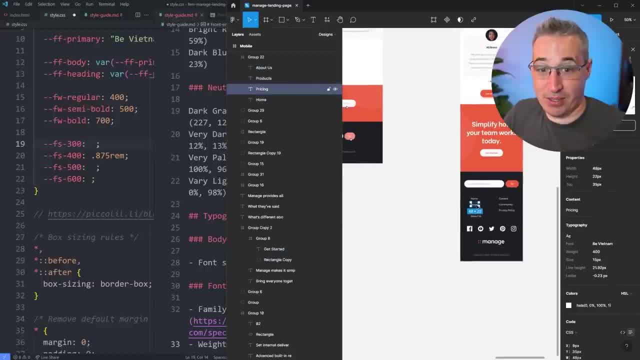 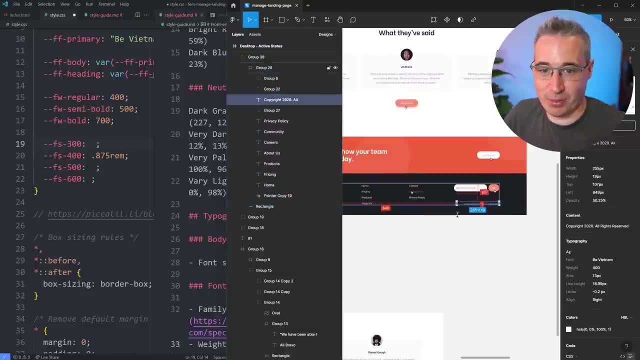 um, there's a few things that are going to be kind of annoying here. these are at 15.. what are they over here? so there are a little bit of inconsistencies, and again this is when the older front-end mentor projects. I did notice this a bit more. in the newer ones they tend to be a bit more. 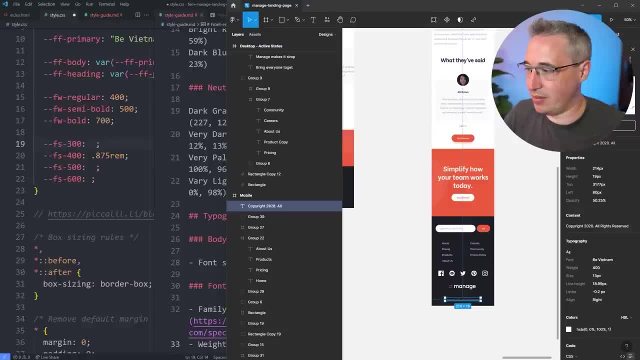 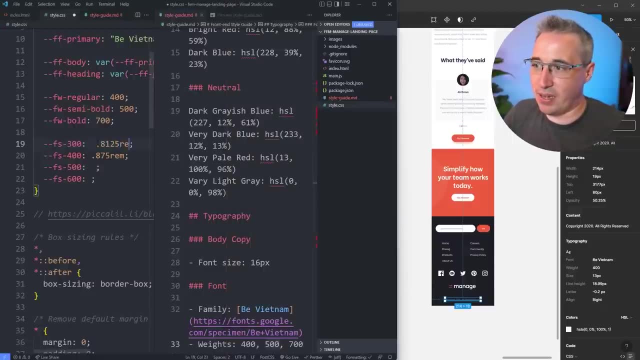 consistent 13 and 13.. um, so 13 divided by 16 is 0.8125, uh, 8125. the reason that I'm actually this is if we want to set it up with like a very simple system here, normally, like you can correlate like: 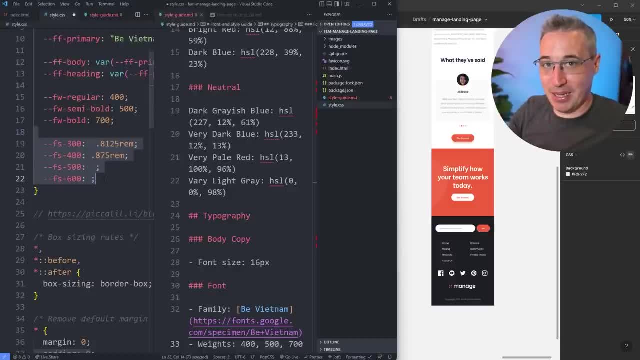 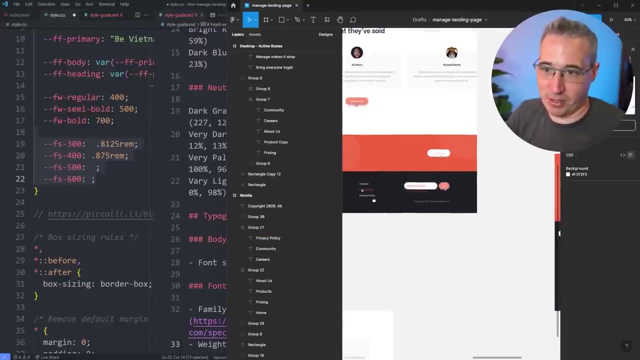 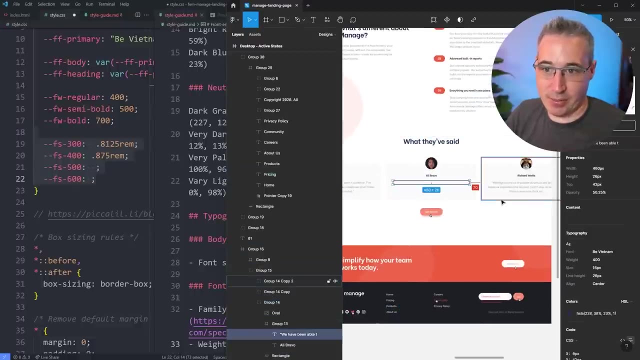 this font size becomes this one, and there's a very easy link to make in this case, where the fonts are very like a 16, or we have like these, with our at 15, and actually I think they're 15 and 15 probably. um, so those stay the same, but like here, we have a 16. here that's becoming whoops, 16 of my body text. 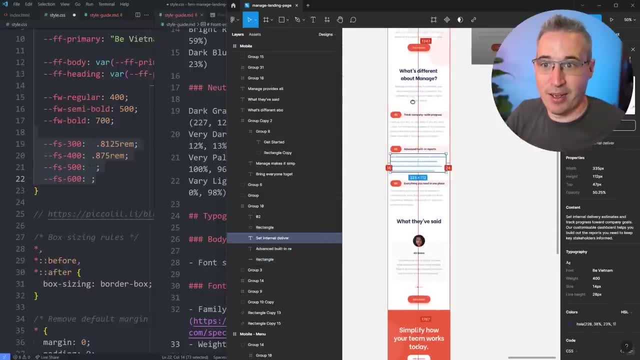 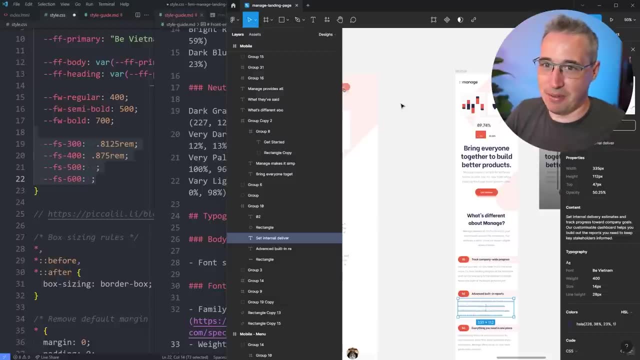 is a 16 and the 16 there is becoming a 14.. um, I have a 13 here which is actually getting bigger like, but then some of the 13s are staying 13.. um, it makes it a little bit harder to play around with a little bit with a simple system in. 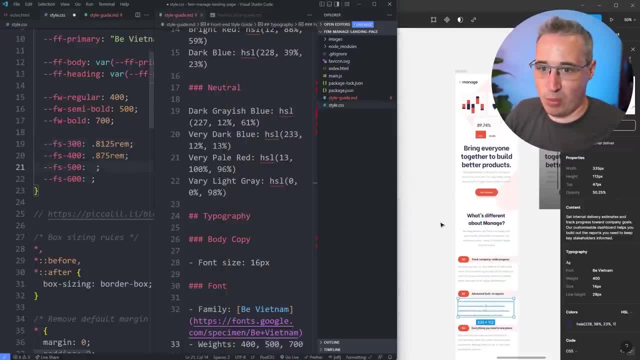 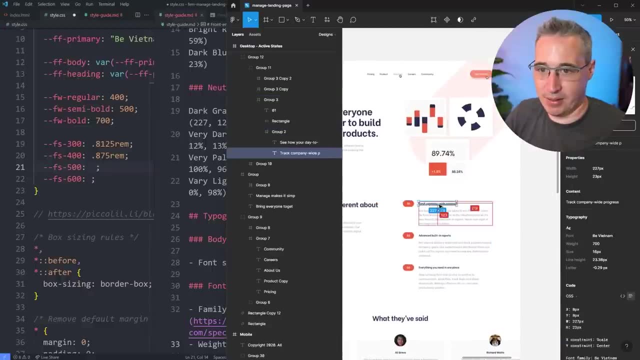 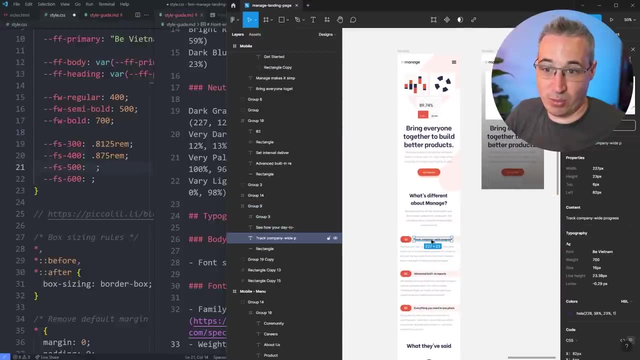 place here. but that's fine, we can work around that, it's not a problem. I think what we'll do. this one was what. this one's 16 here and is also 16 here. so see, like here it's 16 and 16, and then at this screen size, we're running into it. 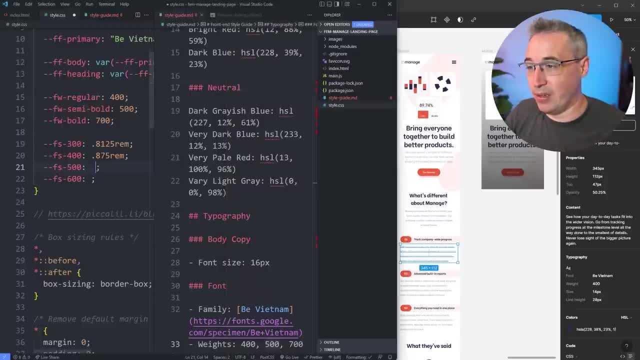 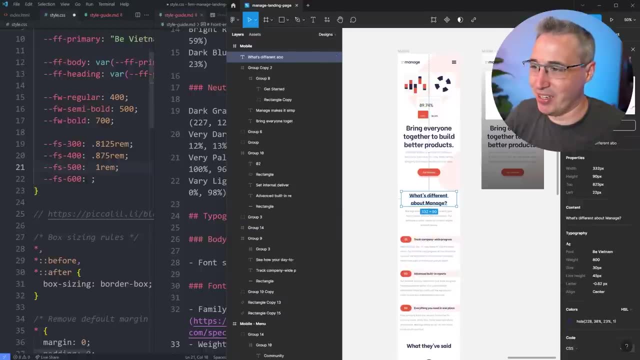 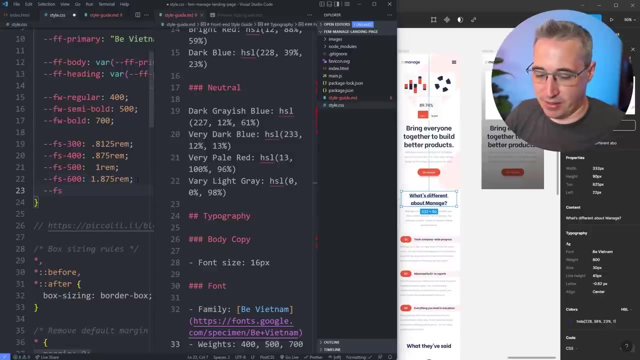 where it's a 16 here and a 14 here, so that does make things a lot harder. this is 30.. 32 is two rem, so that'd be 1.875, and then the font size, 700, which will be my biggest one for this one. uh, is this guy here which is a 40? 40, I believe is. 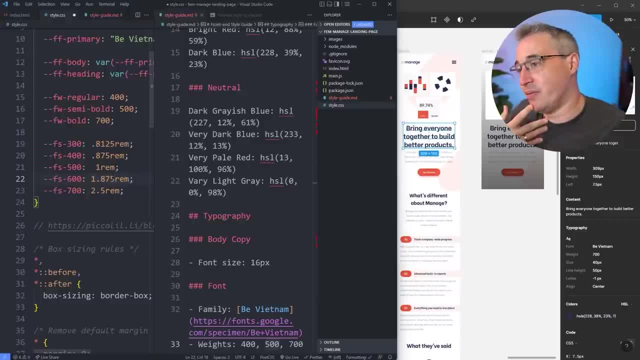 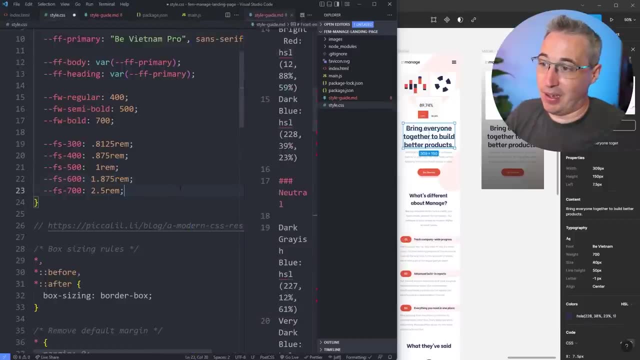 a 2.5 rem um. so I mean, one option here is to abstract things more than I've actually planned on doing, because we could point all of these. then these are sort of the different sizes being used at mobile, but then we have a different group of sizes at a different screen size. 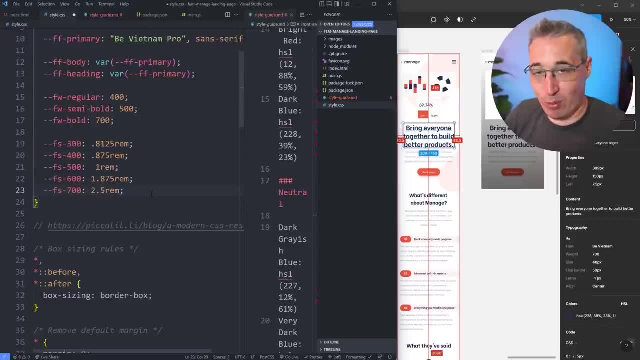 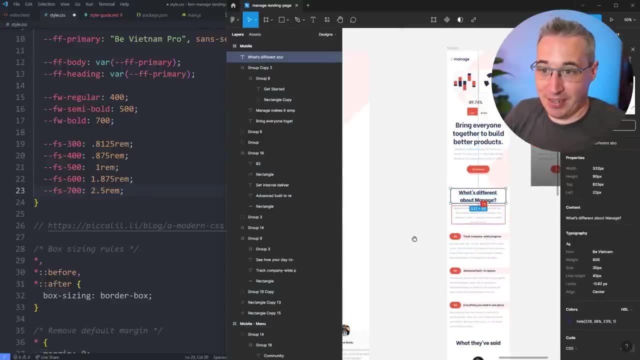 um, because normally what I like to do is: this is my base, and then we throw a media query in and then we just change those base sizes and everything correlates really nicely. this is leaving me having to think a little bit more on how we're going to approach that. 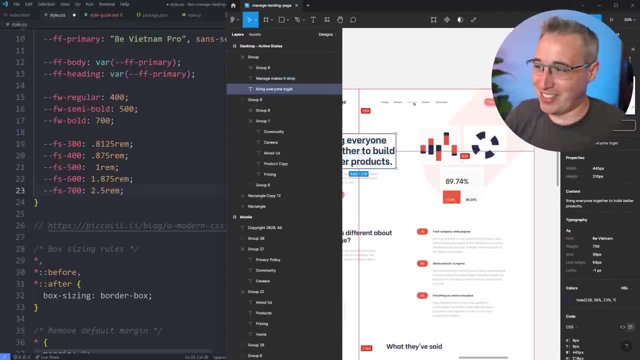 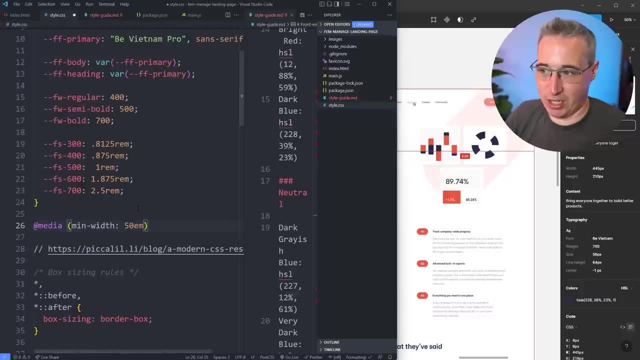 um, let's start with the easy ones, because the 700's very easy. so let's throw our media query here. at media min width, we'll say 50m. this number we can change, but that's what we're going to stick with now because it's easy to remember and root. so my font size is going to: 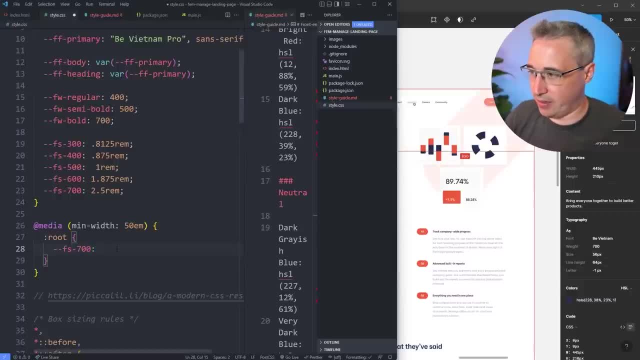 become uh 56. 56 is I don't know. so uh, just do this off screen. we have uh 56 divided by 16.. is this bindable? that's pretty neat. if you notice it's a nocam: first batch plus another batch, first batch plus another batch, plus you take two or three, that's plus minus two, and then las flies and that's minus two. then someone had this: that's minus 4 squared, or whatever. let me try this one as well. that this one was called 50mm. this number we can change. 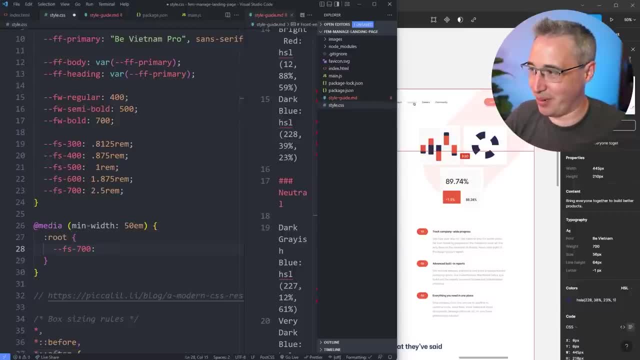 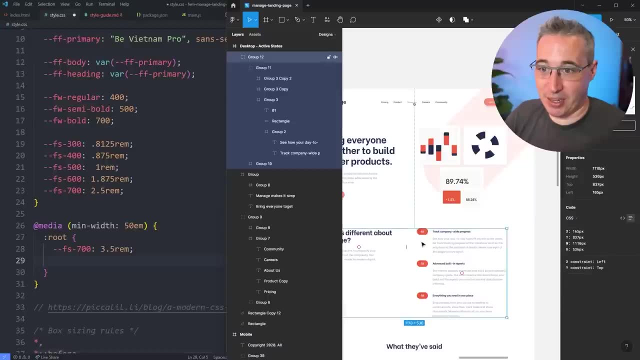 just do this off screen. we have 56 divided by 16 is a 3.5, 3.5, 3.5 RAM. I believe the other consistent one is this one, because that one's there also, which is my 40 pixels, which is going. 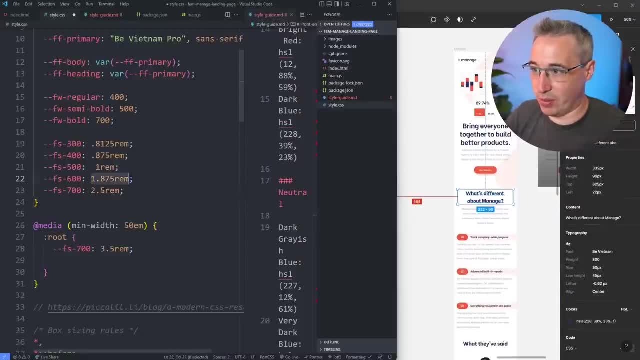 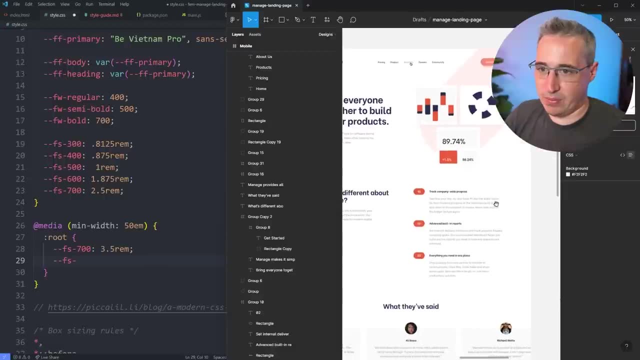 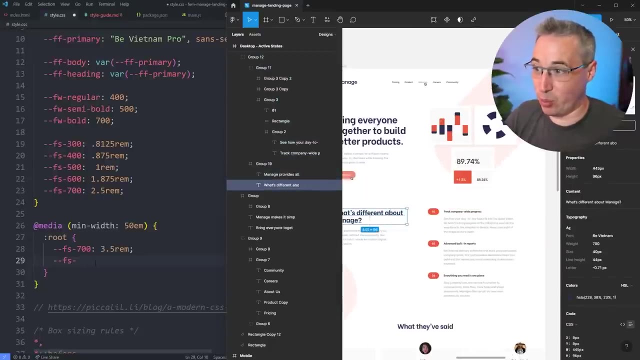 down to 30,. 30, we already know, is this one. so my oh wait, does 600 not change? we have wait what? oh sorry. yeah, Kevin, we're going up now. this is going up to a 40 pixels, so we're. 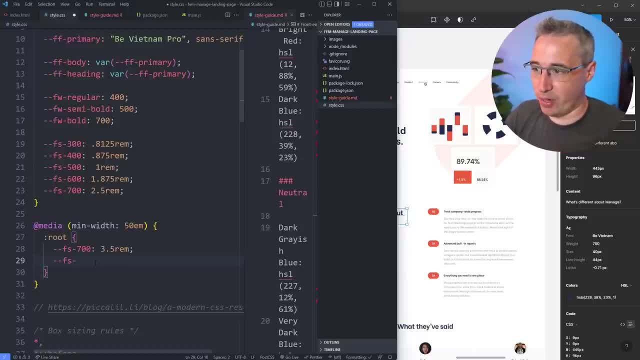 going from 1.875, 40 would be 2,. so 600 becomes 2, RAM or no, it can't be 2, because 2 would be 32, 2.5,. there we go, which we know because we had that here, because that was the size here. 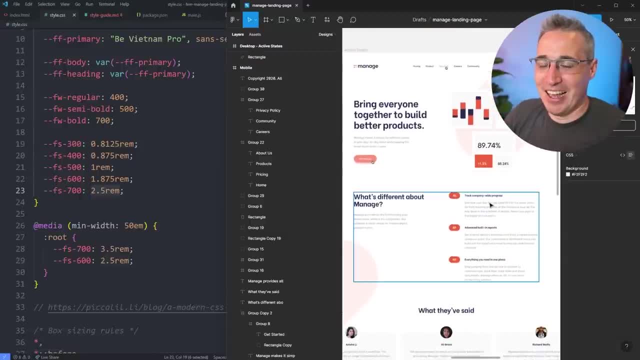 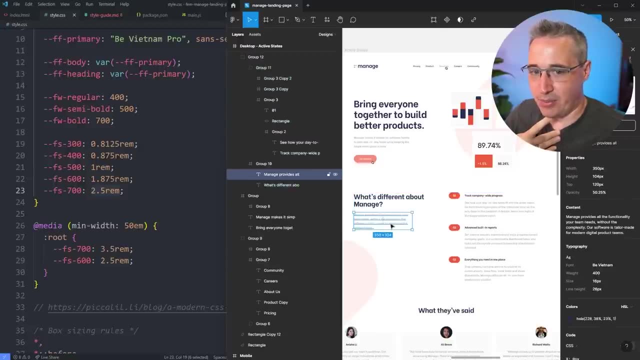 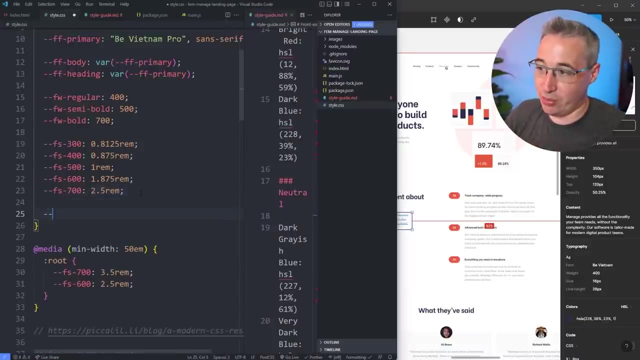 that was at 40, perfect, okay, so I know that's 2.5, the ones that are more complicated are my body, which is 16, into 14, so I mean, what we could do here is I could do. there's different ways to do this. 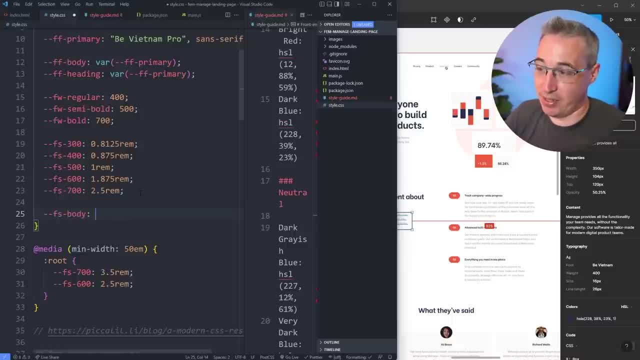 honestly so you wouldn't have to. but I could say: font size body is: here is actually my var font size 400, which is looking at that one, and then here we could say that my font size body is becoming var font size 500,. 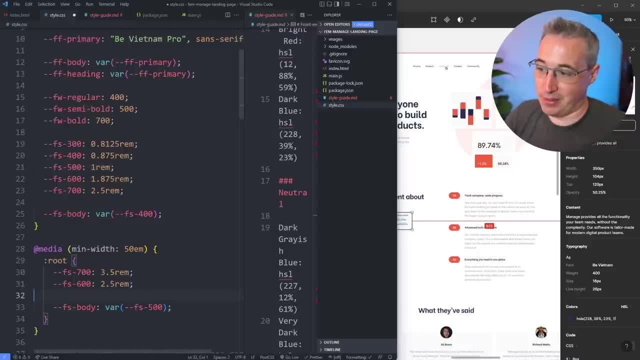 so then it goes up to the 16, so that is an approach I could take and this is what I said. I usually do more with Sass, where I have sort of this set locked in thing, even though we have media queries, and it wouldn't be exactly how I would do it, but maybe we do that and then we 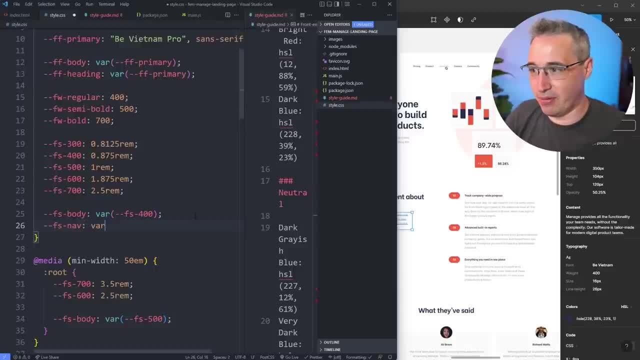 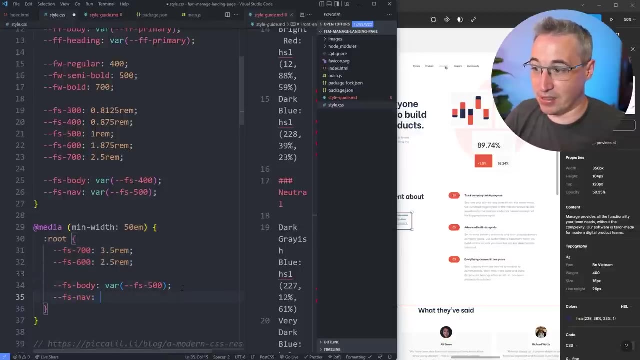 could have like a font size. nav is my var font size. in this case it was the 300,. no, it wasn't, it was my 500,. small screens and then at big screens my font size nav gets smaller, so it becomes my font size. 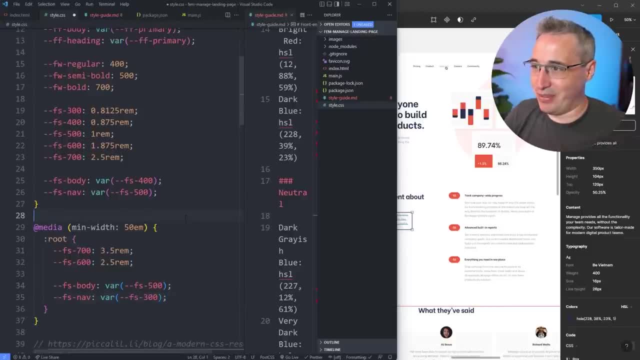 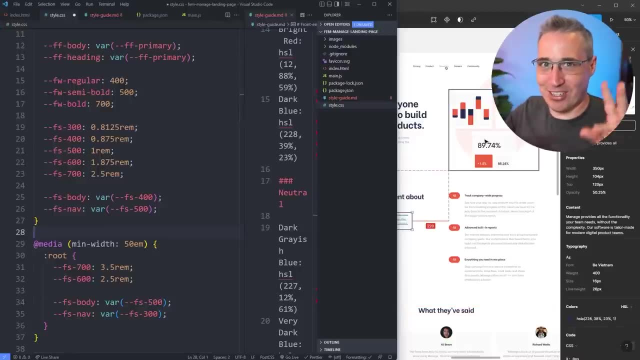 300,. yeah, we were going beginner friendly at this point. you may be going, Kevin, this seems like a little bit much, but it's worth setting things up and doing all of this and not just starting to style the page one thing after the other and hopefully you see why once we actually 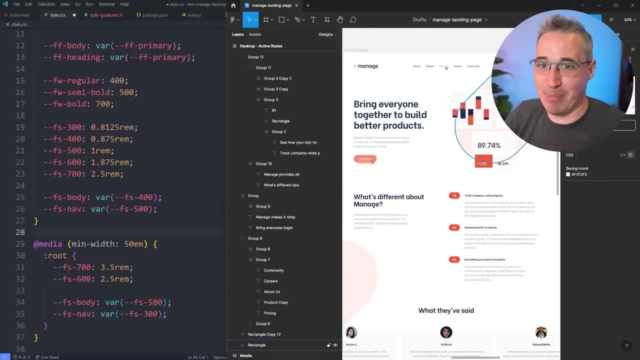 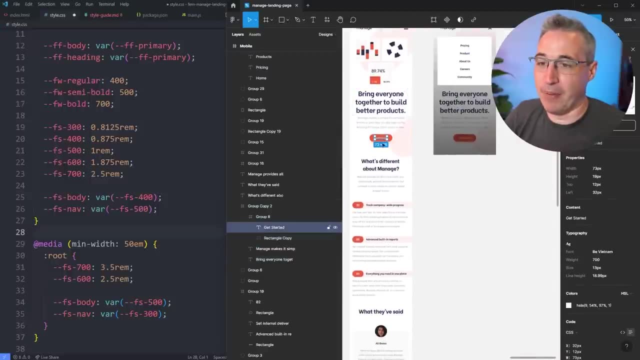 dive in and start making all of this actually happen. my buttons as well are a 13, and they probably stay 13,. yeah, so buttons are always 13,. so we could even do that. we could say my font size button is: 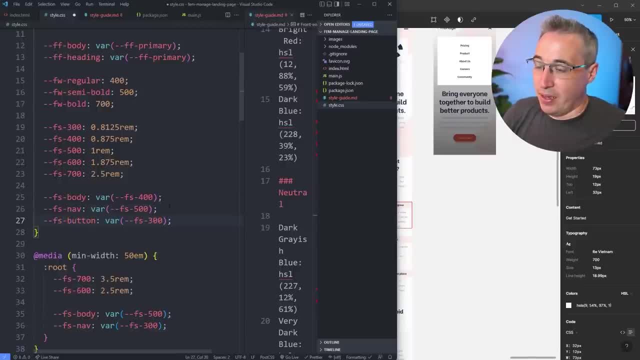 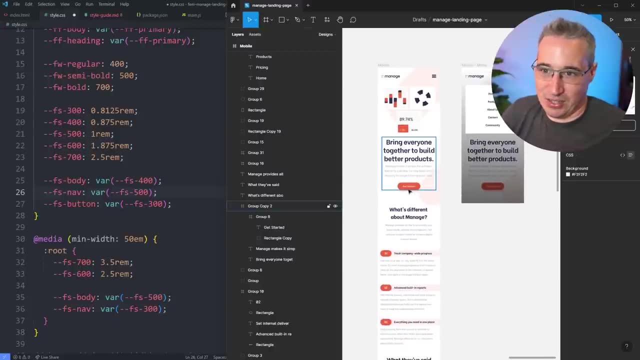 var font size 300, and it never changes. so then we don't change that within a media query. I think this is the right way to do this, just oh, this is annoying. we have a 16 here. I just assumed. 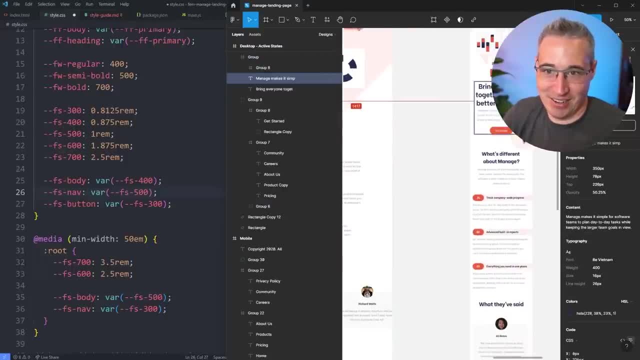 like: this is 16, and then it stays 16 here, but all this one also. no, this one shrinks. this is the only one that's staying, and then it stays 16 here, and then it stays 16 here, and then it stays 16 here. 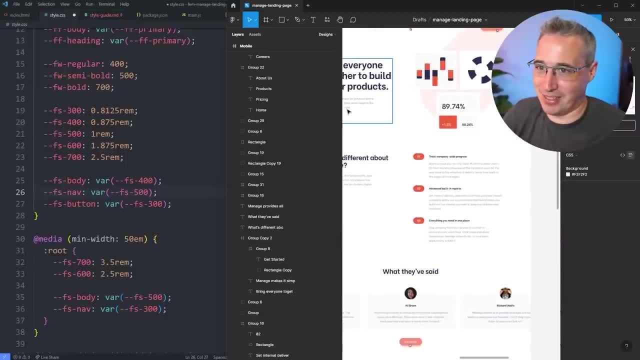 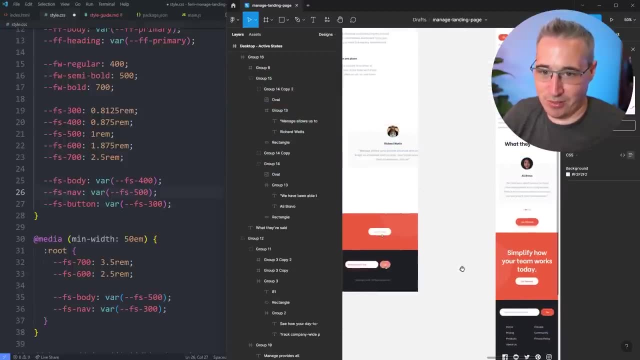 and then it stays that that one. we're going to shrink all of them for consistency. 16 is going to become 16, my testimonials are the 14,. here they're a 16, good, I think. oh, we have these. 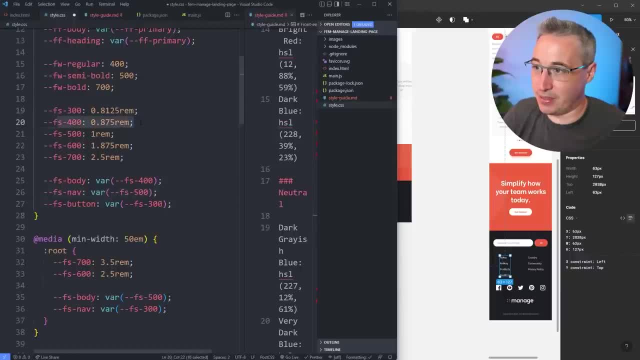 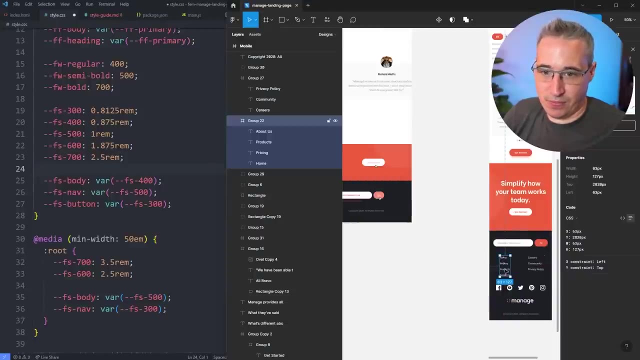 ones down here, which are my 15, the 15 pixels is this one? oh, we didn't create one, so I mean, this is why I like this numbering system actually, so I could decide that my, because these, these are 15, right, these are 15 here and they're 15 here. 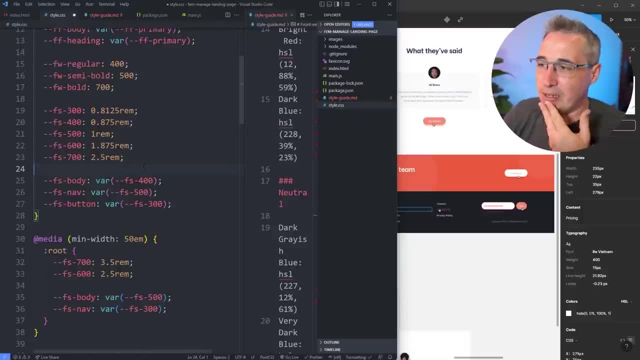 yeah. so this is where I'm actually going to change how I'm doing this. here too, actually here, let's do it now before I get to the 15, font size: 900 is going to be a 3.5 rem. I'm going to. 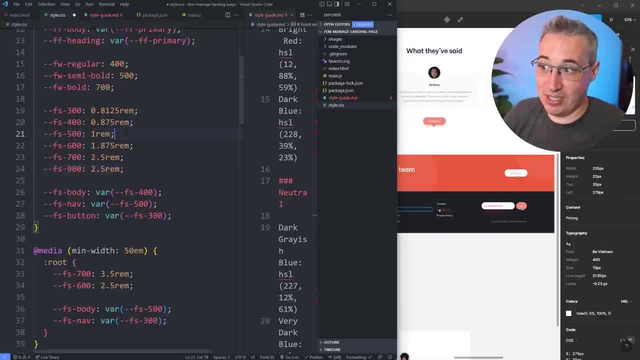 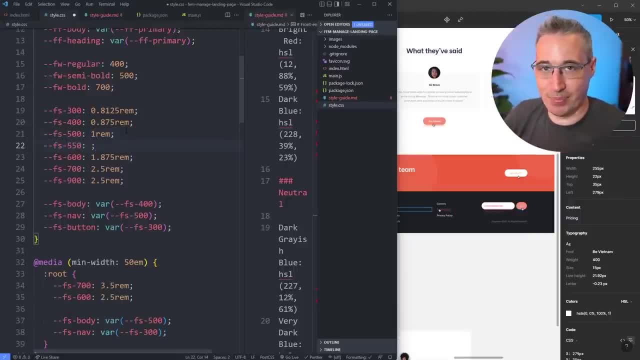 and then I need a new one. I can do a font size 550, and squeeze something in between. so, instead of a 5 and a 6, this makes it easy to add new things in, because we haven't actually started applying these styles anywhere- I'm going to make this an 800,. 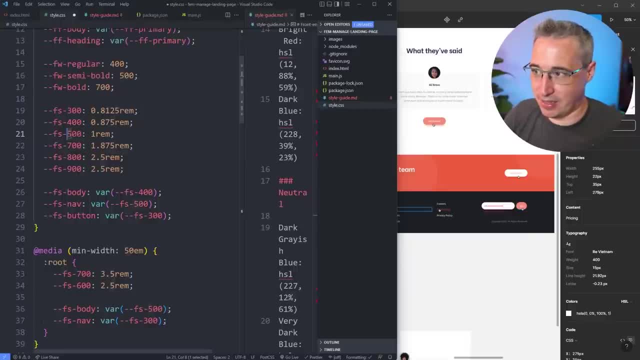 this one's a 700,. this one's a 6,. no, that one's 5,. yeah, this will be a 600, which is crazy for one rem, but it's, it is what it is. font size: 500. 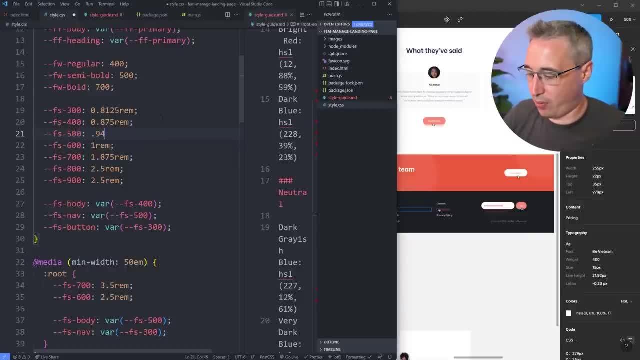 can be 0.95, 375,, which is 15, cool. so yeah, I mean having this in this. it's kind of. anyway, it is what it is, that's fine, and, as I said, we're going to change this a little bit. so here I have my 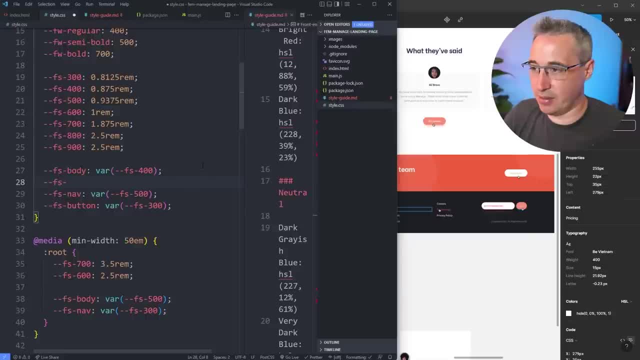 body, my nav, my button. here we're going to do font size. primary heading: var. font size is 800 by default, or at the small screen sizes, and then at larger screen sizes this becomes the 900, the only reason I'm doing this instead of using this, so we can delete this right away. 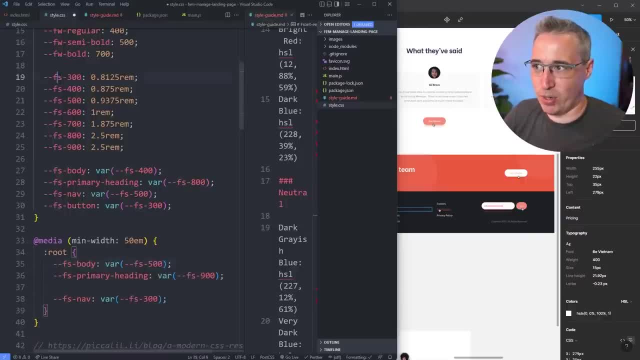 is just so it's more consistent. like it's kind of weird to have some of these changing and then sometimes these changing. I'd rather like here's all the font sizes being used and I'm only changing these within media queries. I think that makes a little bit more sense. 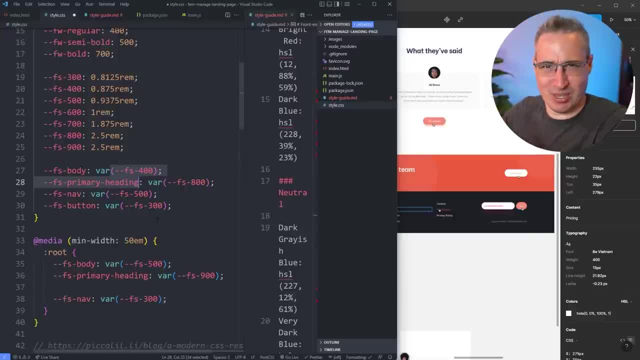 and it's just easier to track than like. sometimes it's a number switching, which is like my base style, but sometimes it's these other things. so, yeah, just a little bit more consistency on that. So that's my font size primary heading and this will be my font size secondary heading. 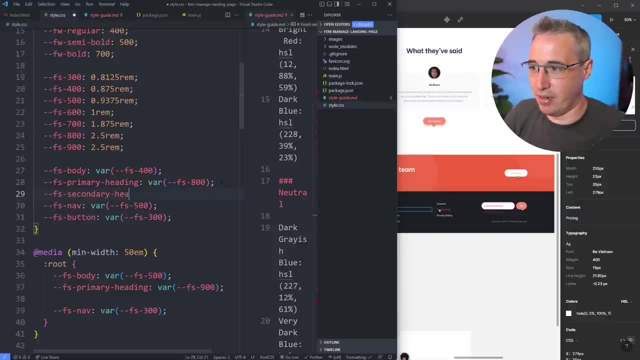 or subheading: secondary heading. secondary heading: var. font size 700, which here becomes: let's just duplicate. let's just duplicate that line. this is my secondary, and then this one becomes my 800,. except that's wrong. no, this is a three. 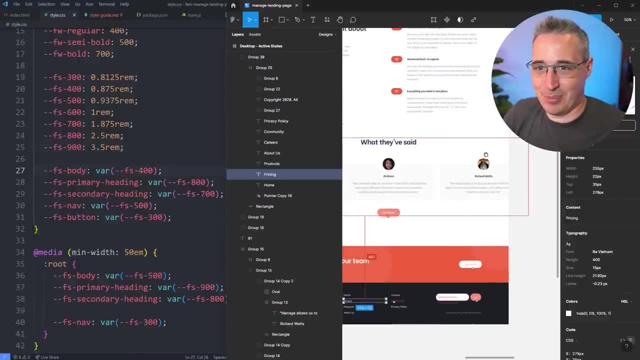 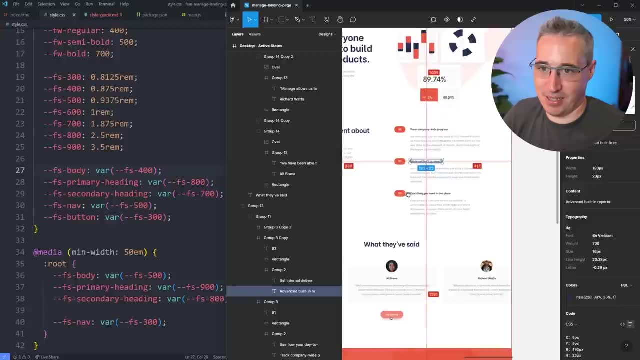 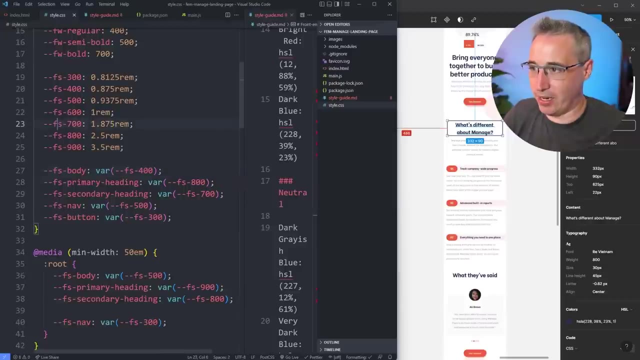 I think that's right. Let's just double check that. This also, this is my like H3, basically that stays at 16, and I think stays 16 here. Yeah, this one is 30.. Yeah, yeah, okay. so that's the 700, perfect, okay. 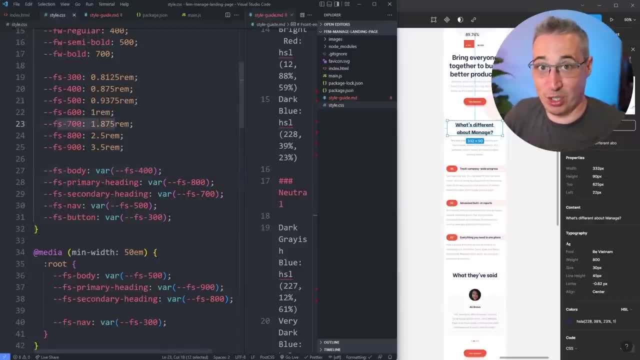 And the reason I know it's this number is: I know that 2rem is 32, so I'm just like, well, it's slightly smaller than 2rem because it's 30, yes, So yeah, that's just how I did that. 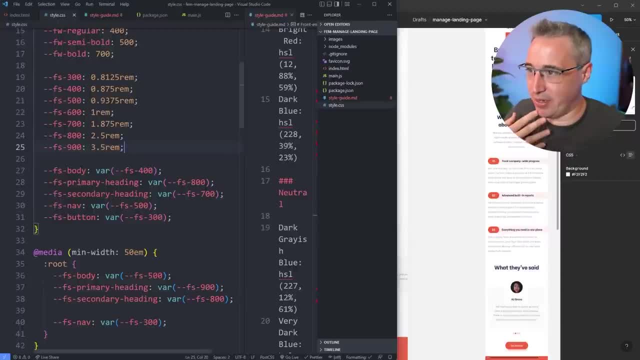 Quickly, Is there something else here I need to put in my body which is changing? Those are okay. It's still a little bit weird how I have this set up, because sometimes I'm going to point to things that are over here and other times I'm going to point to things that are here. 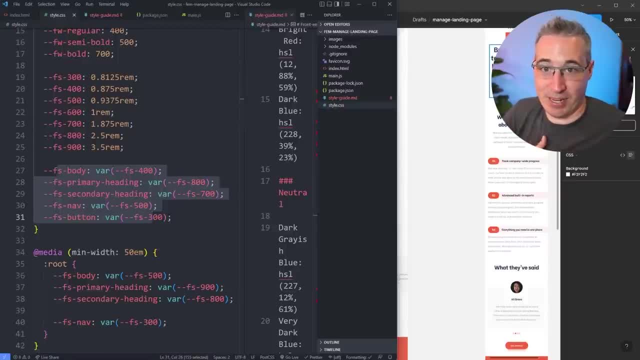 and I'm just wondering because this? I said that I was going to like forget about him, but maybe What we're going to do is- This is also where I usually like having font sizes that are like utility classes, that. 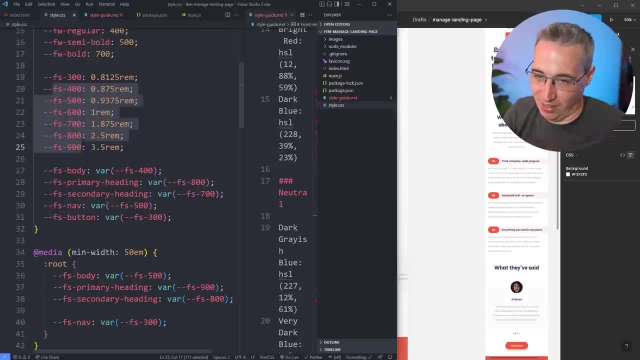 are based on this, which I'm not really going to be able to do with this setup, which is okay. It's not the end of the world. This is not exactly how I usually work, which makes it more interesting for a video, because 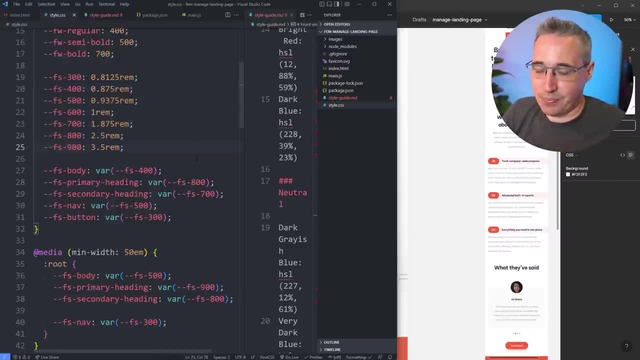 I'm really having to think about how we're setting all of this up. So that stays there. So maybe we have primary heading, secondary heading, and then we can just do a Font size, fixed font size, like we have body, which will change a little bit, and 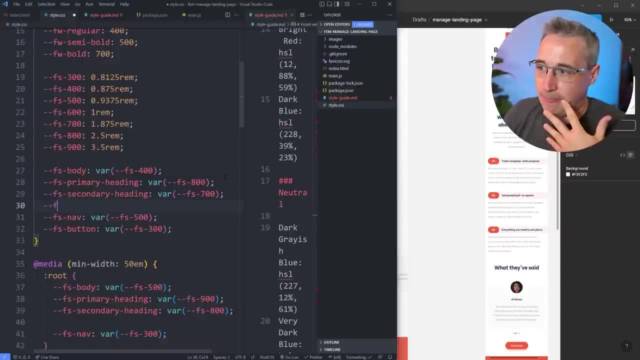 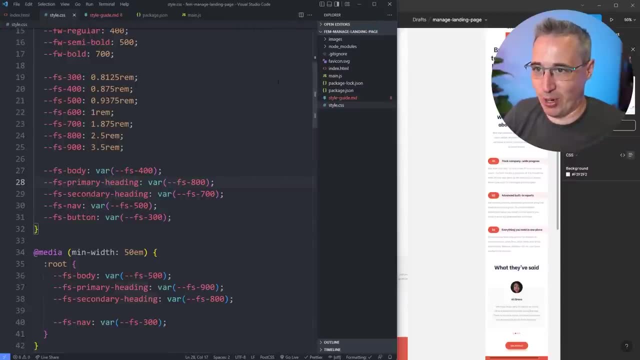 that's fine. Maybe we don't need. I'll leave it like this because we don't need to switch it. We're going to leave it like this. We'll see if we change my mind along the way. But yeah, that's going to set up like that nicely, I think. 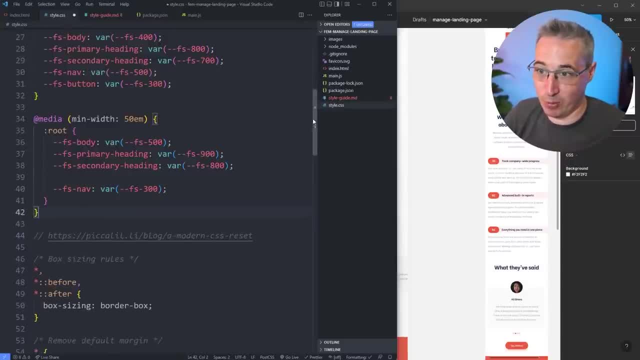 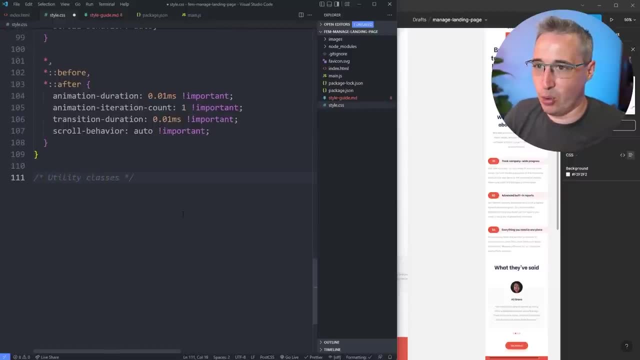 And then we can create those utility classes. So for these I'm going to go below my reset. We can come all the way down here and let's put this in Utility- Utility Classes, Which are all going to be based on that. 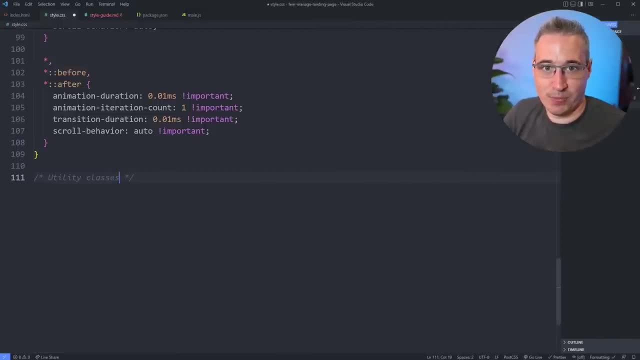 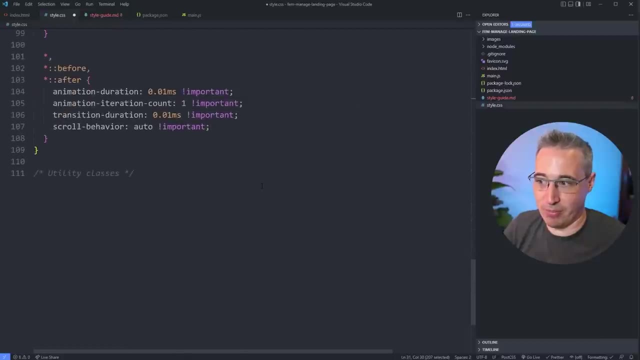 Now what's annoying- if ever you are setting this up we can go full screen- is if ever you have a single file like this and you're going up and down to like look at these and look at what you're doing at the bottom, you can just right-click on your CSS file. 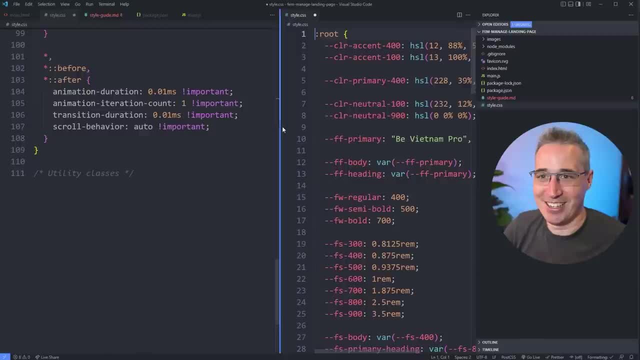 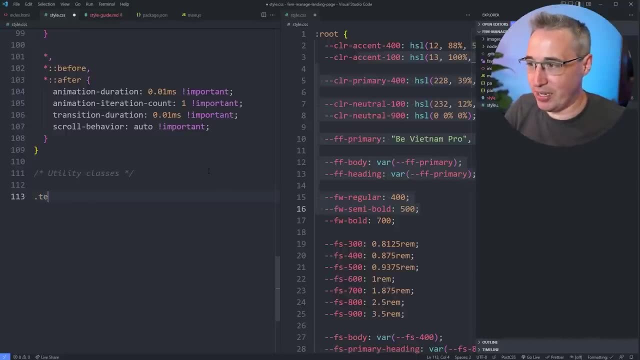 again and open to the side. You can have the same file open twice, So this one can stay at the top and then this one down here makes it a little bit easier to set these things up, So I'm going to do a text color for all of these. 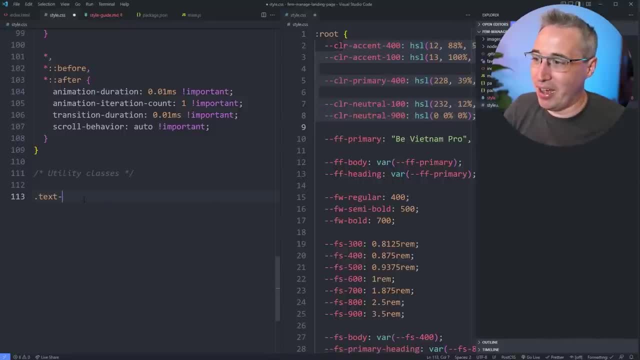 I don't even know. I don't know if we really need that, but I'm going to set it up anyway. So text: primary 400.. And then here we can do a color of my var color: primary 400.. You might say, like Kevin, do we really need to do this to make the utility class? 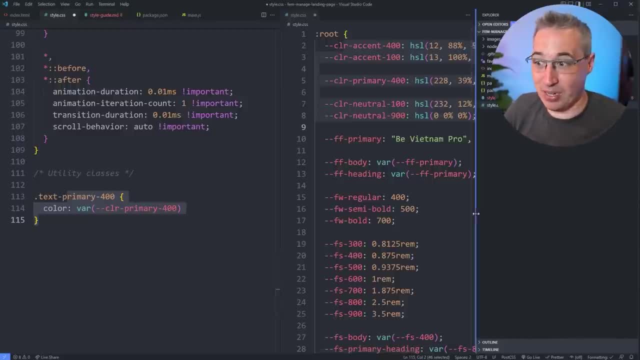 Hopefully, once we get into the project itself, you see that there is value in doing this type of thing. So I'm actually going to go through pretty quickly and set all of this up, and then I'll see you on the other side. 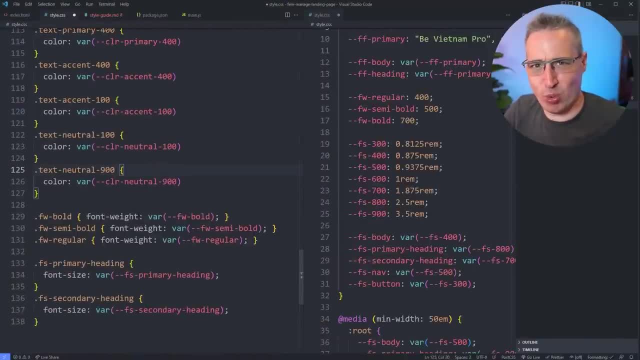 All right. So I've set some stuff up here. I haven't finished everything, But I just want to show you One way that you can work a little faster when you're setting these up. So you can see, here I've done all of my colors. 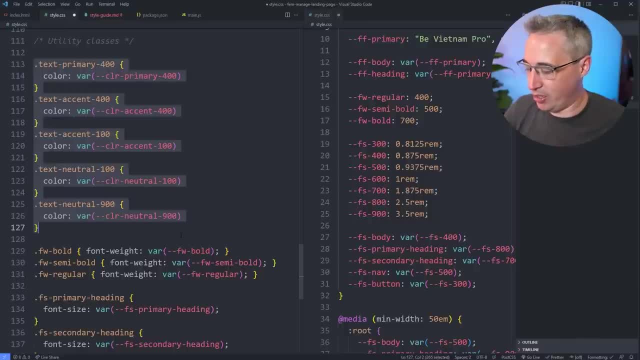 So what I'm actually going to do is select all of that and then I can do a shift, alt and then down on my keyboard, And I think on a Mac it's command shift and down and it's going to duplicate all of that. 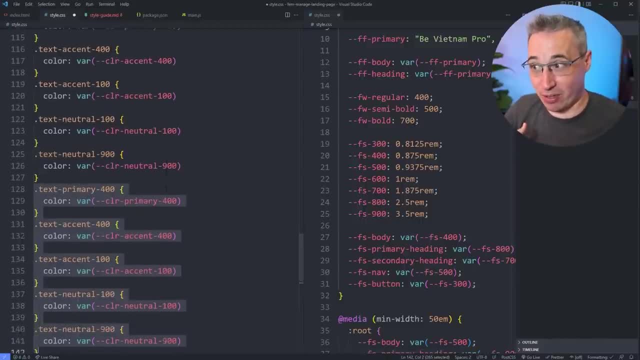 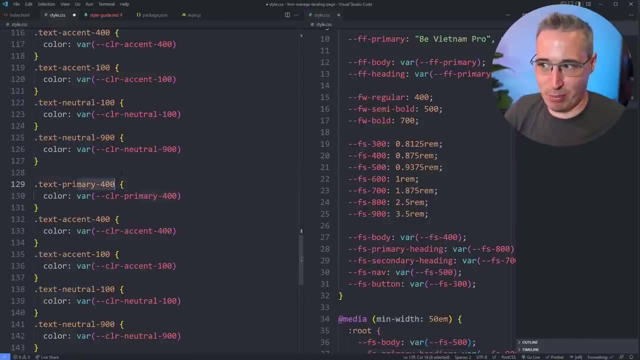 And then because here I've set these up as text colors and now I want to do background colors. So to do that, now I'm going to come here and to select this first one, because this is, you know we've gone from. I can see this is my primary 400, where I started at. 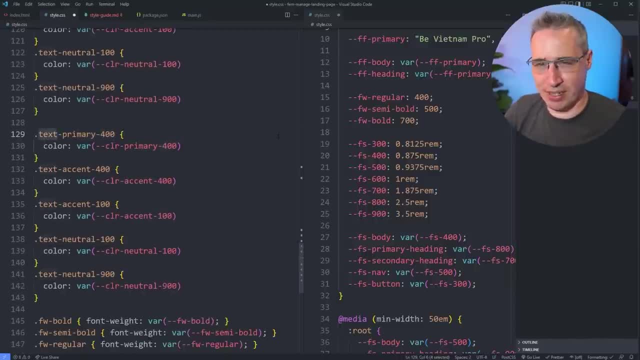 So these I don't Want to be text anymore, so I'm just going to push control D again, command D on a Mac, and then I can go through and multi line, select that and turn that into BG primary And then on all of these where it's color same thing, select them all, push my arrow key to the side and then right back around color. 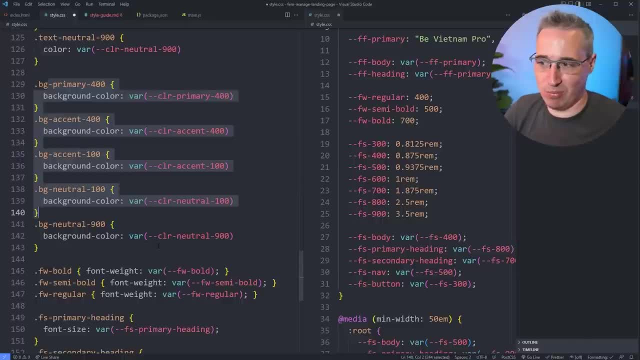 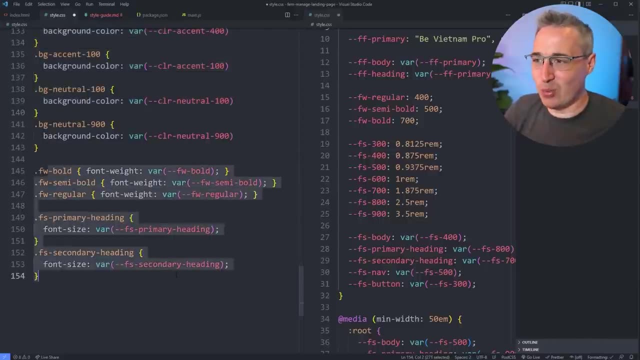 And then so these now just become background classes And so you can work a lot faster by doing stuff like that really fast here on setting up these utility classes. You may be going, Kevin, do we really need these? You have the. you know why are we linking utility classes to variables? just so I can work a little bit faster once we start actually making the site and bringing it all together. 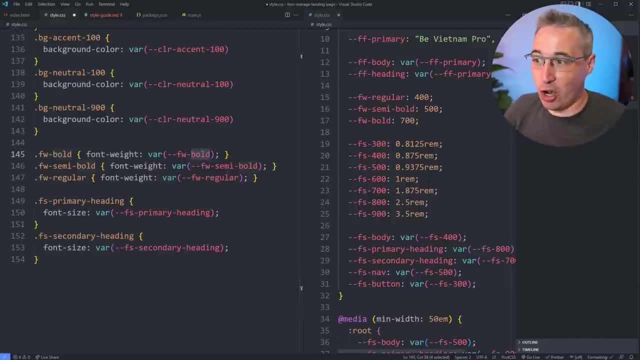 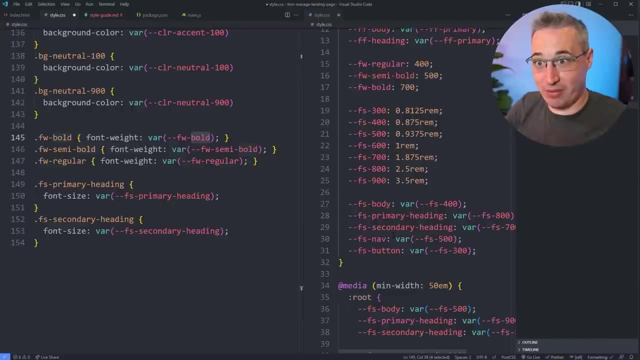 And I didn't finish and I wanted to, you know, actually talk my way through part of this, because this is different from how I usually work, because of this sort of the difference in how I would normally do my font sizes compared to what we have in this project. 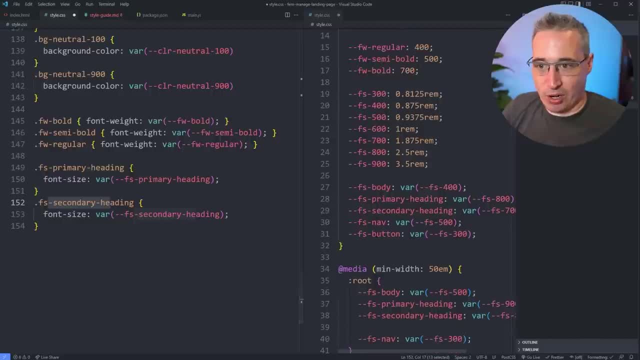 And so I do my font size primary heading, font size secondary heading, which are fine. font size body. I don't need, I'm just going to put that on the body itself. My nav: I'm going to use that when I'm styling my nav, my buttons. 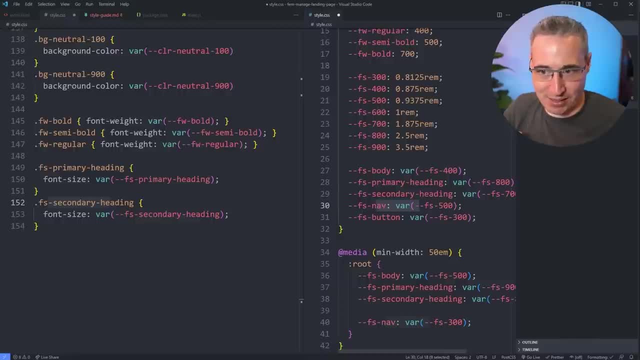 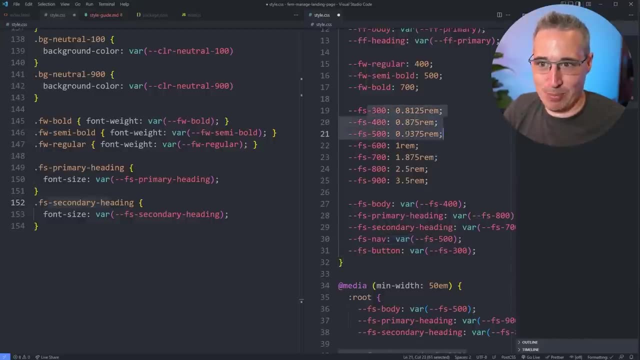 I'm going to use that when I'm styling my buttons. So those, these are like specific things that I can use in specific places. But what's different is I do need these to be used somewhere, right? Because my body is my body's, looking at the 400, but it changes to the. yeah, these ones are changing. 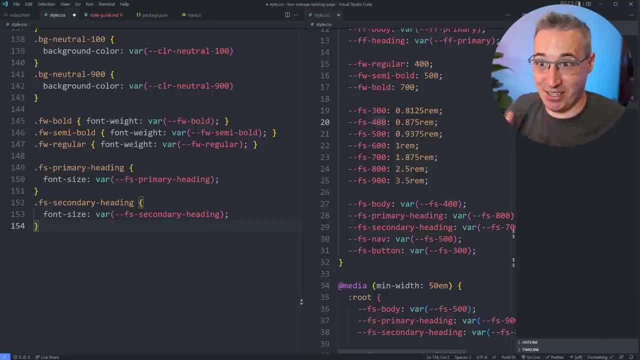 So what I need is, like what happens when I have a 16 that stays a 16, or what happens when I have this like the 13 that stays a 13.. Or things like that. So I think what I'm going to do is a font size X, X, S for extra small, and you can even do extra small if you want it. 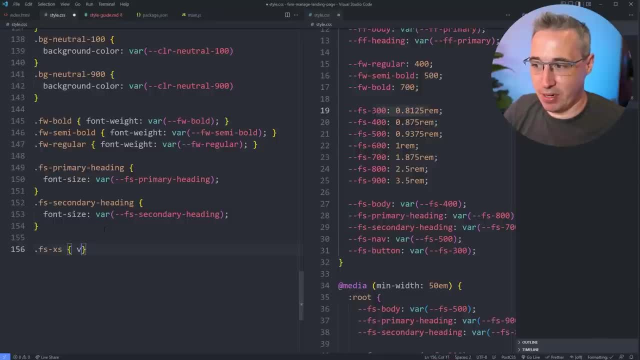 I'm going to do XS for extra small and this will be my font size of our font size 300, and then we can do a font size small Again. I usually don't do it like this. I usually this is my numbering. 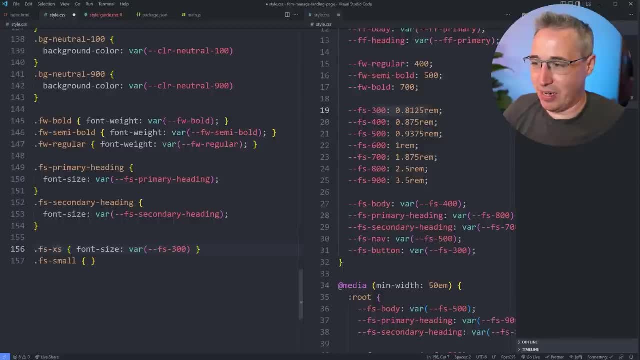 Do I do my numbering here? Okay, let's think I'm going to font size, of our font size, 400, because it's still pretty small. And then this is my 15 pixels, and this is the problem. This is why numbering is nice, because, like I have small, extra small, small and then like kind of small. 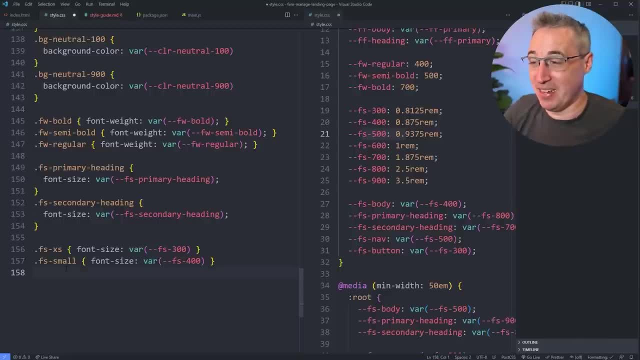 So maybe I just stick with 300, 400, 500. And then it's just: I don't, Yeah, I might do that just because. and then, like say, we did add a 550 at one point, like what name would that get if you had a utility class to go with it? 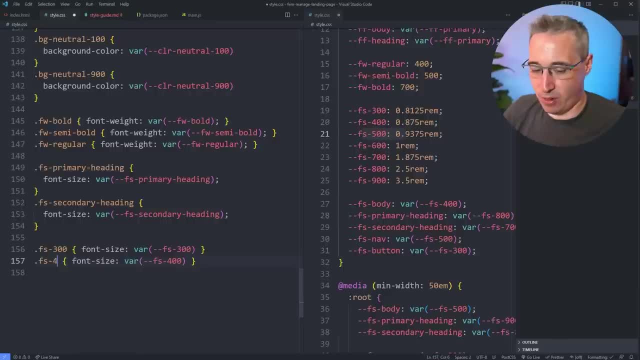 So we're going to do that. We're going to say 300.. 400 and we'll do a 500. So again, you could duplicate the whole line, like I showed you, and then you could select the 400, push command D or control D, and then just change both of those to a 500 at once. 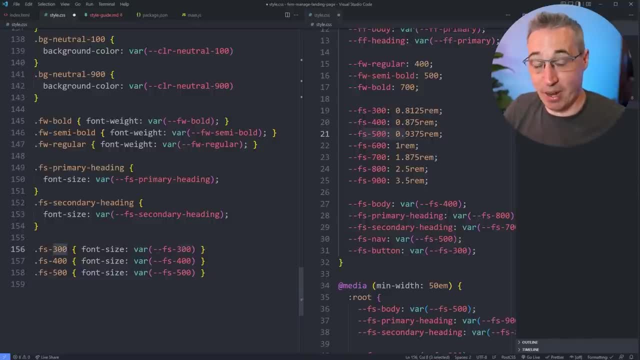 So I just sort of have to know that if something is a number, it's not changing. The media query has no effect on utility classes that are numbered, but it will have an effect on ones that are not numbered. So if something is a FS secondary heading. 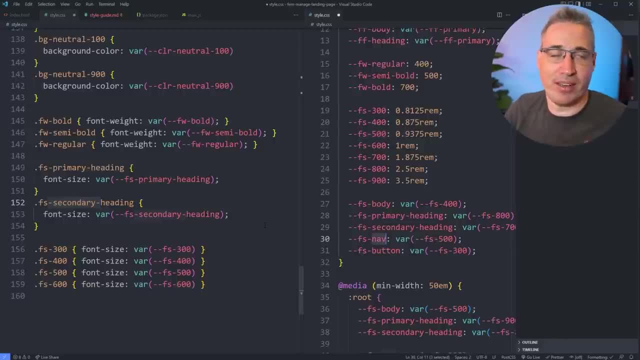 Or if it's my font size, nav or whatever, if I had other ones that I was using in the system. the idea is if it's numbered, it doesn't change ever, And if not, then I have a utility class with a different name and those ones do change. 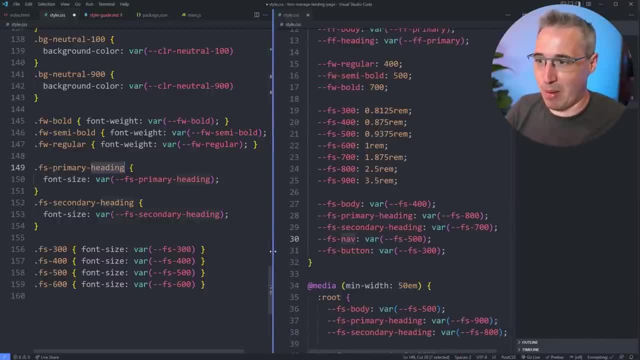 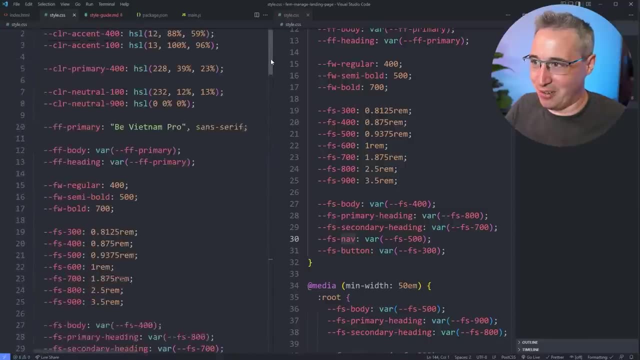 I think that's sort of how I'm going to treat this project And hopefully I remember that while I'm building the rest of it out. So right now we have my colors, Let's hit save on this. We have a whole bunch of utility classes set up, our root system here, I should say. 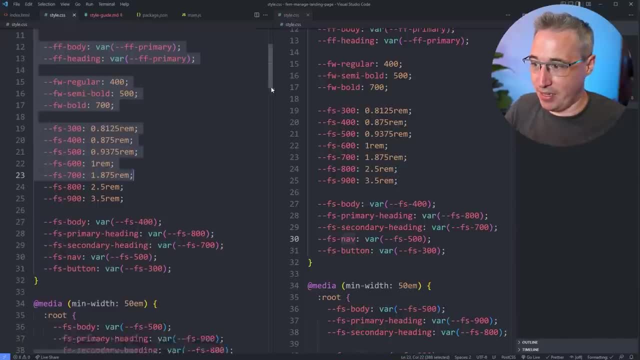 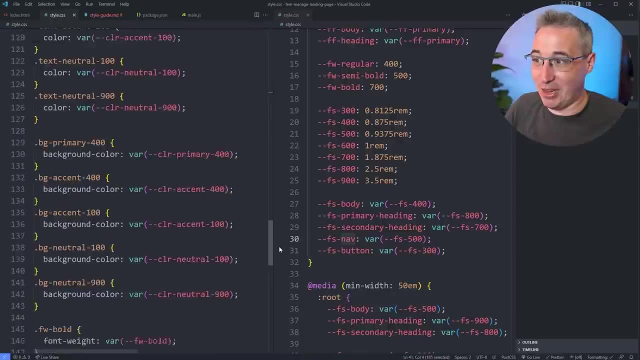 So we have all these custom properties set up. We have a few things that change within my media query, We have a reset. that's just sort of getting us on the right stage. And then we have these utility classes that we can use for things like font sizes, background colors and text colors. 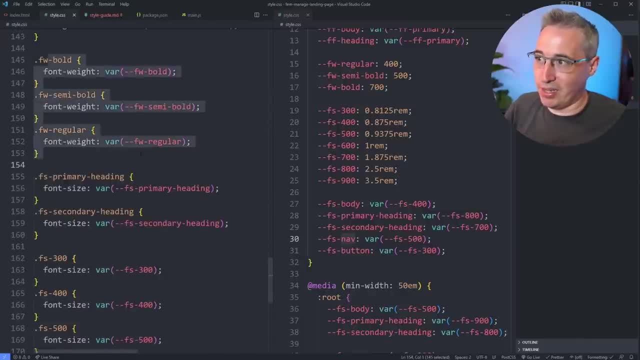 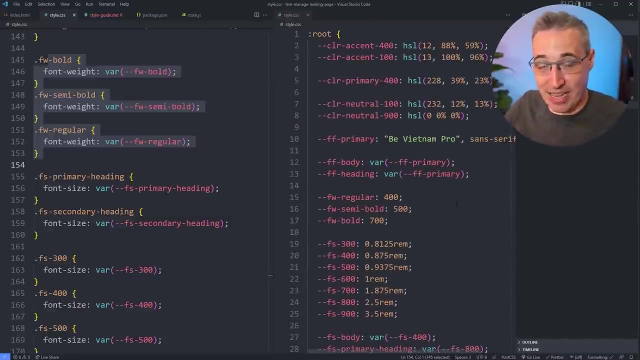 And font weights. I did do some for font weights as well, And I think we're on the right point now to dive in and actually start writing some HTML. I'm hoping I didn't forget anything- I probably did, But I think this is good enough to dive into the HTML and start writing some of that, getting everything to come together. 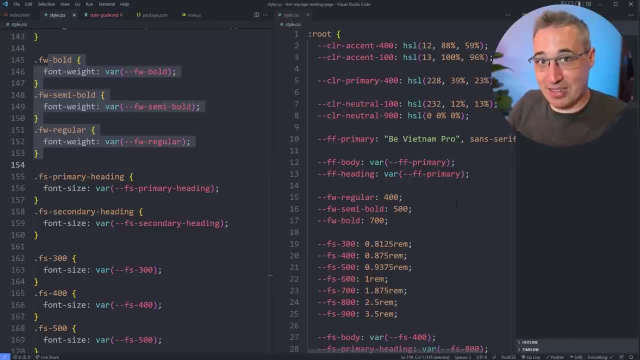 We'll be going back into the CSS, because there's normally a few other classes I would have at this point, for, like my container, I have a flow class that we're going to explain a little bit, But I think what I'm going to do instead of doing those right now is bring them in as we're styling them and using them on the page. 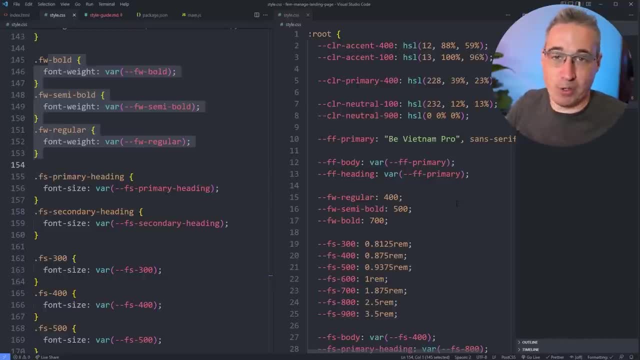 Just because I think it's going to be easier to make that connection on why I'm using those classes instead of making you know. a font size class is obvious what it does, Whereas the flow one it makes a lot more sense once you actually see it in action. 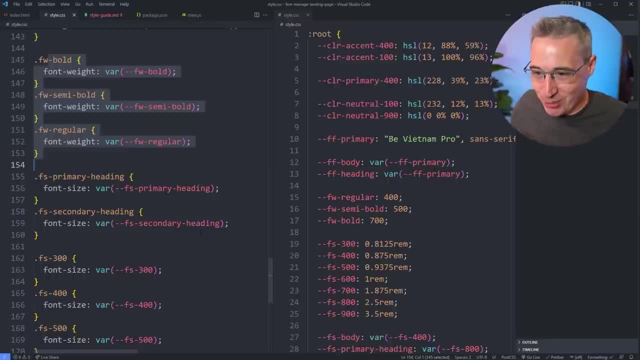 And that was also a really long part one. So, yeah, we're going to end this one here. I think it's a nice ending place And if you're watching these as they're coming out, the next part will be coming out in just a few days.